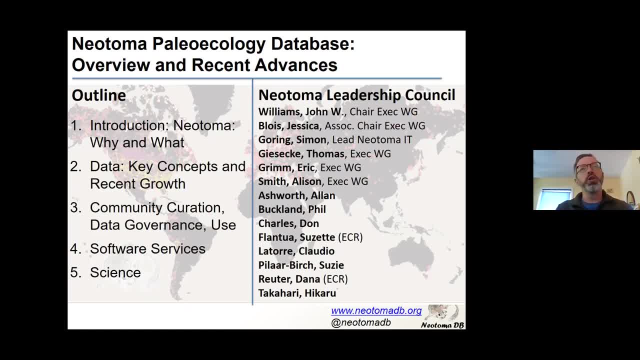 people here who also are active contributors to or users of Neotoma data. So for this talk I've designed it as kind of an overview, kind of walking through some of the main components of Neotoma, but I'll sprinkle in some updates and kind of latest changes along the way for people. 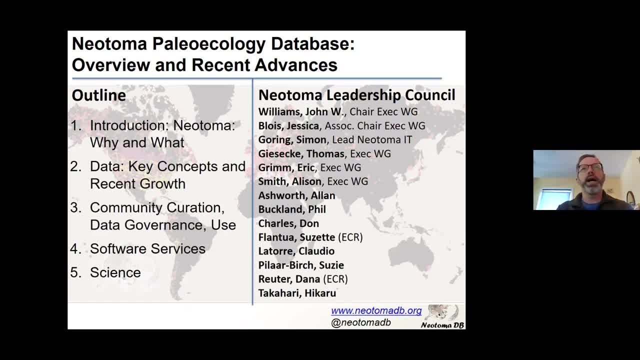 who are more familiar with Neotoma can see some of the current things that we're actively working on and are in progress. So I also want to acknowledge with this slide and the next one that, as Daryl said, lots of people are involved in Neotoma. 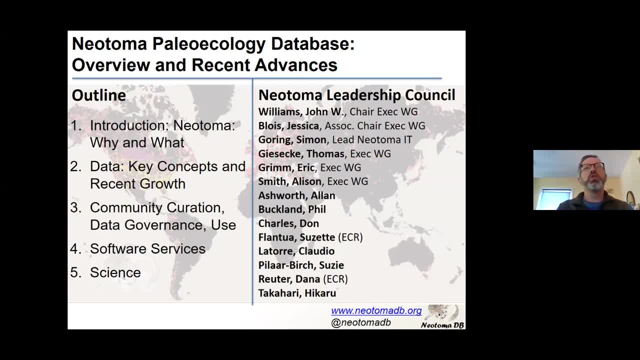 I serve as the chair of the executive working group, along with Jessica Blois, Thomas Giesecke, Eric Grimm and Allison Smith, And the executive working group is part of a larger body called the Leadership Council that sets the policy and sort of acts as the scientific 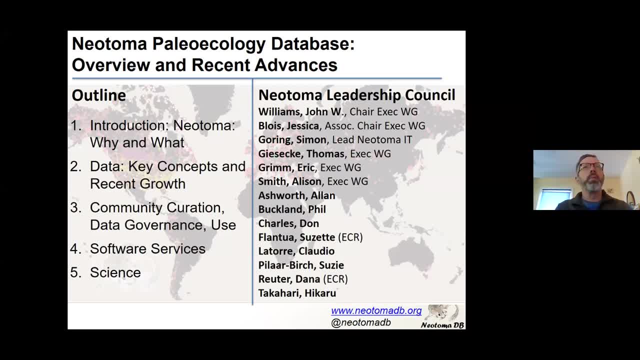 stewards of the database, So I'm representing lots of people here, All right, So I'll give an intro. I'll talk about some of the key concepts in the Neotoma data model and growth trends then, equally important, perhaps more important. 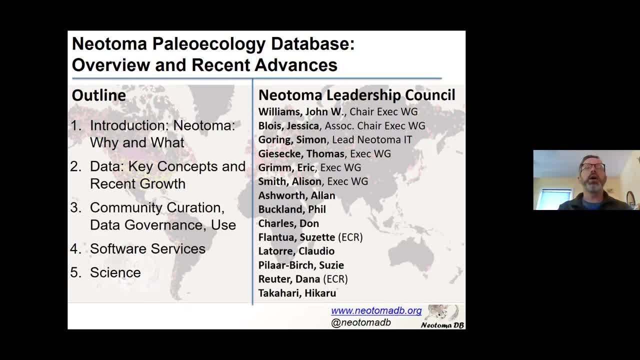 talking about some of our key concepts in community curation and how to govern a large international multiproxy data resource and policies of data use. then talk a bit about some of the services for software that are available, and then just a highlight or two of some of the science that's being powered by this kind of work. 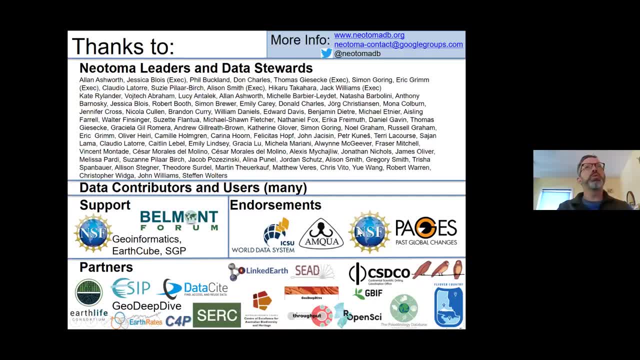 All right. So again really just want to say lots of people are contributing in lots of different ways. A really key concept is that we have people who are data stewards. These are people who are actively uploading data. They have expert knowledge in their domains. 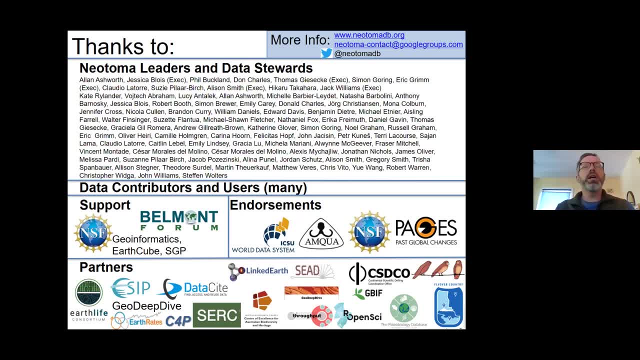 They come from fields of palynology, diatoms, ostracods, terrestrial vertebrates, geochemistry, lots of different people from lots of different parts of the world, putting data in, organized into these constituent databases that I'll talk more about. 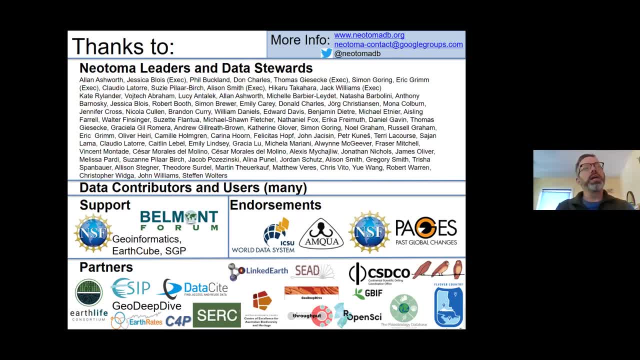 I also certainly want to acknowledge support. Most of our funding has come from the US National Science Foundation and the Geoinformatics, EarthCube and Sedimentary Geology and Paleobiology Program. We've also got some funding recently for a couple projects from the Belmont Forum. 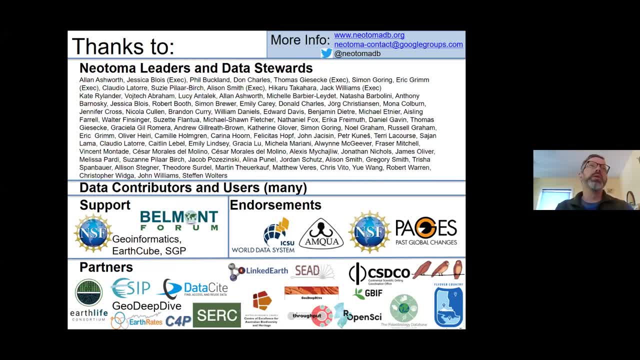 So really that's what makes a lot of this possible. And then a key goal for us has been kind of accreditation and recognition And so, as Darrell mentioned, being recognized and recognized, And so I think that's really important. 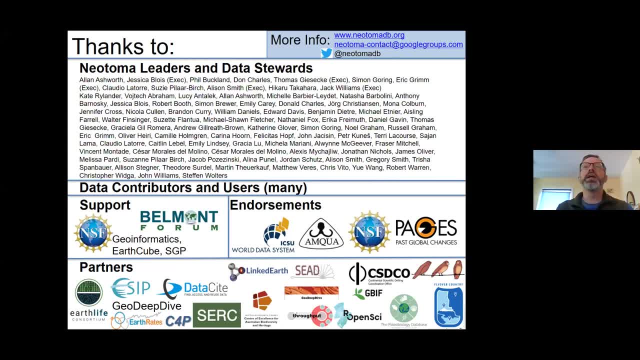 I think that being recognized by PAGES is really important to us as a trusted place to put data, along with NOAA, paleoclimatology and Pangea, as sort of three currently recommended PAGES data repositories. We're listed as an NSF-approved data repository. 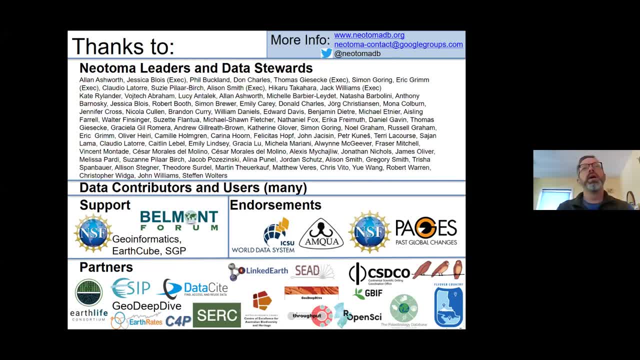 So if you have an NSF grant and want a place to put your data, Neotilda could be a home for it. And then the ICSU is a sort of international registry of trusted and approved world data systems. And then there's lots of different people we're partnering with. 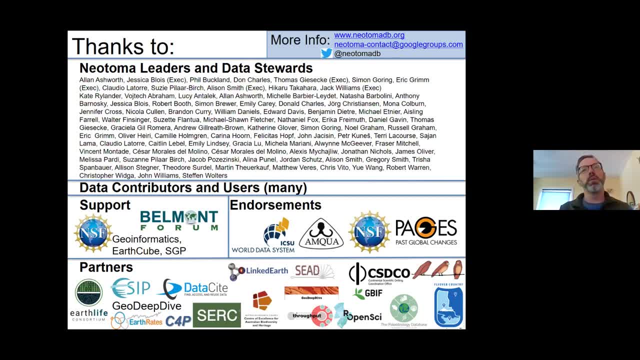 As we're all trying to build out this ecosystem of these data, resources and components. we kind of work with different people in different contexts And so just kind of showing some different partners down there And just to kind of start with the motivation. you know why do this. 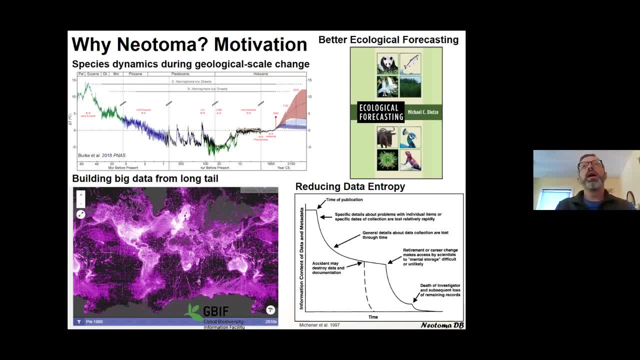 Why invest time and effort by any of us in this kind of effort? You know, for me, as Darrell mentioned, very strongly motivated by global change and the promise that paleo records have a really important part to bring to bear on global change. 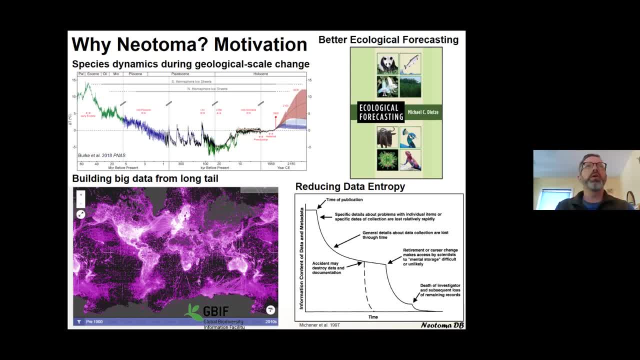 We're living through a period of geological scale climate change. Does it have geological precedent or not? Well, clearly we're going outside the historical record in terms of the range and scale of variability. So we want to look for analogs or at least model systems for what's happening today. 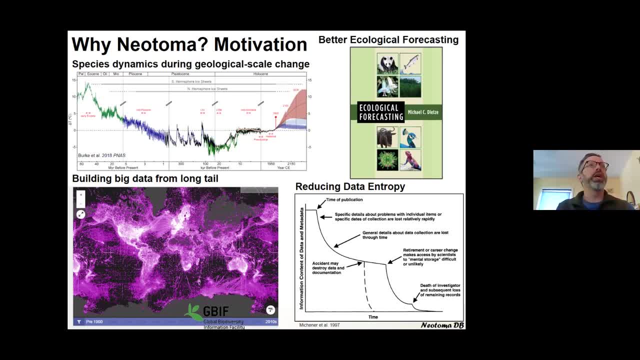 looking at things like past glacial interglacial cycles, or going as far back as the Pliocene say, or even the PETM, or finding for at least partial analogs in meaningful ways for the changes happening now, So bringing all that knowledge to bear. 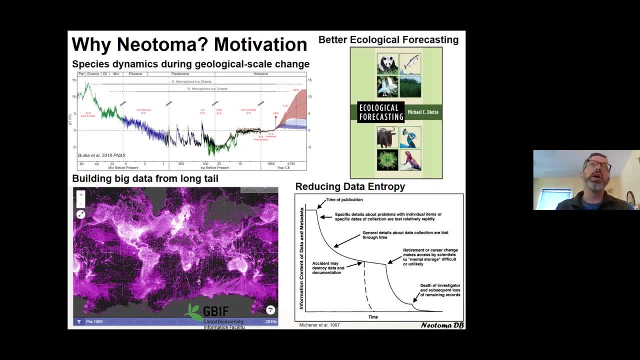 about how species have evolved or moved or responded to those climate changes of the past. Then lower left, you know GBIF as a group that's been very successful building up a global resource of all species occurrences or species occurrences worldwide. Every dot there represents a location where a scientist or there's been some observation of 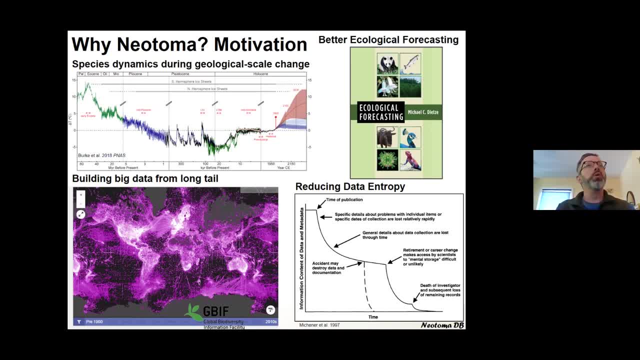 a species at a point really powering and enabling these global biodiversity studies and wanting to achieve that kind of coverage and capability. So we're going to look at that And then we're going to look at the data that we have, for all the many, many records we have going. 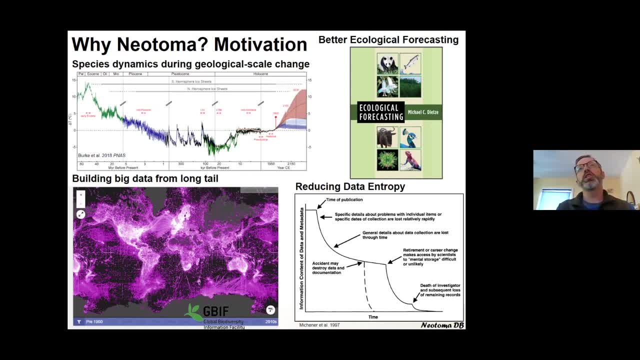 back in time through the past. Using that information to power our better ecological forecast right. Using this data to make our models better, improving our ability to predict where the world will be over the coming years to decades, given different scenarios of, say, climate change. 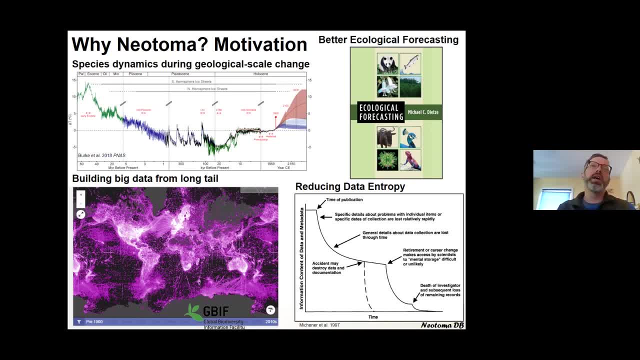 And then this last challenge of archival that you know. we all know that data is lost over time, that we write our paper, We move on to the next project, We lose the notebook, The server crashes, There's all kinds of ways that data gets lost. 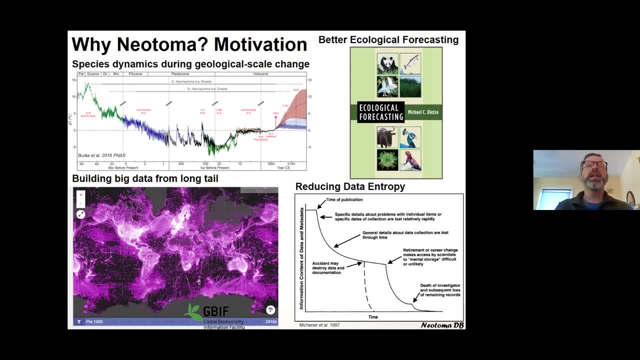 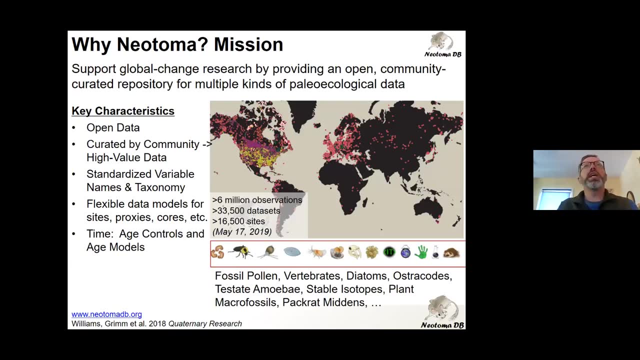 And all that hard-won effort in getting that data and finding it goes to waste, And so efforts like NIATOMA also have this very important archival mission in addition to their- maybe you know their- equally important science mission. So NIATOMA, then, its mission is to support global change research by providing an open 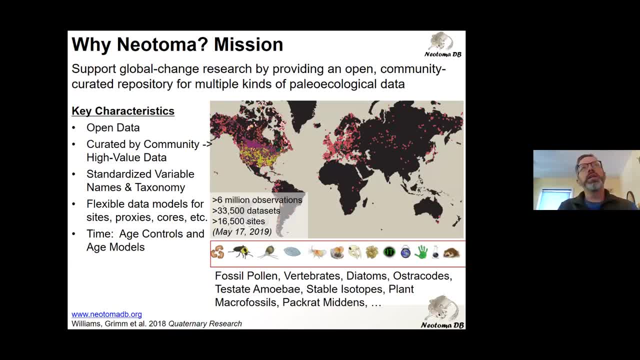 anyone-can-use-it- high-quality, community-curated data resource for different kinds of paleoecological data. We, you know, adding value by doing such things as making sure that our variable names are standardized. We have a defined dictionary of variable names. 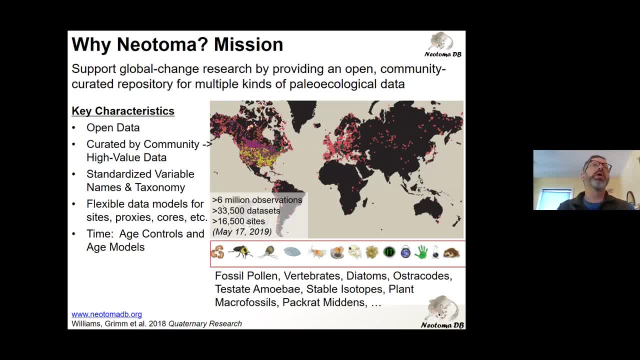 So if somebody misspells a taxon name somewhere, that doesn't we clean that as we go. We correct kind of common errors like that that can really hinder larger scale data syntheses. We have our data model able to handle, you know, multiple cores from a site, multiple. 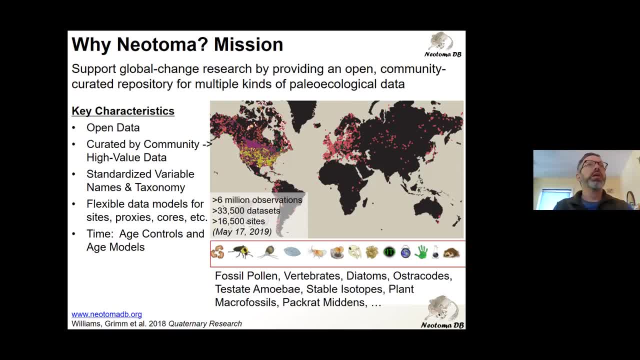 samples from a core. It's a very flexible data approach. And then ways of- I'll talk more a little bit about, you know, flexible ways of handling time through our storage of the radiocarbon dates or other age controls, and then the inferred 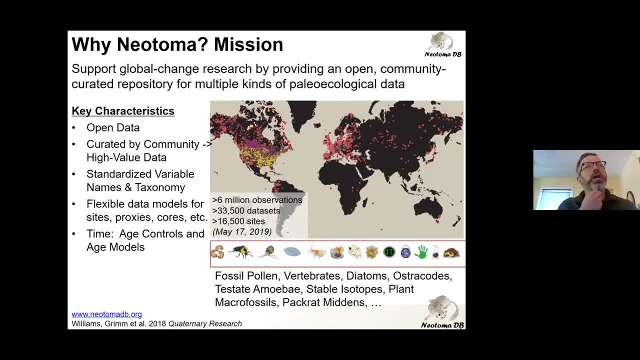 age of models, Those numbers, they're actually a little out of date. I must not have updated that particular part of the slide, But you know we have now over 70 million observations. you know worldwide Over 30,. you know, I think, over 37,000 data sets and 17,000 sites. now. 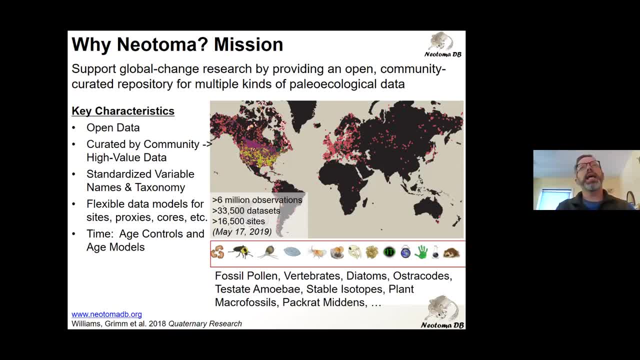 So you know again. one of those challenges in the big data era is like how do you manage? you know how do you manage all this data And you know this is large, from a sense in the perspective of being an individual. 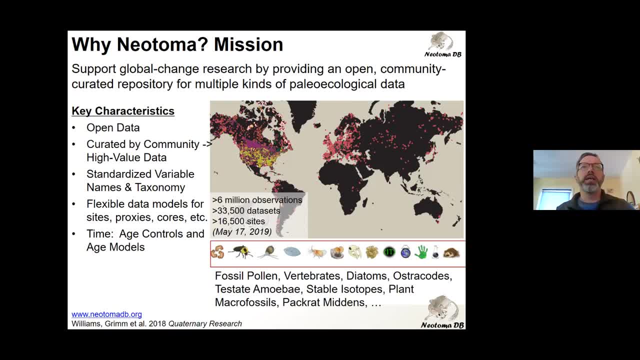 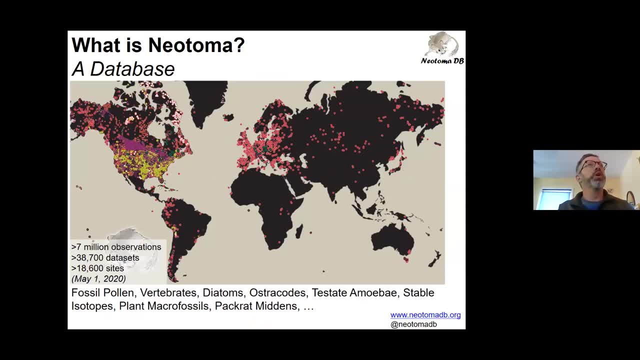 scientist trying to compile data together and really making it possible to bring all this data and knowledge to there. Okay, Right, So then. yeah, so, moving then to: you know what is Neotoma? Now we've kind of talked about the why. why have Neotoma? 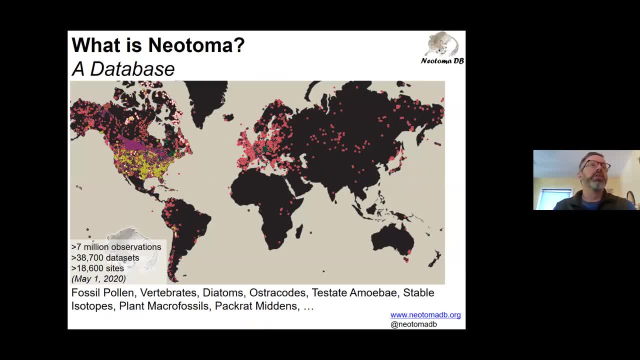 So it is a couple of different things at once. It is a database and there, in fact, are the updated numbers, there in lower left, From May of this year. This year It's a database, right, So it contains, you know, species occurrences or abundances for different tax, at different 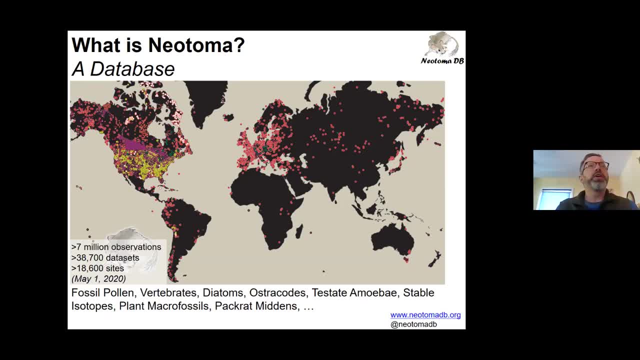 places It can. it includes your radiocarbonates and other age controls. It stores increasingly different kinds of geochemical information, like stable isotopes in different places. So that's one thing that the Neotoma is. That's often the first thing that people think of when they think about what is Neotoma. 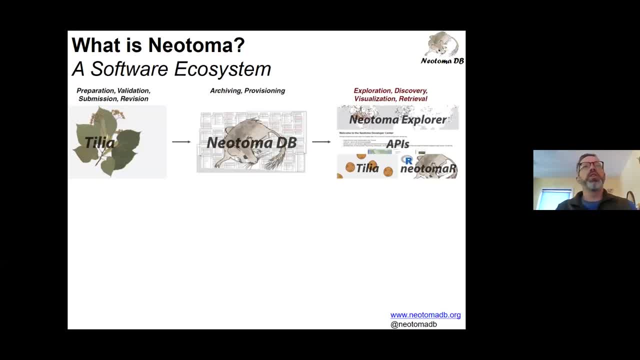 But it's also a set of software that goes with that database. right, You know it's. it's. there is the Back end relational database and all this is stored in, but then there's also a series of of software packages and resources that go with it. 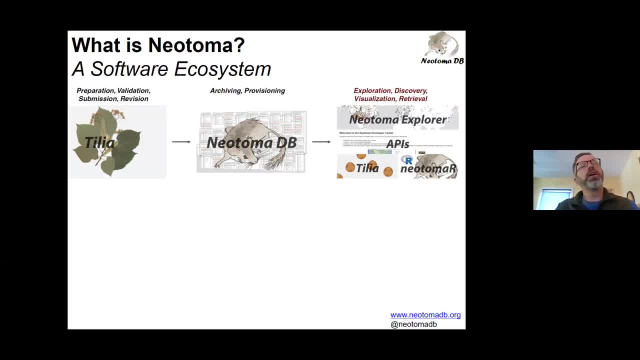 We have Telia that Eric Grimm is the lead developer of, and that is both. That's what we both use to upload sites into Neotoma and make sure that all the data cleaning is done. So it's a primary tool used by the data stewards cleaning and preparing data for upload to. 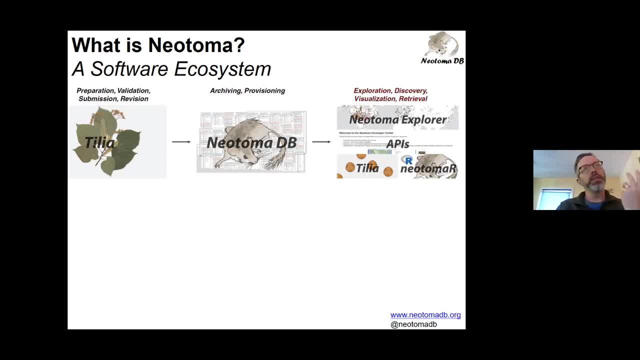 Neotoma. You can also download data from Neotoma back to Telia, So it's also a good place to look closely at it, Individual sites and what they hold. And then there's other tools as well. There's Neotoma Explorer, which is usually the first point of contact that many people 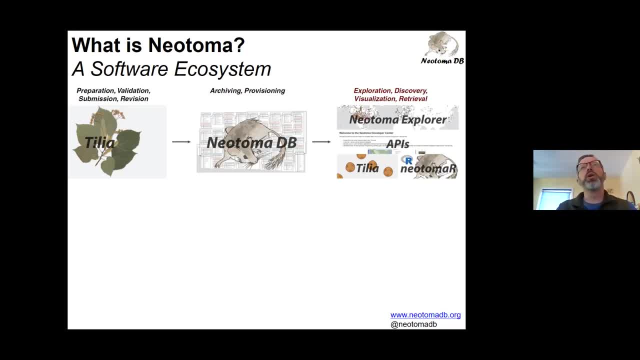 use when they're first learning about Neotoma, a map-based interface for exploring and looking at Neotoma data. We have the APIs, the programmatic interfaces for extracting data from Neotoma, And then we have the Neotoma R package that sits on top of that. 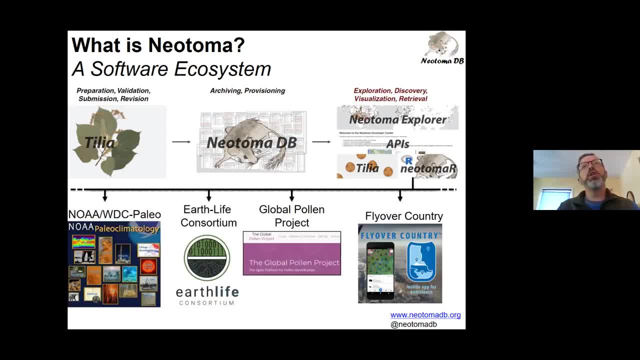 I'll talk about these a little bit more later on, But then you know, sitting on top of that, you know those. this top tier is the stuff that we have supported and developed within the Neotoma team, But then by making the APIs kind of open source and available- the R package open source- and 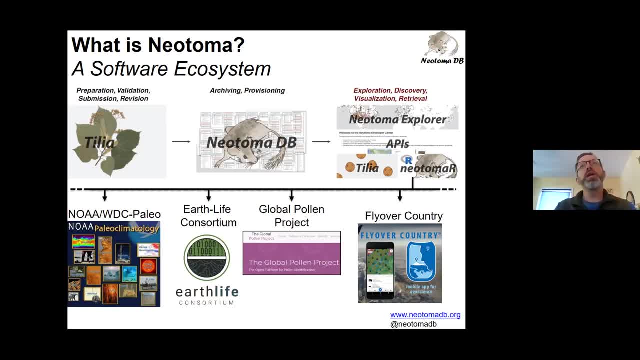 available. then other people started to build on these tools and started to build their own capabilities. So NOAA paleoclimatology is you can. you can search there through their paleoclimatic data portals and retrieve Neotoma pollen data currently. 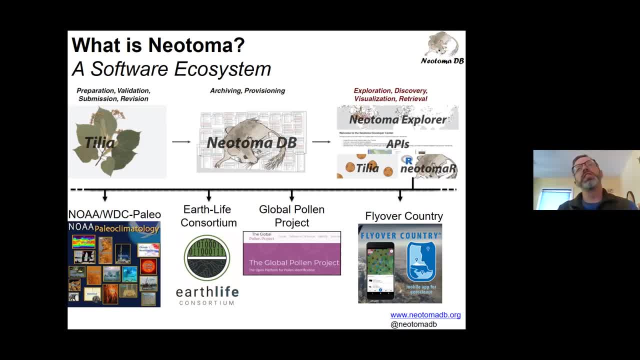 And we're working with them right now to extend their data retrieval services to other kinds of Neotoma data. The Earth Life Consortium. Earth Life Consortium is a resource for looking and searching across different paleobiological data resources, And it has some tools that you can search in Neotoma, the paleobiology database, and 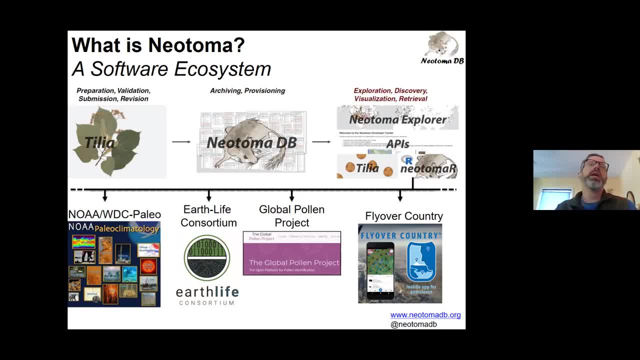 other data resources: The Global Pollen Project, which is a kind of a library of pollen images helping people identify their pollen types, And that that will query the Neotoma to look at maps of where different pollen types are found. And then Flyover Country as as a third party app that mostly based in the US but not 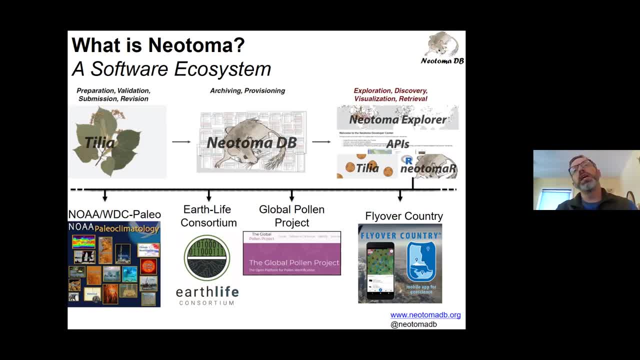 exclusively, Whereas you, as you travel from place to place, you can get information about the kinds of rocks you're flying over, that where where the mammoths or dinosaurs have been found, and other things like that. That's also drawing upon Neotoma resources. 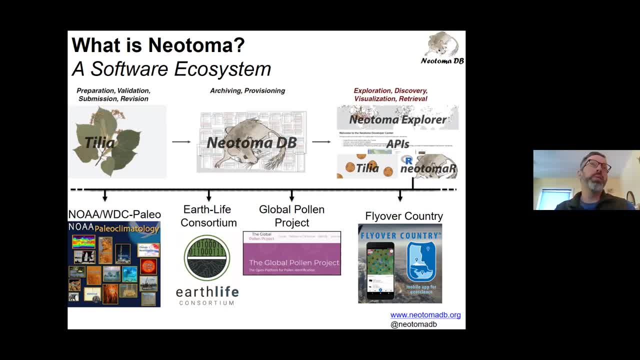 So to me, one of the important points here is that once you make data open, all kinds of wonderful things happen and all kinds of other things start to get leveraged- things that you yourself could never do- And so creating these open data resources really powers a whole new layer and possibilities. 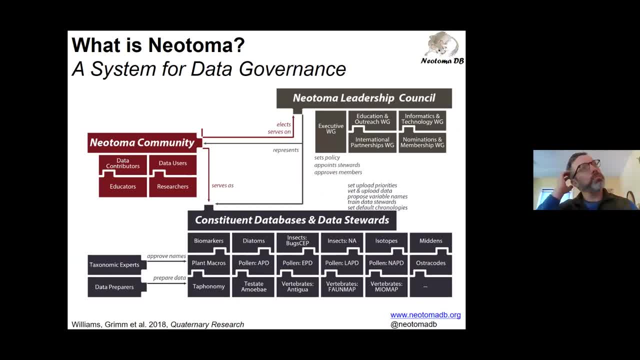 for innovation And it's a system for data governance that, when you are working with different kinds of data from different regions with- and nobody has all expertise. You know, I have my area of expertise in pollen, but I don't know anything about vertebrates. 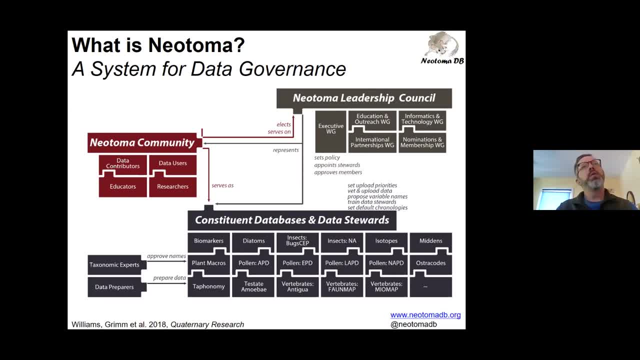 and everybody's got their own domain. We need some kind of system that both centralizes the data management, the backend infrastructure, the software, but then distributes the governance. So you need ways for different people to be able to have ownership of different parts. 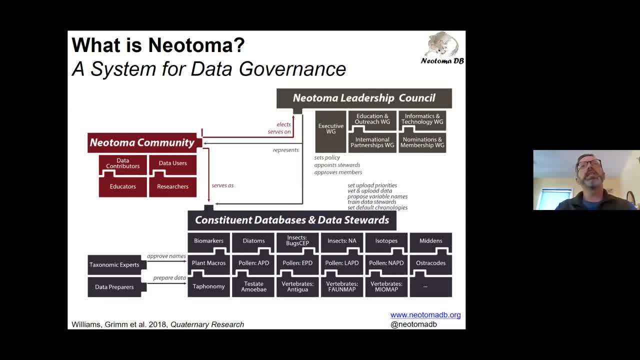 And for me that's what I'm looking for. And so the way we have kind of organized this conceptually is that we have the leadership council that I mentioned that acts as sort of a steering and coordinating committee for the entire group, But then a very key component of that is down at bottom there, that the constituent databases. 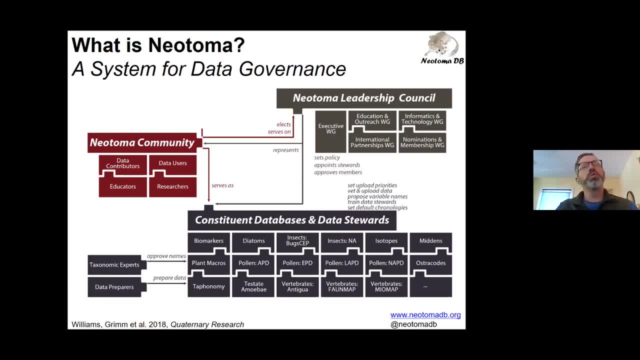 and data stewards, where different groups are in charge with different parts of the data. So, for example, there's the European pollen database and the Latin American pollen database, There's the vertebrate database for North America and there's a test data media database. 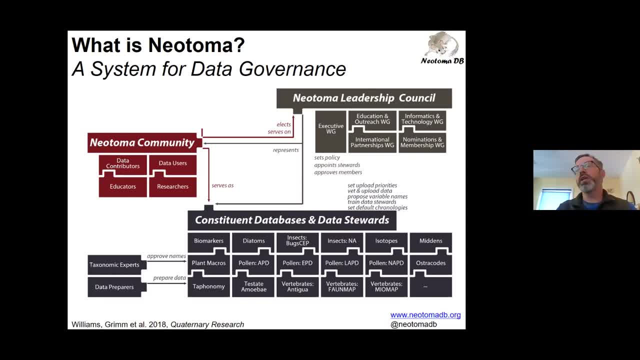 So the idea being that different portions of the data stored in the Atoma are curated by different communities and those communities and those stewards can both upload data, they can correct errors, they can update data, So they have the editing privileges, but only for their data domain within the Atoma. 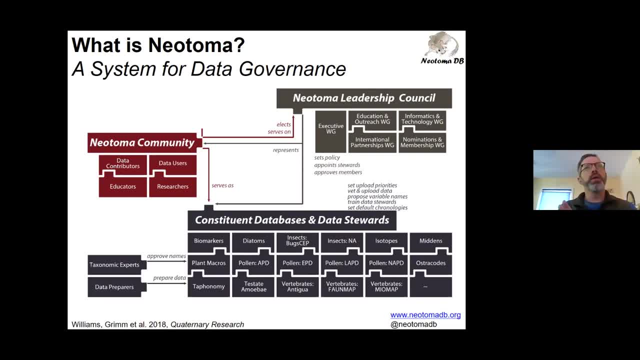 So I can't go in and edit the vertebrate data because I don't know anything about it. It wouldn't be wise for me to do that. But I do have editing privileges as a steward for the North American pollen data, So that's kind of my domain of expertise. 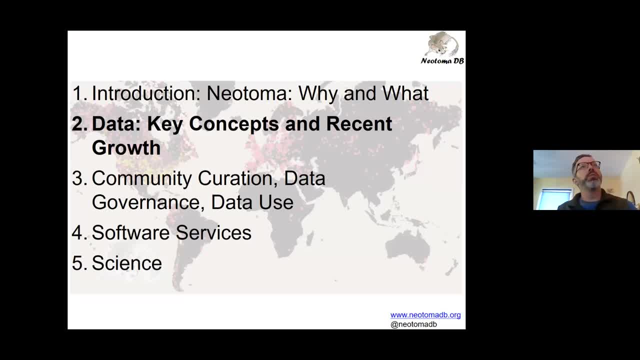 Okay, so that's. we'll come back to that a little bit too. So this is just some of the overviews, But it's really important to kind of land that point that it's a database and it's a software ecosystem and it's a community governance structure. 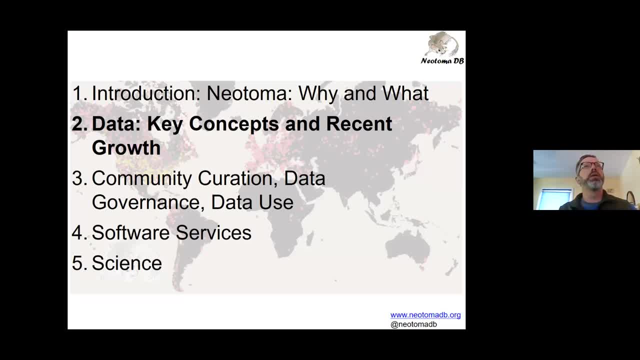 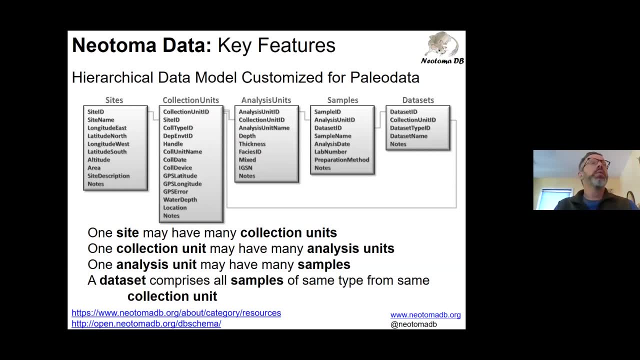 They're all kind of co-bound together. All right, So some concepts that we don't. you know we could spend more time in any of these, but it's just to kind of understand some of the features of the data If you kind of dive into the relational database model that's sitting behind. 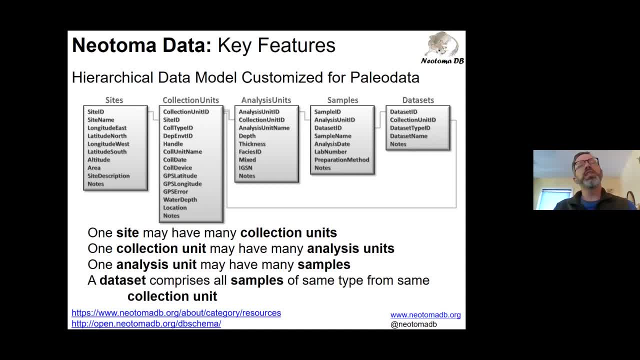 all this. it's got a couple different things- ways that things are organized- And one- and this is all designed by Eric. Eric has both designed the Neotoma data model and the Tilea software. One thing it's got is a very important concept. 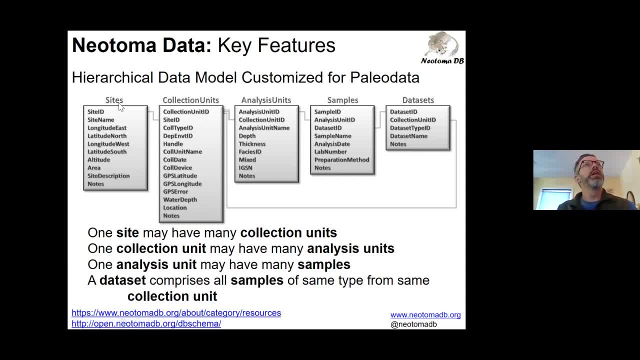 This is hierarchy, where you go from sites to collection units within sites, to analysis units within a collection unit and then samples within those analysis units, And so a site would be like a lake or a cave or an archaeological site. Those would become a geographic entity. 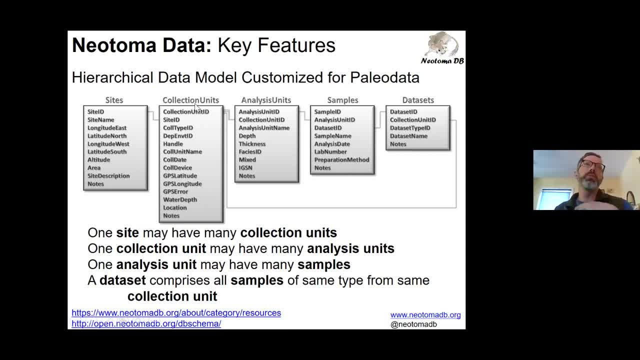 The collection units would then be the cores or the pits or the bone piles or other spatially discrete locations within your site that you're going to take some data from, And then the analysis units and the samples are basically, you know the vertical horizon to where you go. you know, layer by layer, 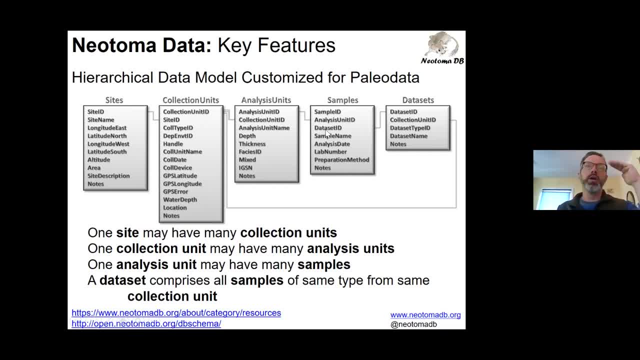 level by level, and take a series of measurements from your sample, your core or your cross section, road cut or what have you, And then the data set. A data set in Neotoma terminology are all samples of a given same type from a collection unit. 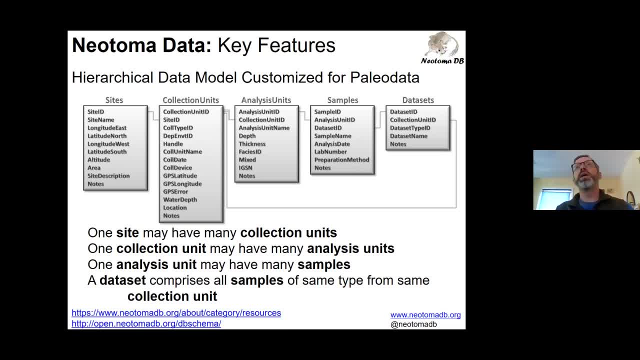 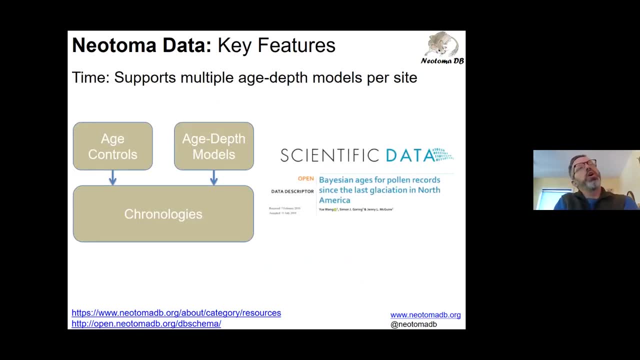 So all the pollen samples from a single core would be a data set. All the diatoms from that same core would be a different data set. So that's how we define and bound data sets. So that's a quick overview there, And then another quick overview is just to talk about time. 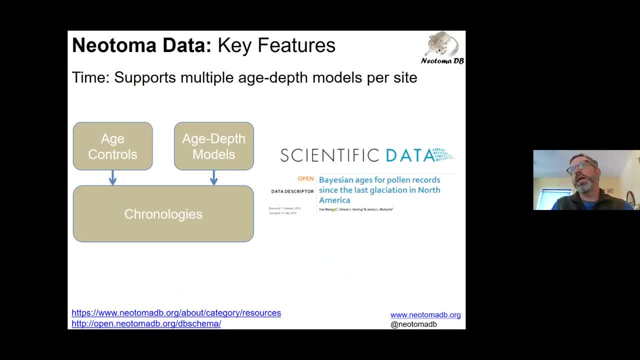 So we have, you know, in our structure, the radiocarbon dates, the lead 210 dates, the other age controls are the raw data that usually will not change that much after the first measurement and reporting, And so those are stored in one table, the geochronology table. 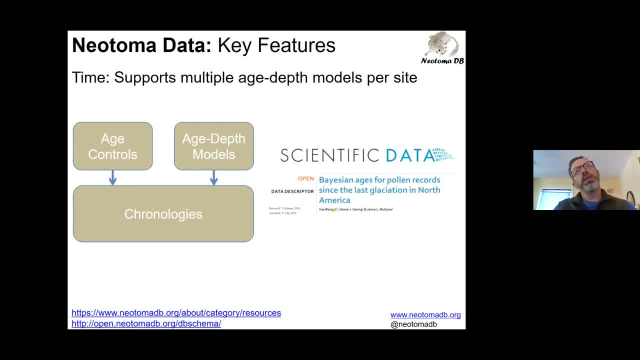 that's pretty stable and does not change that much. But then you know, age depth models change all the time. We get new statistical packages like Bacon or B-Cron. We now have INTCAL 20.. So we need to go back and revise all of our calibrations that used to use INTCAL 13.. 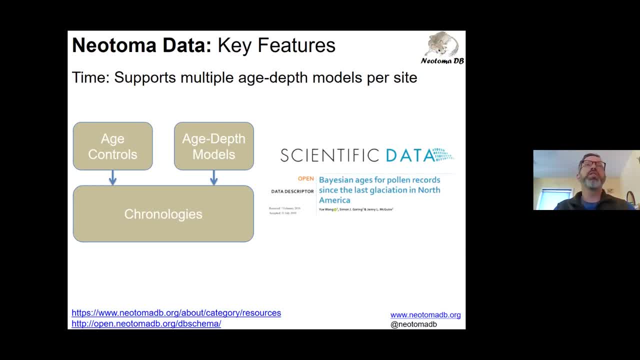 So the age depth models get revised regularly. So we have another set of tables that store those metadata about those models And then the chronologies are essentially the combination of those two And then the age inferences that come out of that So we can store for a given depth in a given core or collection unit. 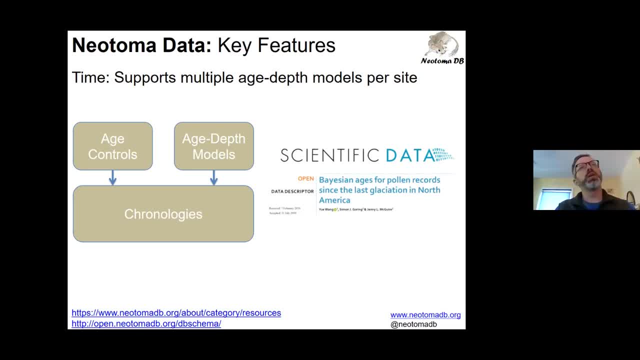 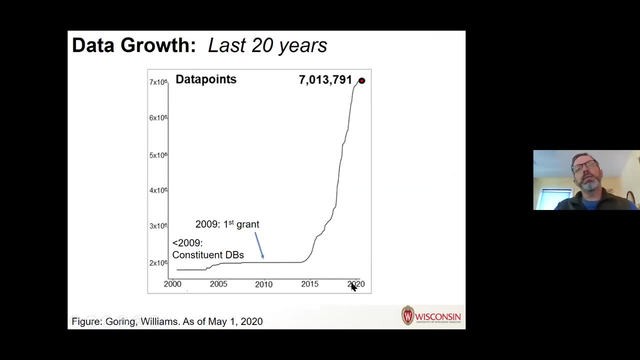 multiple age inferences based upon the different age depth models that have been run over the years. Well, you can have a preferred or kind of, you know, maybe the default one if you were just kind of going in and pick one quickly. So that's a few key concepts about the data model. 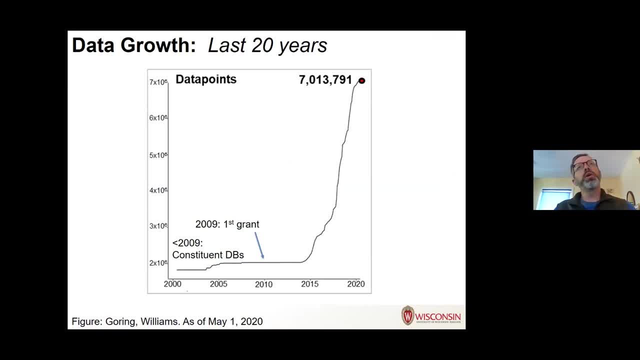 And then, you know, a key point is about data growth. You know, one of the real values of having this community-curated approach is that almost always there are these key bottlenecks with building these large databases, which is it is labor intensive. 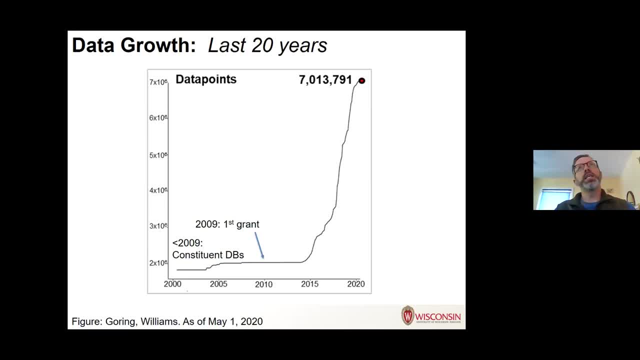 And one thing we want to do is make it less labor intensive to add data into it. So let's start with the data. So here are the two caps on the right hand side. So in this case, in this case, if I have a bunch of different data, 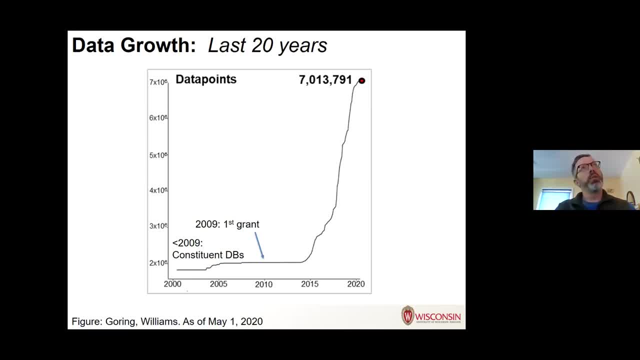 then the data, that the data is being issued, is going to be distributed. So that means the process of uploading data, cleaning data, standardizing data. that takes expert judgment and some time, And so by distributing this expertise and workload among a broader community of stewards- 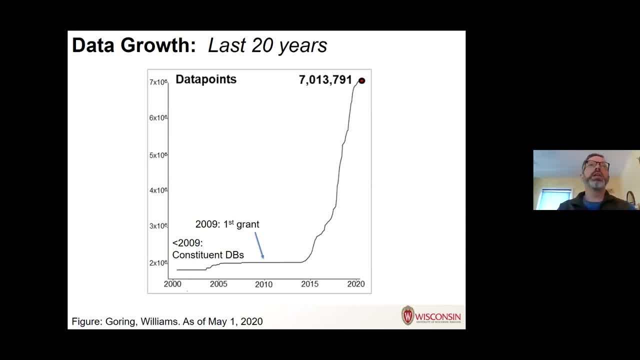 we can then increase the rates of data upload. first grant that got it started was in 2009, and before that there was individual separate databases like the global pollen database or the or fawn map or these kind of discrete continent scale or taxa scale databases. they existed, they pre-existed, but now there's been. 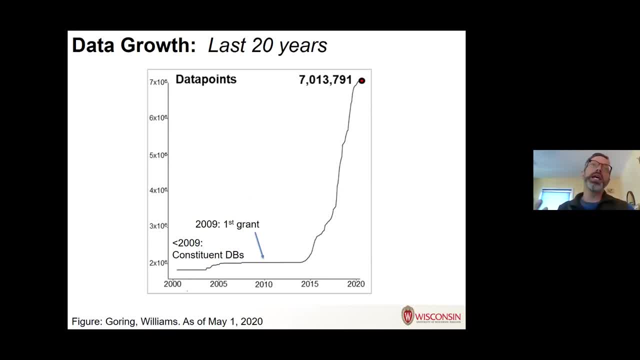 this effort to coalesce them into neotoma and then start to add new data to neotoma. and then you can see that real inflection point about 2014 and that's when eric released tilia with this new functionality for data stewards to upload data to neotoma to make corrections and 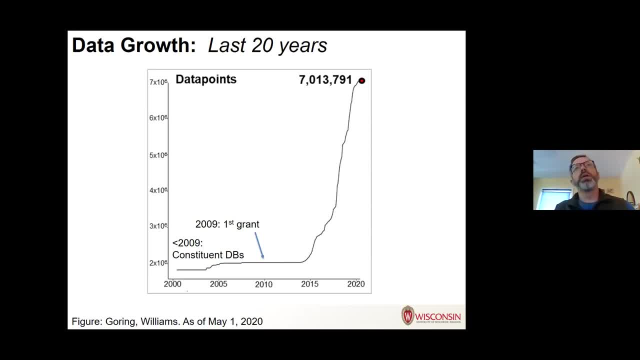 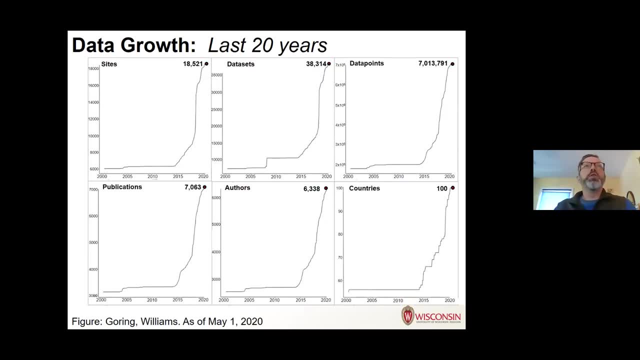 so forth, and that's why we've had this very rapid growth ever since then. so, as of you know- uh, last you know, last may- we're over seven million data points and you can measure data growth and data volume in different ways. so you can see number of sites, you can see number of data sets, um 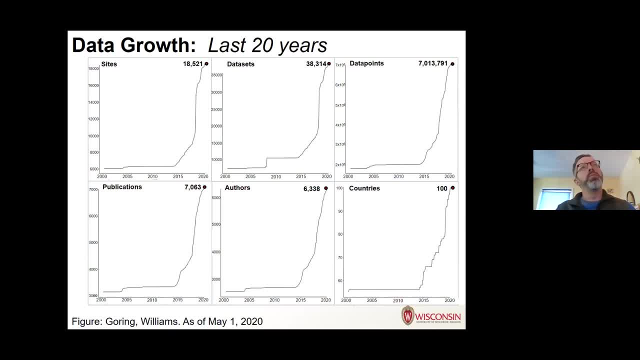 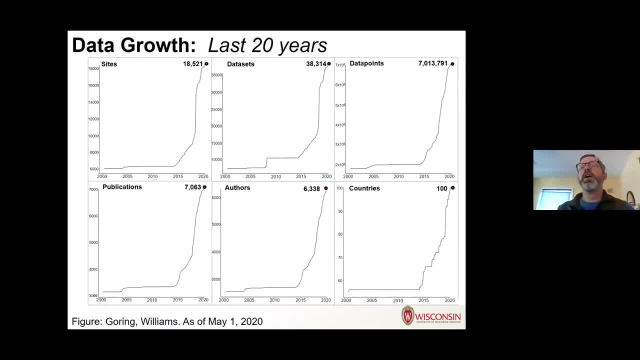 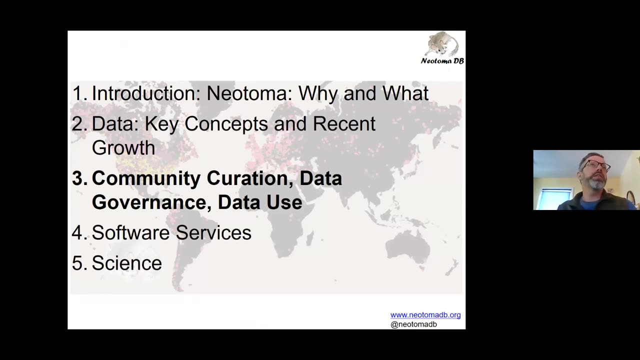 metadata about the publications and authors and so forth. you can see that lower right one. now we now have a hundred countries now represented in the account. we've hit 100 country mark, okay, so that's kind of a summary, some of the key data, concepts and growth. then to talk about this, 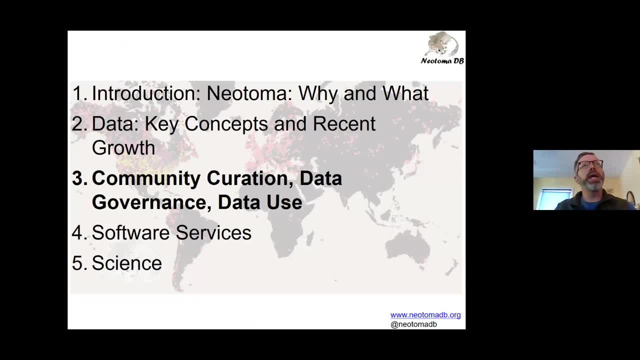 key, i think, for this community. it's really important for people who are involved in pages to think about. how do you just as the pages, how do you have an international coordinating body? given many different kinds of research in many different countries and people are involved for neotoma, how do you build a community, international, multi-proxy? 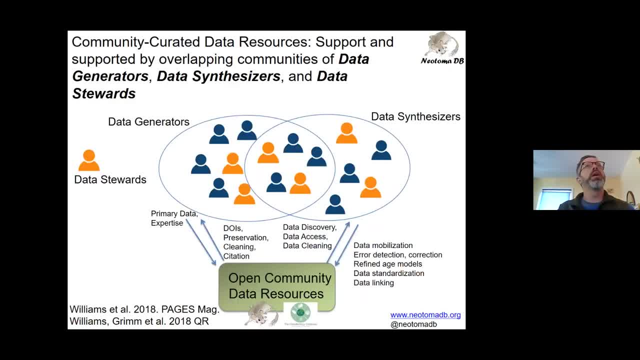 data resources. so here's some of the key elements of that. so one key concept and this was- this is a figure that was from a special issues of pages magazine from 2018 that daryl and i co-led with a couple of others- um, that really, you know, really talked about this concept of data stewardship and 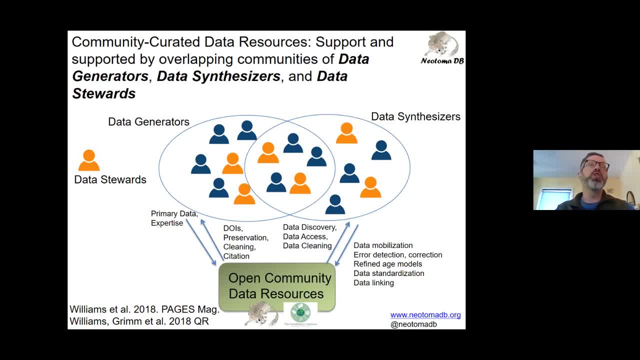 thinking about open community resources and both the services provided to the community and the services received from the community, this very important symbiotic relationship, and then further separating or kind of thinking about in the community how there is at least three roles. there are the people who generate data. they go out and take new cores, they work in the lab and 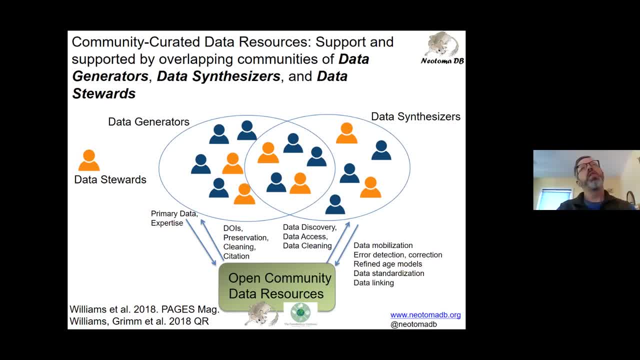 generate new measurements, the data generators. there are the people who are the data synthesizers. they are gathering lots of observations together, they're cleaning, they're standardizing, they're updating age models. they do that work. and then there are people who are the data stewards, who 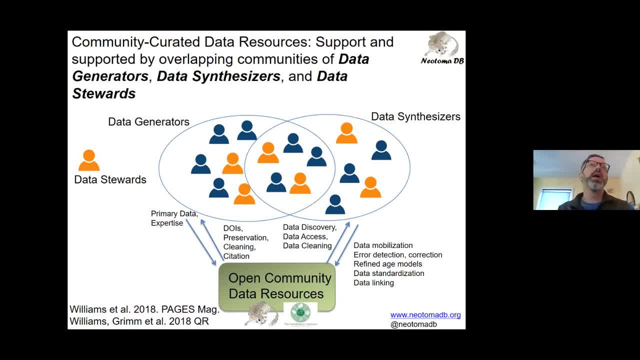 are kind of working as a point of interface between the two and the databases- and you can see how the diagram is drawn here- is that these are three overlapping communities. most of us, especially in this day and age, can move among these different roles. there are some times where my lab we're up generating new data. there's other times in my lab. 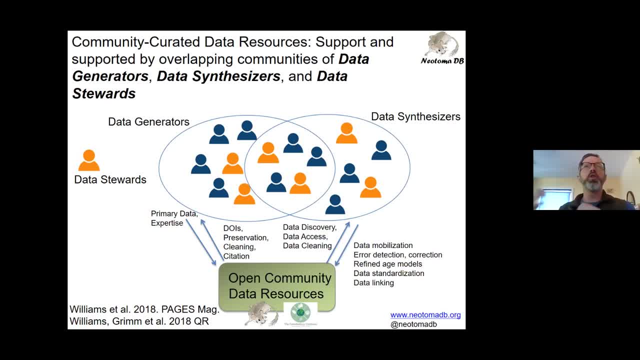 we're trying to like look at our, our data in contacts with other records that other people collected. so you can. these are not distinct communities, these are overlapping communities here and then thinking about the services received and provided. you know data generators: they add data and they're generating data. the data generators: they add data, they're generating data. 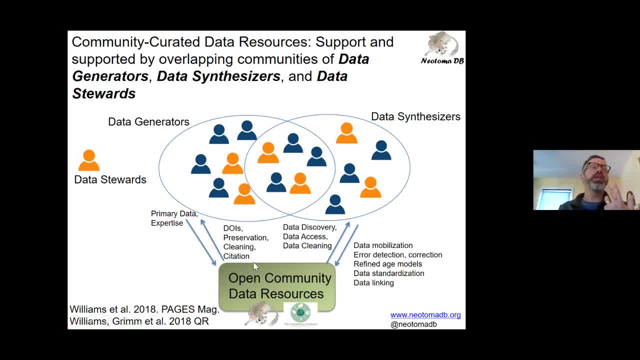 um. the other thing that we're doing- an interesting study that i've been doing in the other subscribe um, the other big one- is able to do here, um is that we're looking at which data generators and why that is the data generators, their data to neotoma or other open community data resources. you can see i've got an icon for 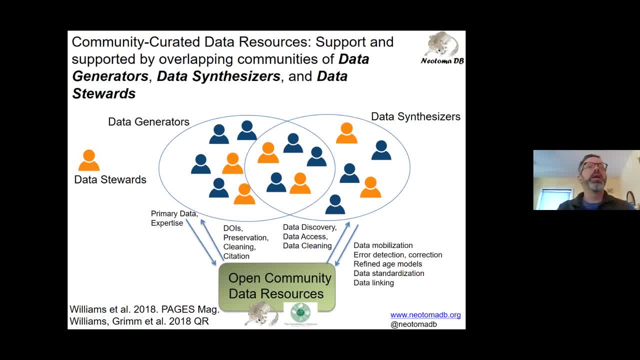 the paleobiology database, which is kind of very similarly structured. um, they add their data to neotoma and then they receive services of doi's being assigned to their data. they have some confidence the data will be preserved. over time there's been some cleaning and standardization. 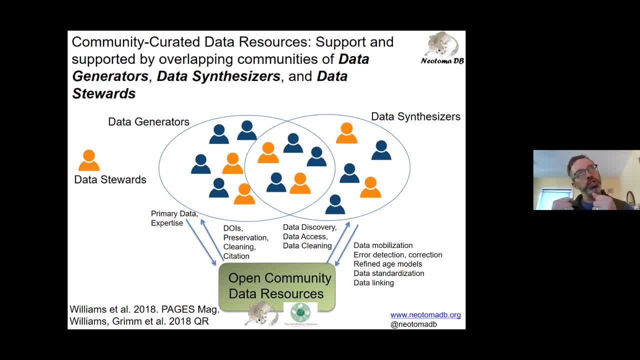 so their data is more kind of able to be kind of connect, collect, use in association with other data and, you know, enhance citation rates. there's definitely good evidence that when you put your data to open resources like that, you get cited more, so there's a sort of citation benefit. 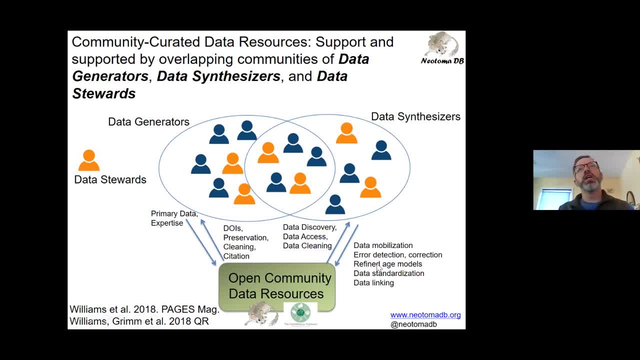 that goes with that. um data synthesizers: they help by helping get new data added to neotoma. they can often detect errors that were missed during time of upload. they can update or refine age models. they can contribute to data standardization efforts. they can start to link. 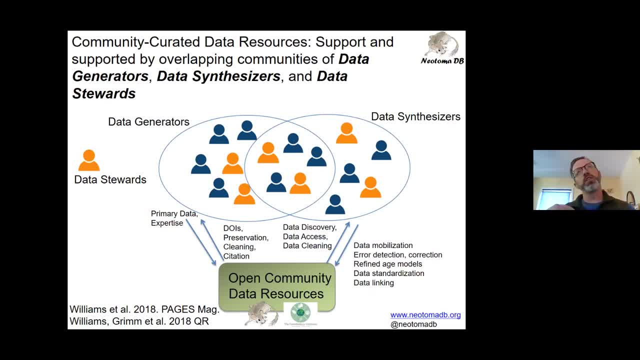 neotoma to other data resources that are out there. so there's another set of services that the data service synthesizers can provide and then, in return, neotoma makes it easier for them to find data, to get the data, to get some data that already has some pre-cleaning done for it. 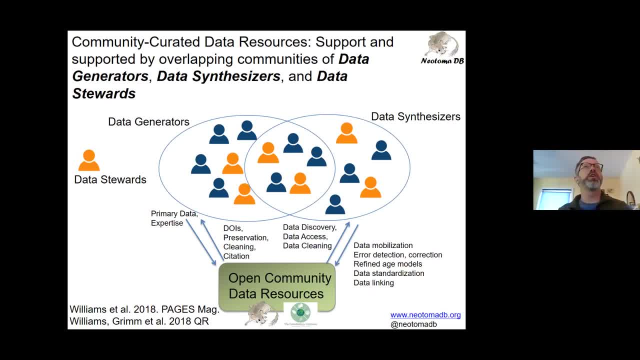 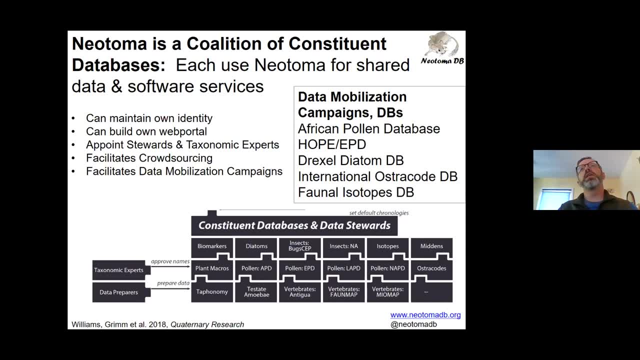 so this is important two-way symbiosis in all these different directions, and so a very, very, very important concept in neotoma is a concept of constituent databases, and this is i just want to, you know, emphasize this as much as possible, because neotoma did not appear. 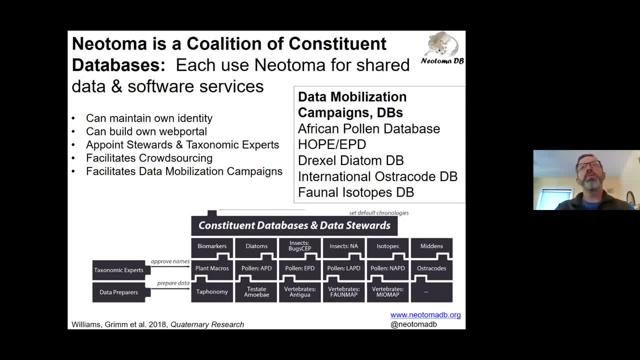 to be a binary type of data collected by the data services. so a lot of the data that we collect in the data systems are actually from the data services that we collect in the data services. so there's been a profound change in neotoma in the past and i think there's been a lot of. 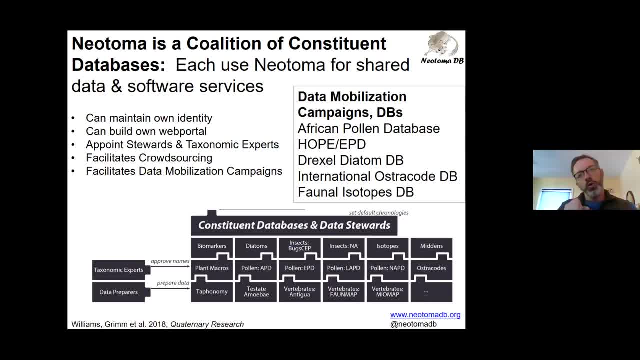 improvement in that as well, in the data that we have on the internet, because neotoma now has a really large database of databases and we can trace it back to the mid-1990s. again, we can trace it back to the early 1990s. so if you have a database of databases that is biologically. 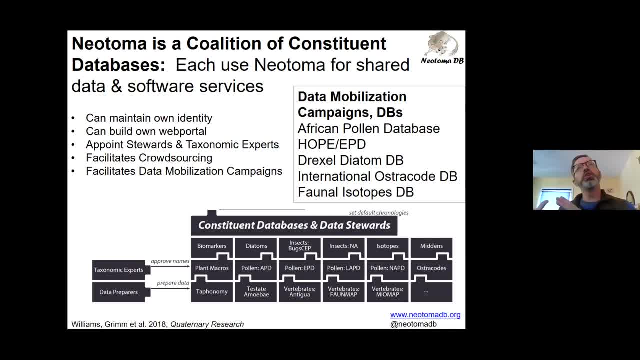 or biologically external, or biologically workable in the data research community, then you know the this process that builds upon these prior efforts, And so a key challenge, then, and a key need, is to make sure that these individual groups are recognized for their effort, right, Because? 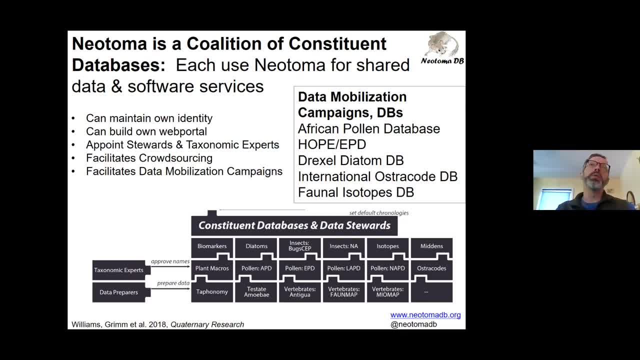 the Neotoma database makes it possible for people to find data in the European pollen database. but the European pollen database is its own distinct entity with its own distinct set of stewards that are doing the work and gathering the data and approving the data, And so EPD needs to. 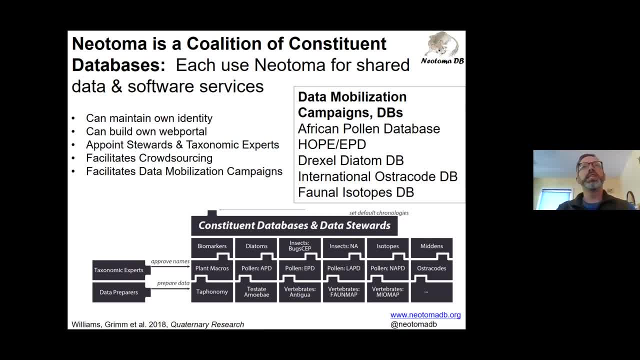 be recognized and supported as much as, say, Neotoma needs to be recognized and supported. So then this could be, and there's no inherent limit to number of constituent databases. So there's other people out there who think about well for my region, for my tax element group. 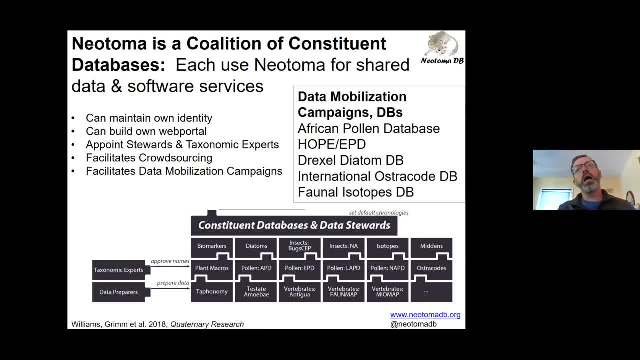 I don't have a place to put my data. One solution, one option is to create a constituent database. join Neotoma, get people trained as data stewards and start to upload data to Neotoma. Then that becomes a way you can. 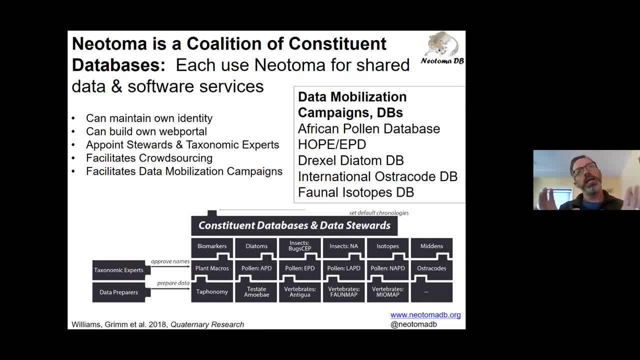 Power, your own kind of regional scale or larger scale data synthesis using the Neotoma support and services, And within that, any number of things could happen. You could have your own logo, you could have your own web portal in which you could- and we're currently, for example, 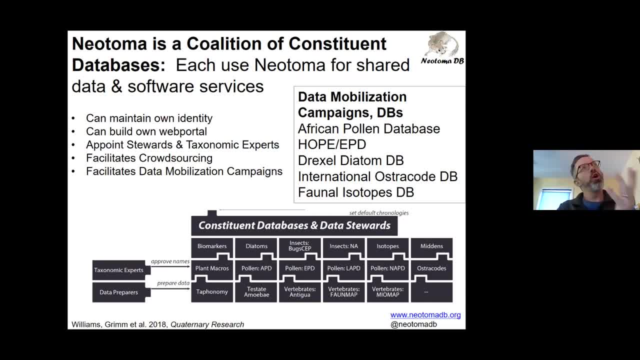 working with colleagues in Australia for the CABA initiative, where they'll be putting pollen data into Neotoma, but they're going to build their own front end web portal. That's a CABA portal for the data of Australia that will draw upon Neotoma. 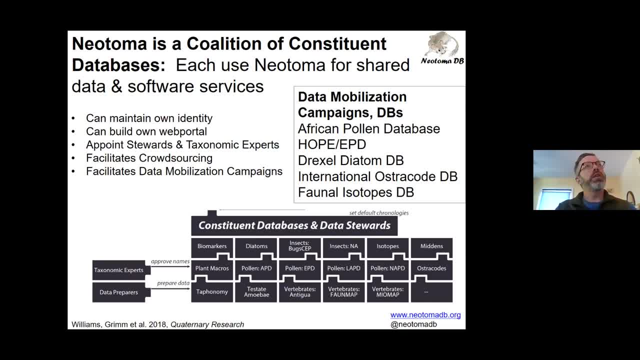 So that's one of the things that we're trying to do. If you're not able to build a local resource, you can build a local resource, So all such things are possible. They, the constitution databases- are in charge of appointing their own stewards and tax. 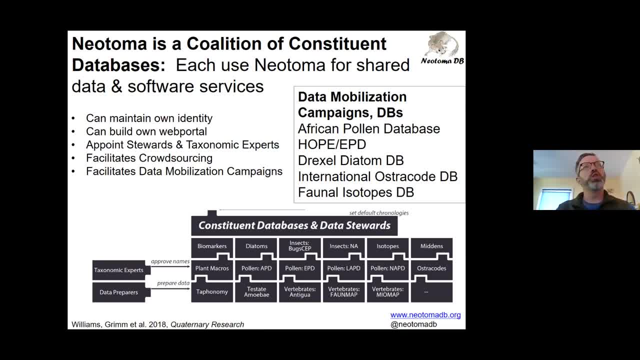 dynamic experts. They decide who who is in charge of these sorts of decisions, And then it facilitates these sort of crowdsourcing efforts and data mobilization campaigns. So, for example, right now supported by the Belmont forum and led by Nick McKay, Ann Marie Lazine, Sarah Ivory and 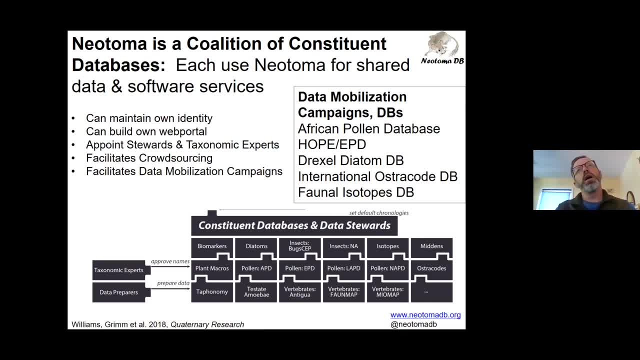 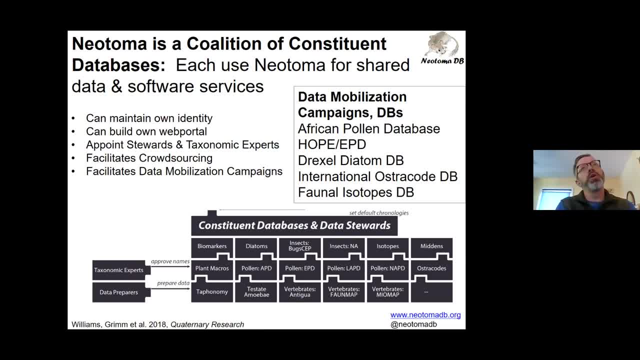 doing an effort to add records that are known to be out there and add them to Neotoma and then make them available to the community through Neotoma and through other portals as well. There's a hope project in Bergen that's doing a lot of work with the European pollen database. I should also say the Latin American pollen database. So it becomes this way: You can have this nice synergy between a research initiative in an area, adding data in Neotoma and then pulling data out to do whatever the questions that they want to pursue. 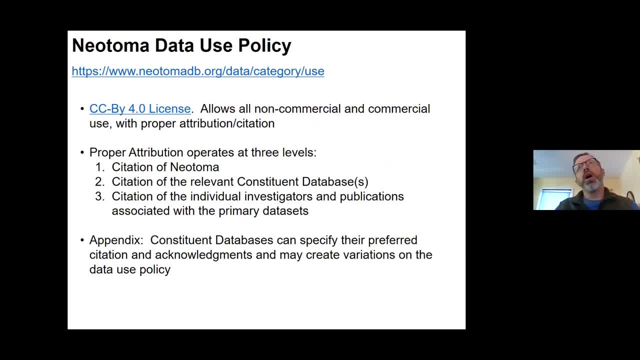 Our data use policy is a is a Creative Commons 4.0 license in which any use is allowed, as long as you properly attribute and cite Neotoma data, And we recently revised our data use policy earlier this year to clarify what proper attribution means. 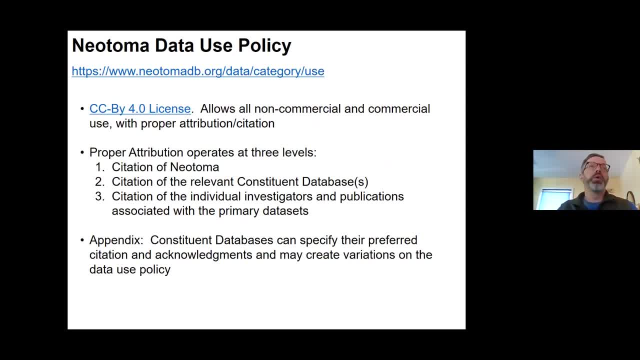 There's really three levels of citation that we'd like to see happen. We'd like to see, you know, Neotoma itself, of course, cited. We'd like to see the Neotoma itself, of course, cited. We'd like to see, you know, Neotoma itself, of course, cited. 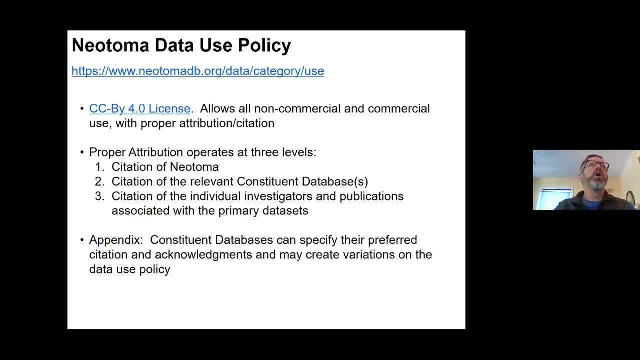 We'd like to see the Neotoma itself, of course, cited, and the data use policy explains that more clearly. about how to do that. we'd also like the constituent databases to be cited. so if you're really doing a project, say in latin america, you're. 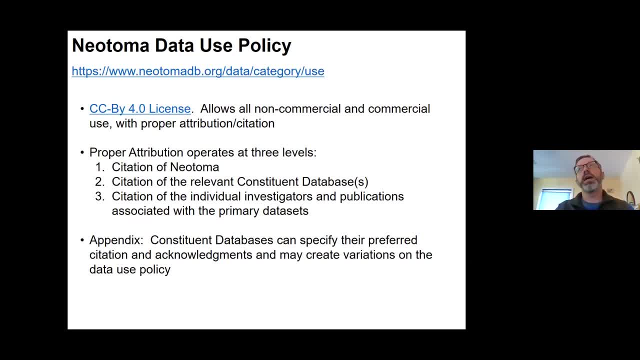 heavily drawing on the latin american pollen database. we'd like you to cite the latin american pollen database and mention it specifically, um, and then we'd like you to cite all the individual records associated with all the individual data sets, and so that, of course, could be thousands of citations. that's one of the great challenges in this day and age. if you're doing. 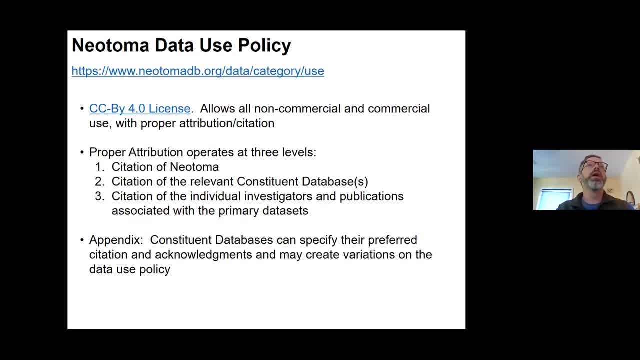 a global synthesis with thousands of records, how do you cite them all? that's where, as we'll talk about in a couple slides, having things like dois and data identifiers makes it possible for people to trace back the work that they're doing at the global synthesis scale all the way back. 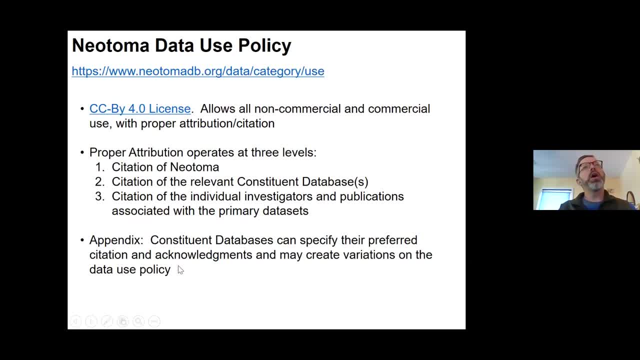 to the individual site scale. and one thing we allow is that you know constituent databases can clarify how they want to be cited. so if you want to be a constituent database and say we want to be recognized in this way, we can easily amend the policy to support that. 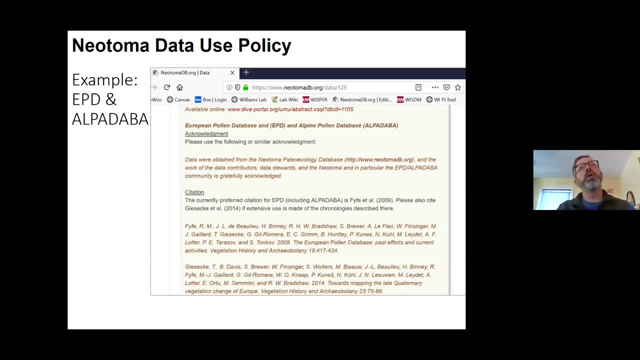 so, for example, the european pollen database- oops, a little typo though there- and the alpine pollen database, alpadaba, in our data use policy specify how they would like to be cited and some of the specific papers that they would like to use as our citation endpoints. so that's a way that if 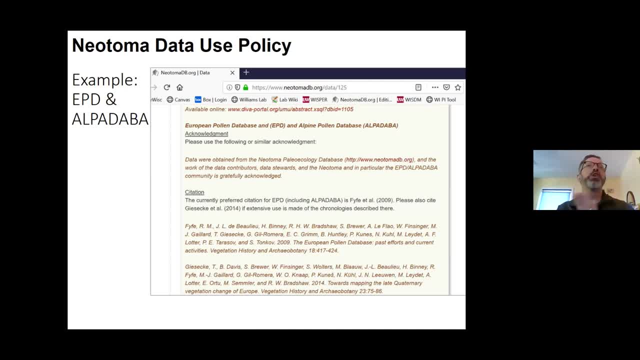 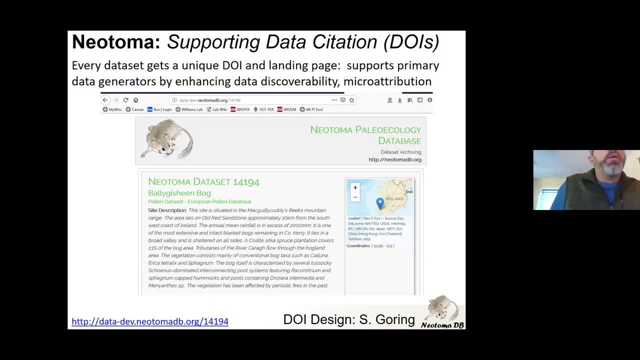 you want to use neotoma and epd data in neotoma. here's how to cite it appropriately. um one, as i mentioned a moment ago: uh, we now assign dois to all data sets in neotoma, so every, every data set neotoma gets a. 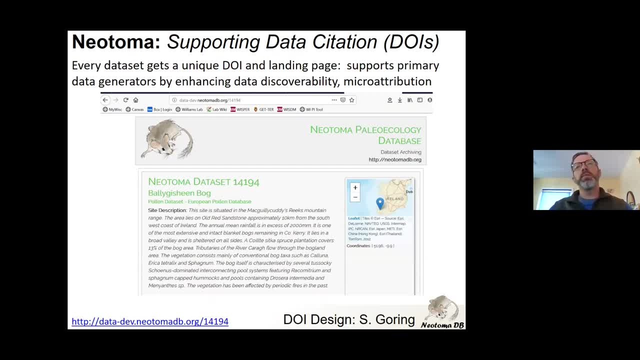 unique data identifier. this has been work led by simon goring working with a data site, uh minting service for dois, and one of the things that's uh in in temporary hiatus is we're doing this migration but is ready to go. otherwise is um have having every data set having its own unique landing. 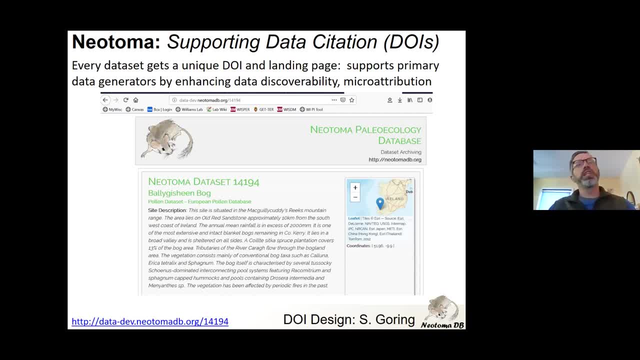 page with its own unique web page. um, that gives some a quick summary of the site and its characteristics, of the data at the site- and this is really well suited for, you know, web crawlers like google data sets or other kinds of automated services to go find your data. so this is an 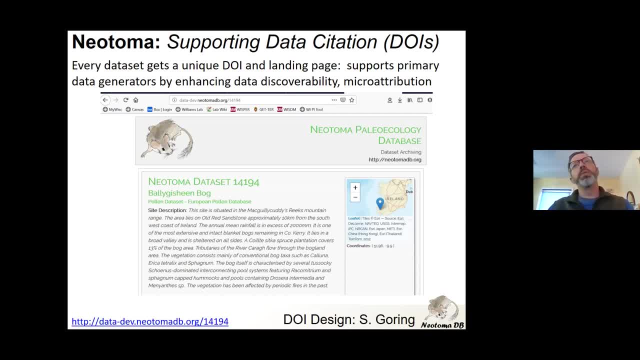 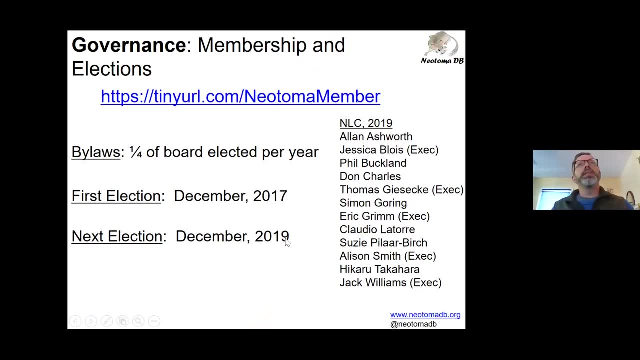 approach that we think will really help improve the data discoverability and the ability for people to find data in neotoma and use it for all kinds of different things and oops uh, that year out of date. But in terms of the governance, it's really important to be transparent about how. 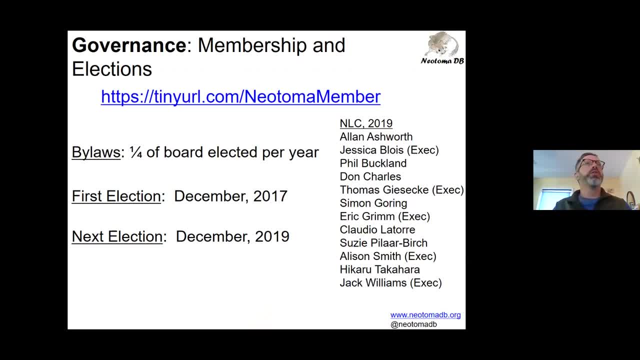 governance works, And so we have the leadership council. the leadership council, people serve four-year terms. We run an annual election in which one-fourth of the board is elected every year, And we have our next election coming up in December of this year. And then the 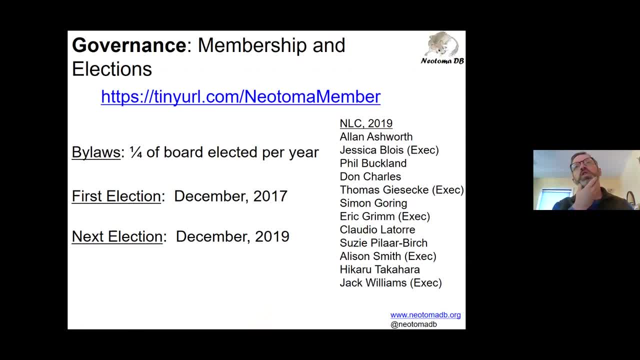 leadership council then appoints and internally votes for the executive members And the executive. you know the leadership council meets, you know, a couple times a year And then the executive group meets, you know, maybe once a month or so to kind of move things forward and move things along. 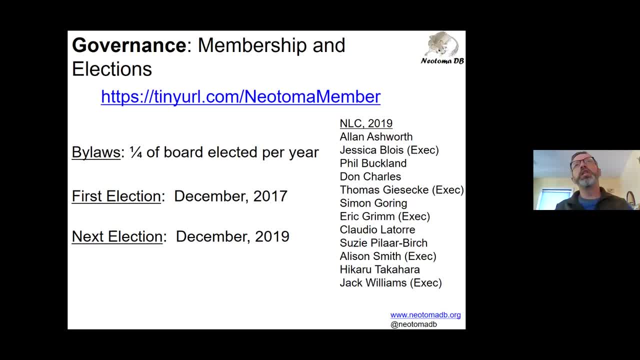 Oh, and who elects the leadership council? Well, the Neotoma members do, And if you want to become a Neotoma member, we also have a basic open membership policy. So if you'd like to join Neotoma and become a voting member that elects the leadership council, just go to that link there. 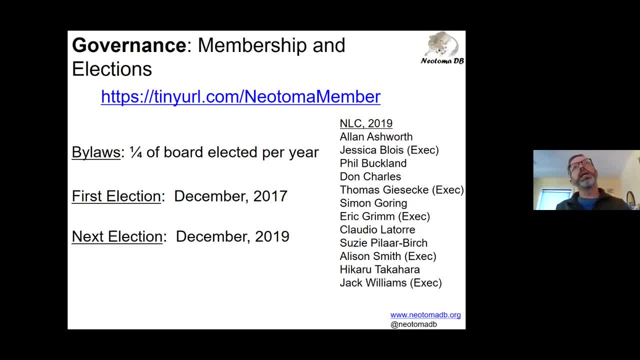 and sign up. We will just do a very quick screen to make sure we're not getting some kind of- you know, random troll or bot in there, But of that, that's a very, very, very low bar to pass And the default is that people are joining. 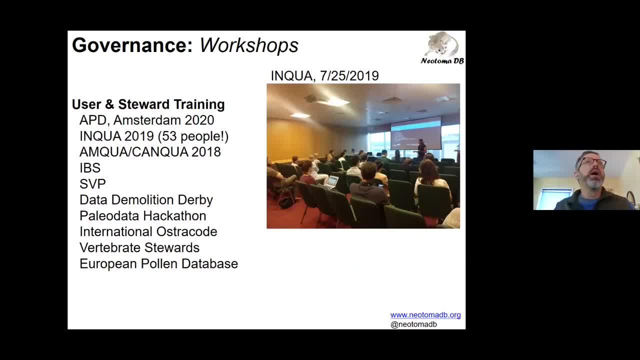 us as members. We also run workshops to get people trained how to use Neotoma data. We usually have sort of two standard workshops. One is to sort of train people in the software services like the Explorer or the R package and how to use those, And then we have another. 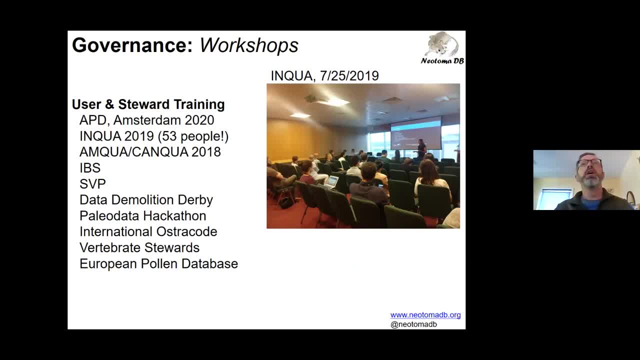 workshop series. that's that's. you know a little bit of a. you know a little bit of a. training that's aimed towards the data stewards, teaching people how to use the software and how to you know, get, get trained to start to upload data into the Neotoma. All right, Let me just 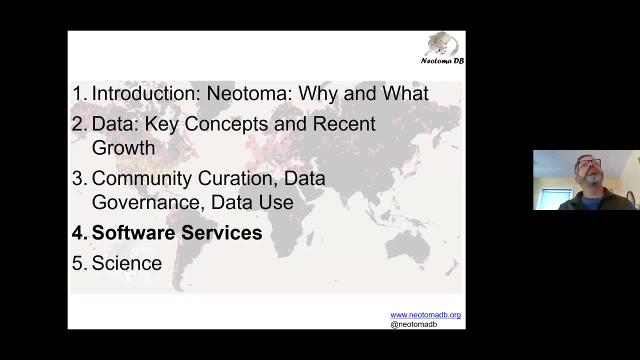 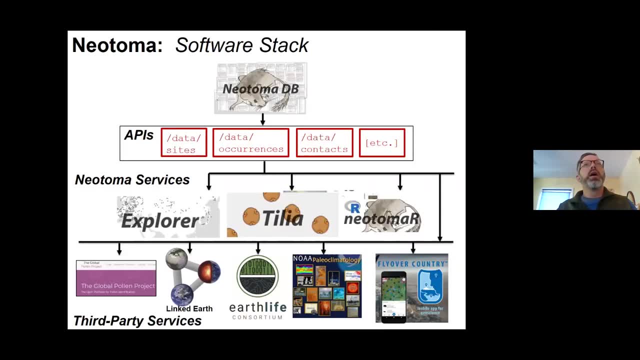 check time here. All right, Okay, So talk for maybe another five or 10 minutes or so. Software services: the kind of things that we support. This is a slight redesign of that figure I showed earlier on that kind of clarifies. 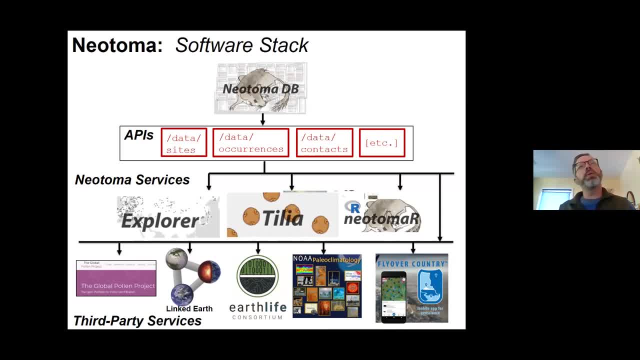 thinking about this as a software stack. This is kind of common concept now in the kind of the online database and software development world, where you kind of have a whole stack series of software layers And I've. you know, I've sort of gone from top to bottom here, in which, at the 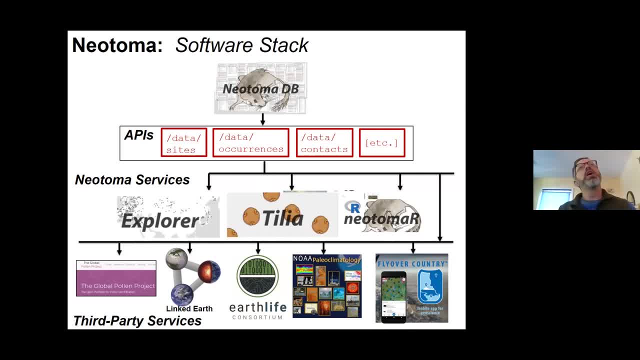 top of the stack. you can also think of it as like a foundation. on the bottom of the stack You have the database itself, the relational database and the data stored in the database And and that's kind of primary archive point, And then that's sitting on a server somewhere. 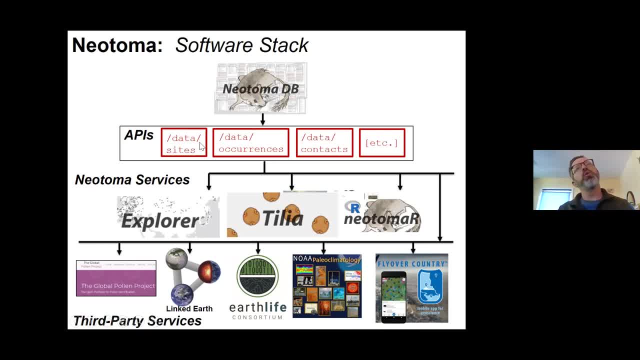 And then you have the APIs, these programmatic endpoints that allow people to query into the database, which otherwise is fired wall. Then you just can't go in and start to touch the data willy nilly. but the APIs are specified programmatic access points that allow you to go in. 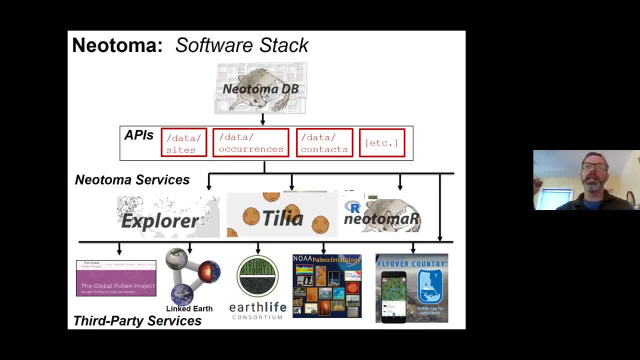 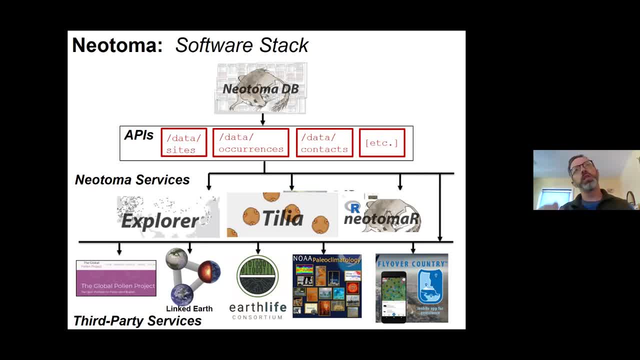 the outside world to access into the database, mostly for the purposes of getting data, And then the software services explore Telia and the Neotopa R package all sit on top of or, I guess in this model, underneath- the APIs and then use the APIs and then create these different. 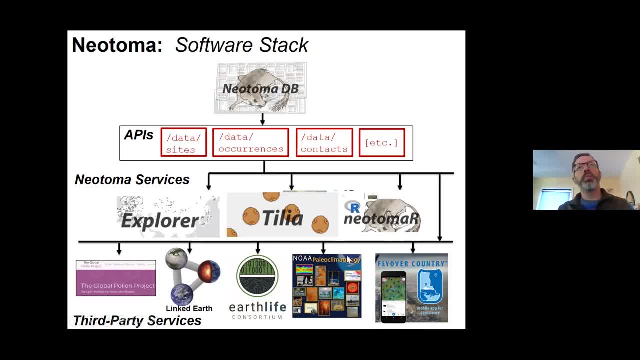 user interfaces, And then other people have built their own services based upon these APIs, And so if this kind of sort of API structure really allows lots of different people to build their own tools and resources using Neotopa data in lots of different ways, 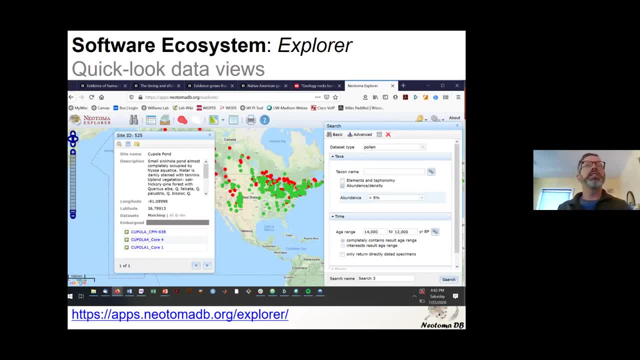 So explore is designed for kind of quick look visualizations. It's great for teaching purposes. I use it all the time for just kind of looking up sites like: Oh, such and such a site by such and such a person, what does it have? And so here's a quick lookup for cupola ponds. 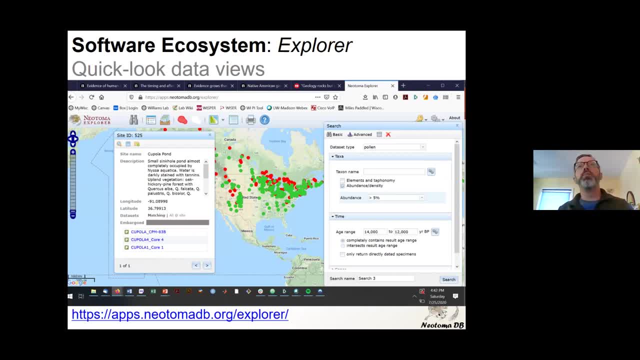 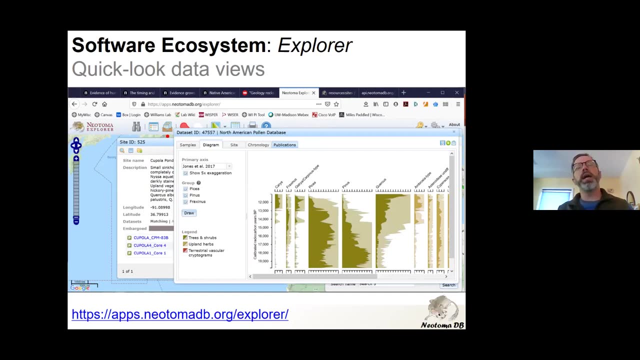 in Missouri. You know I did a search for all pollen records that had data between 14,000 and 12,000 years ago And- and here's what I pulled- and took a look at cupola in Missouri. Once you've picked a site, you can do it. You can build a quick diagram of all the 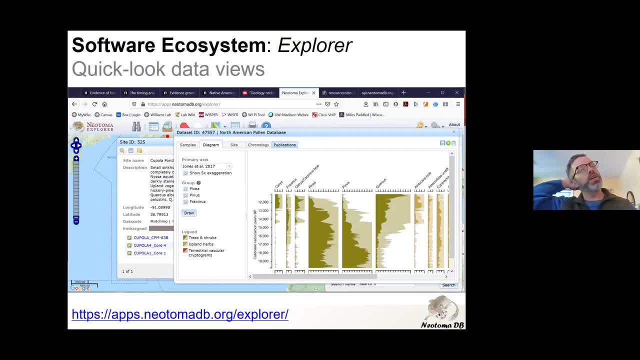 tax on the site and their relative abundances. So sort of a classic quick look pollen diagram or stratigraphic diagram, currently supported only for pollen, but we have a you know on local developments- almost ready for public release, a version of this that will work with any data type. 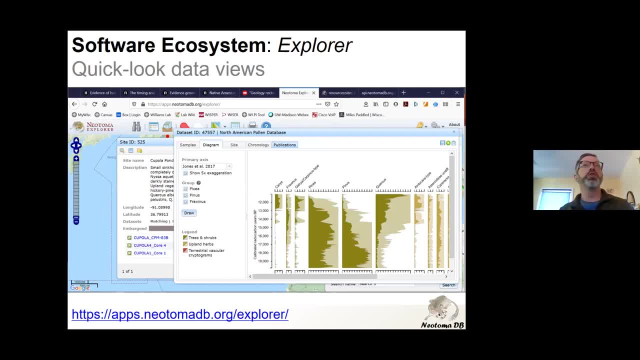 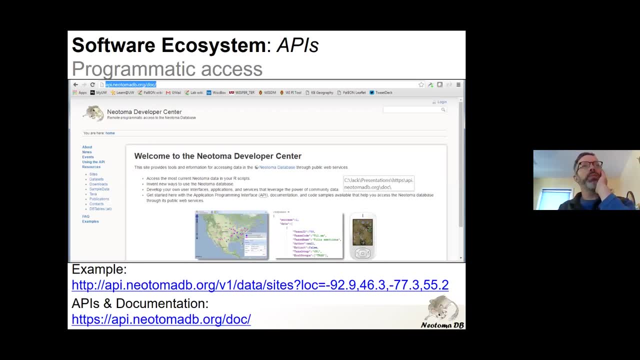 in Neotopa. So Okay, Great. So this will be extended very soon to many more data types in Neotopa. And then we have the API is the programmatic interface, And I won't go into those here except to say here's the URL If you are interested in building your own tools or 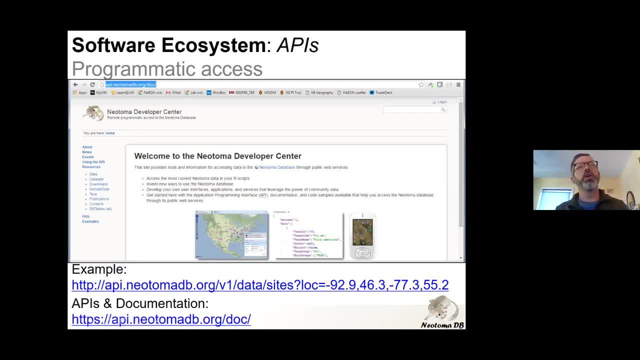 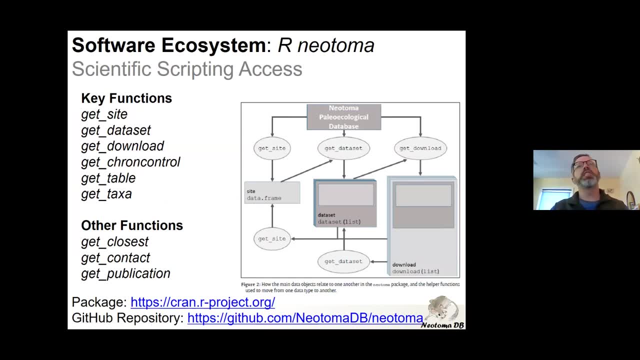 building your own ways of doing programmatic access. you can go here for more info. And then the R package. probably most people are doing scientific applications often work in R these days, And so we have the R package that has these definite, various defined functions. 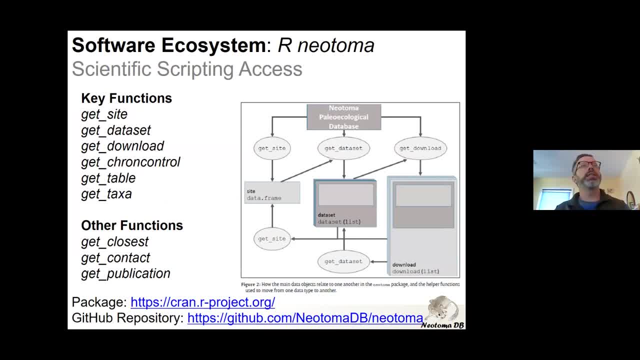 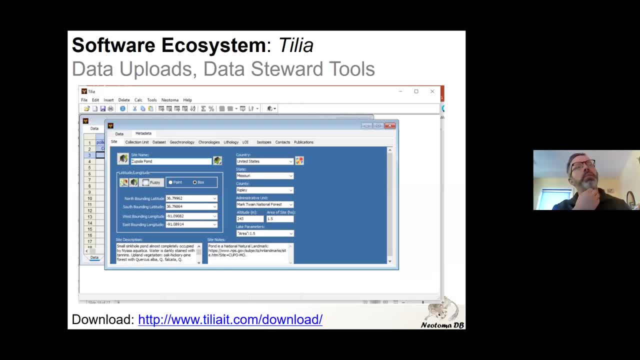 We're getting data out of Neotopa and grab there, And then Tilia. Tilia is this, you know windows based package for looking at the data and metadata. It's very site-based, So you can kind of go a site at a time and you can then look in great detail. 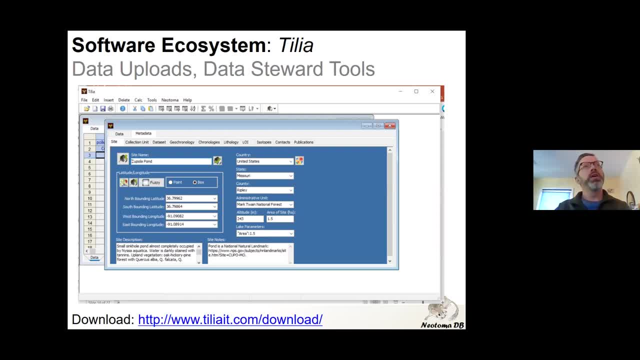 the metadata for that site, the data for that site, And you can both download data from Neotopa into Tilia and look at what you got and use maybe some edits to it, if you're a steward, and then you can push data up to Tilia. And there's a couple of different versions of Tilia out there. 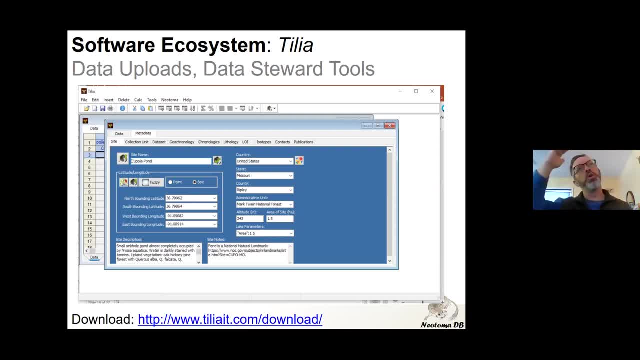 And so there's a standard version that anybody can use. that would let you pull data from Neotopa and may say, make up a pollen diagram, other kinds of basic things. but only stewards can upload data to Neotopa. They have a password or user account, So it has restricted access for uploads to Neotopa. 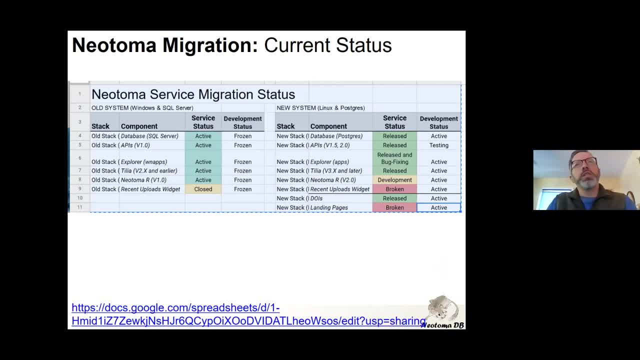 So that's a really good way to get your data back. One important thing that's you know. this is: you know, for this moment in time, over the last month or two, we've been going through a big, big, big migration process, which everything I've just 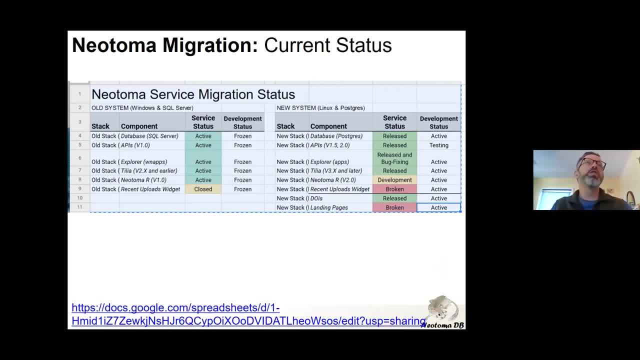 described to you used to be based off of a windows server, with SQL server as as the relational database sitting behind everything we have been. we have been, over the last couple of years, been moving everything over bit by bit to have it to a Linux server and having a Postgres database as the 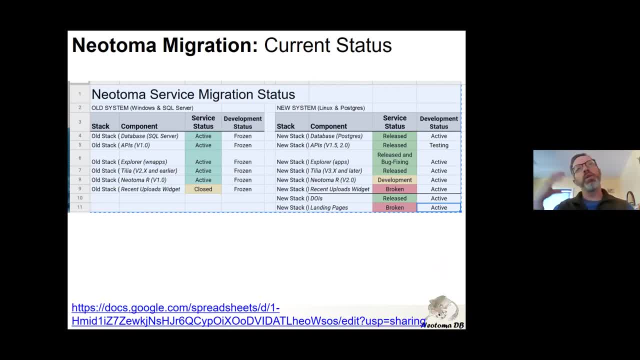 back end, And so we have been moving the database over and then we've been, you know, redirecting or revising all the software to point to the new database, And we're now we're in this sort of, you know, kind of midstream point. 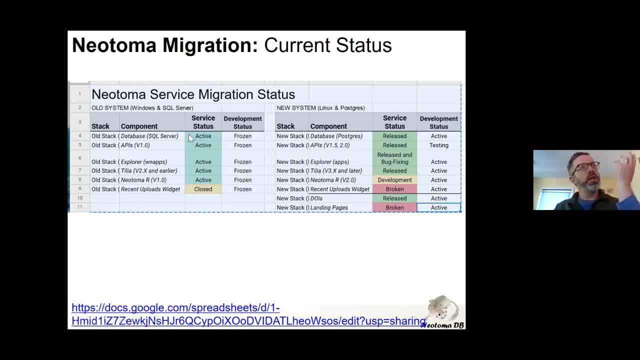 where, on the one hand, we have the windows version of everything that is all active but frozen. We're not. we're not changing them anymore. The database itself is not changing anymore, And now we have a new version, the Postgres version, in which the database is released. 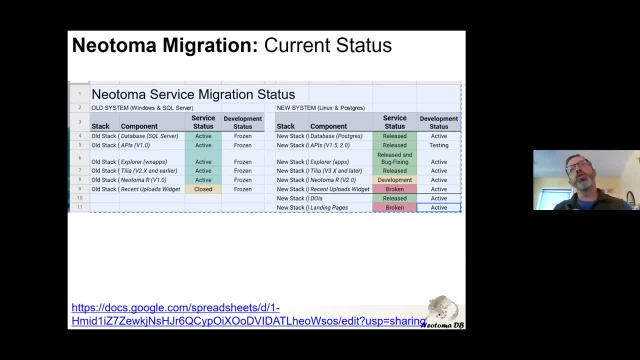 we are now doing some test ads of data to it through Tilia, So it's starting to become the living version And you know we are in the process of making sure that all the software services work. So we have the kind of this current of the moment software status And because we know 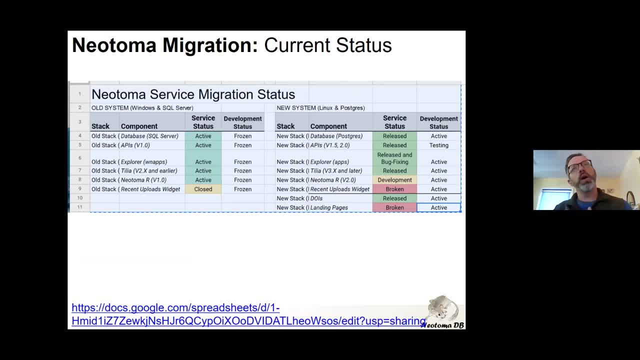 that people are using- you know, our services. they want to know where, where, how things are doing. We have a spreadsheet down below there that we're going to be sort of updating weekly to kind of give updates of where things are, what the status of things are And the Slack channel. 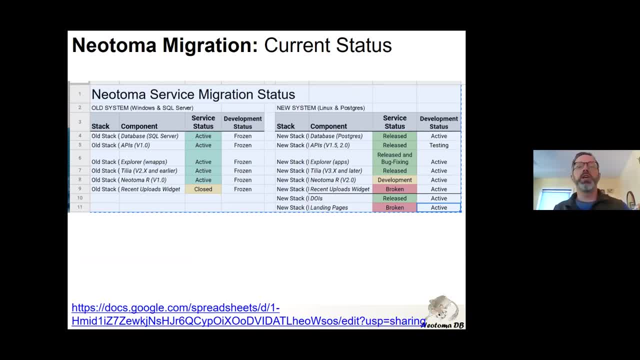 is also a good place to keep track of this migration process and where things are. We want to get this done as soon as possible because we want to move on to building new things and not just migrating over current things. So if we think about what's next on our 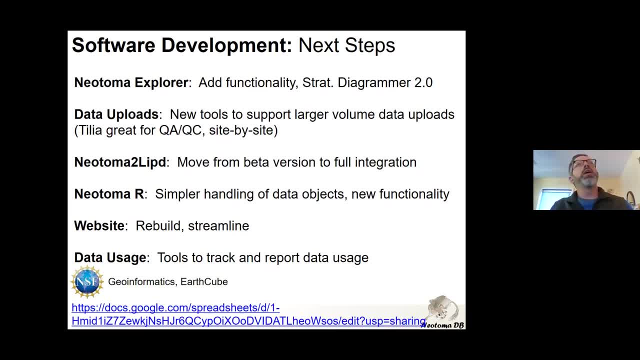 kind of our to build and to do list. you know we want we have for explore. there's lots of little things we want to do. We want to release that stratigraphic diagram or 2.0 that I mentioned. you know it's like we. we basically like explore as is. but 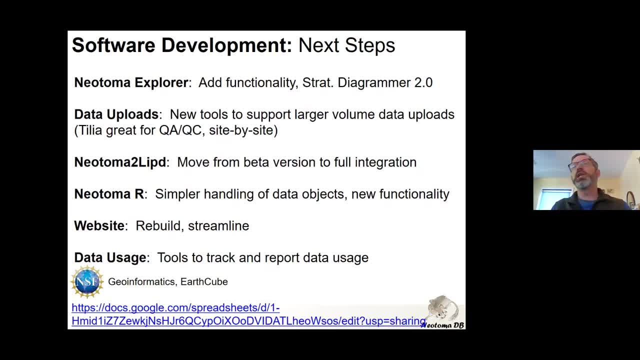 there's lots of little cosmetic tweaks, a little minor fixes and improvements here or there. we want to do that will make you know, improve life for people, based on what user requests have come to us. We want to, as a kind of a major new area that we're kind of we'll be working on over the 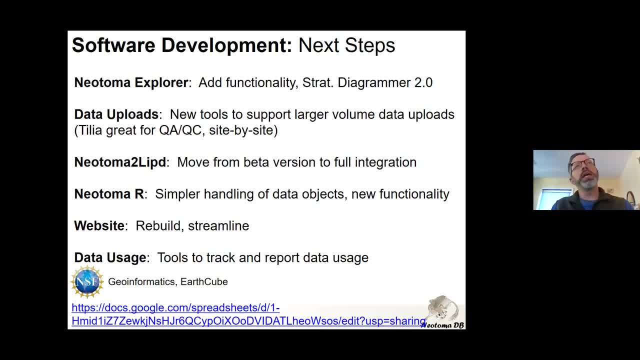 next year, a couple of years is. you know, right now Tilia is very much based upon a one site at a time model And that's great. but it's hard if you want to say import in, if you're a. 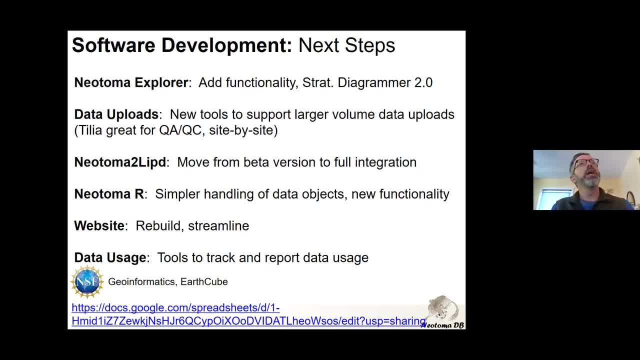 constituent database. you've already got a thousand records that you've you've got on hand and you still have to work on. you know you'll be doing a lot of the work that you're doing, but you've got to make sure that you're building those relationships as well. 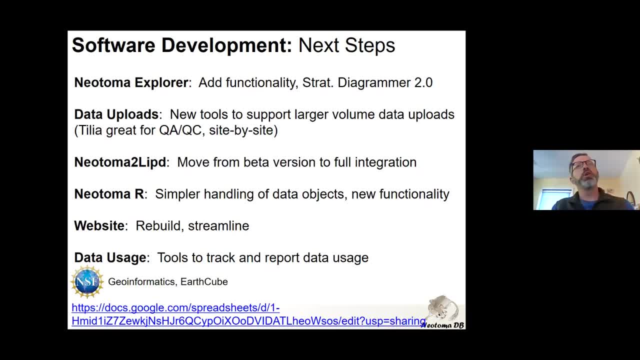 So how do we get, how do we make sure that the data that we're going to get is is accessible to people in the context of the data that we're using? So, from a data perspective, you know, Tilia is a bit of a slow process to go everything. 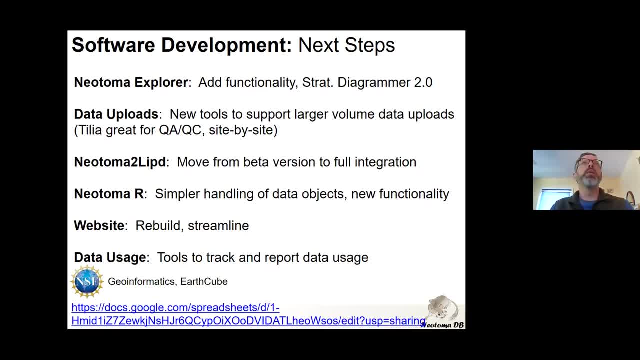 through Tilia. So we want to create new tools to allow our larger volume data uploads, And so we're kind of starting to build build some new tools for that. This is at the very, very, very early design stage right now. I don't think I've mentioned it yet. 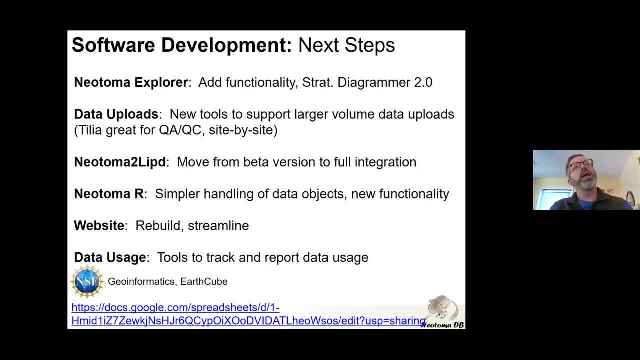 but Nick McKay has been working on an exporter of that already and we want to move, just keep building that out and integrating it more and more with our services. um, we want to. you know we're going to be. simon is going to be building doing a new release of the neotoma r package, a 2.0. that will some of the- there's some definitely 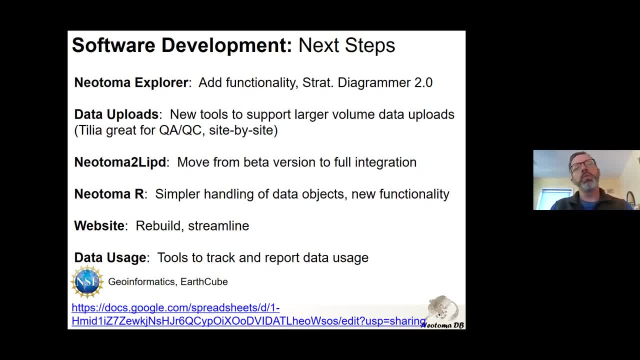 some clunkiness in the current version of the neotoma r package. we want to make that simpler. we want to add new functionality, response to user requests, and we're also at the kind of the early design and development stage of that that will be a fall priority for simon um. we want to rebuild. 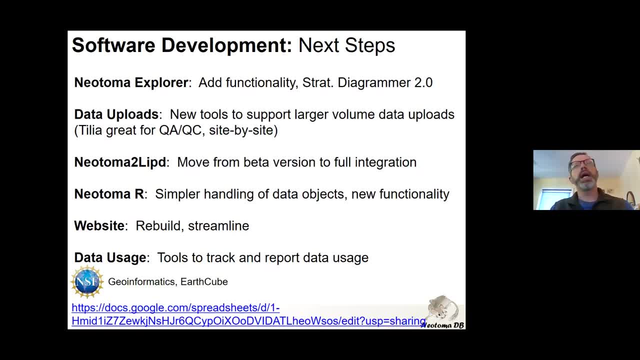 the website um, and we want to get better tools for tracking our data usage goes, so that at neotoma, we can tell our supporters- you know, here's all the you know things that we're doing and supporting- so we want to, you know, be able to track our usage and impact. and then we also would like to make 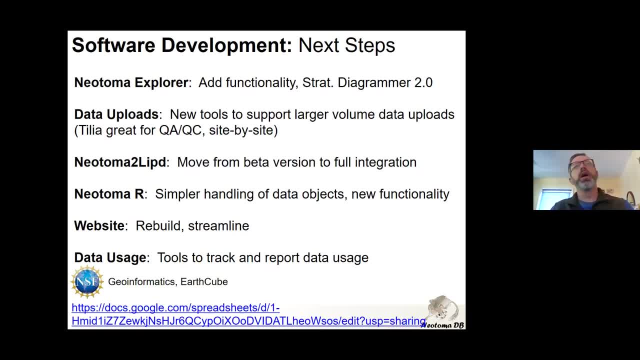 these kind of services available for our individual data contributors as well- letting people know whether their data is getting cited and used, and so forth, and all the things above there are being supported right now by the neotoma r package, so we want to make sure that we're able to do that. 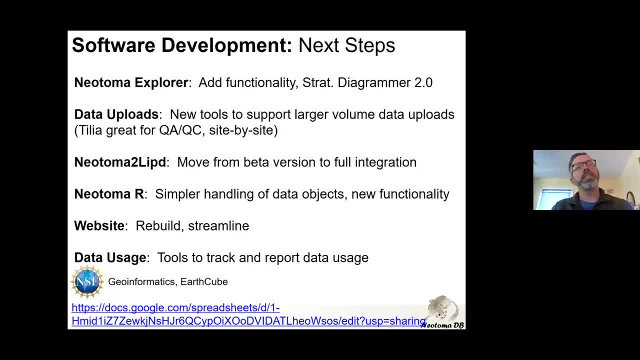 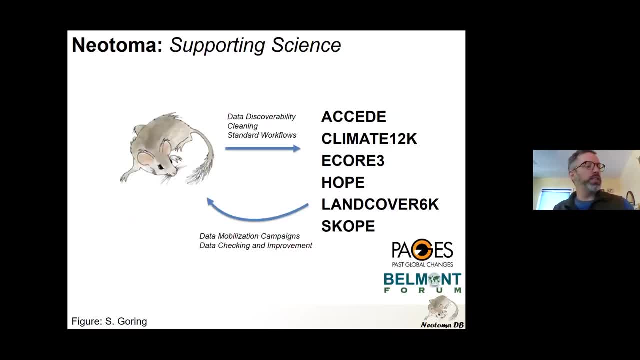 and that's the last thing to say- is that geoframmatics is a national science foundation and we have a three-year geoframmatics grant that we've got about two, two, three, four years on. i'll just say a few minutes about science. you know i've spent all this time talking about 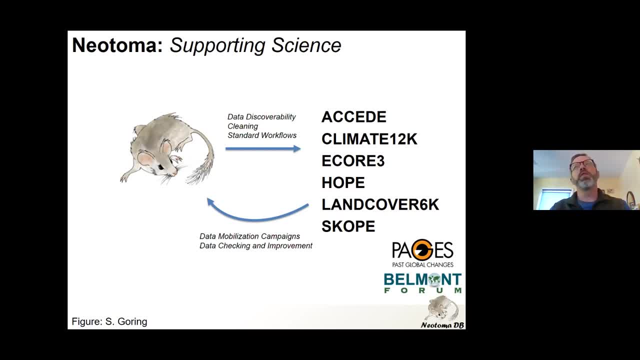 infrastructure and and data models and so forth, and it's really easy to go down the rabbit hole of building these data resources and software services, and that's great. you want to do that. Are you making, are you powering new kinds of science that couldn't have been done otherwise? And so you know we, as an open resource, recognize that to some degree our effort will make other people's science better. right that we don't expect to be co authors on. 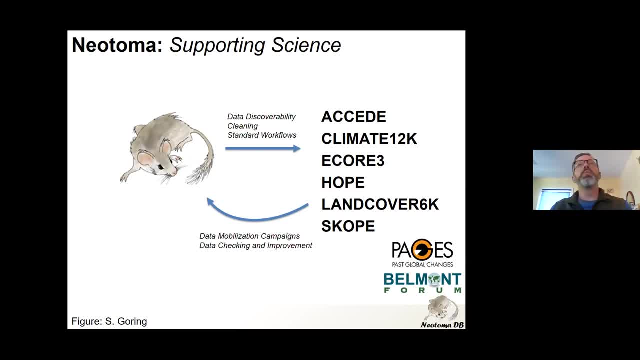 every paper that uses data. We have our own sites that we want to do, that will be a part of, are happy to participate in. But so some of these projects that right are these kind of regional to global scale synthesis projects, some of which were involved in some of 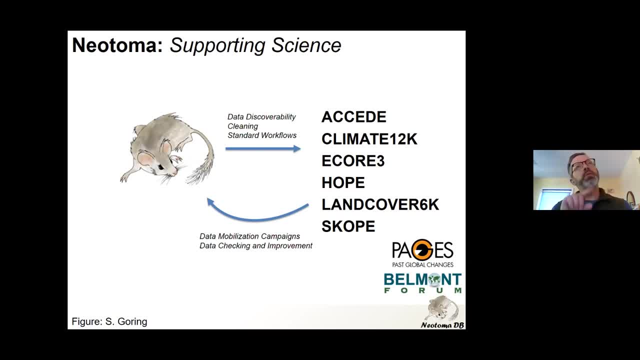 them and that's all all to the good and that we really see, but we do want is to make sure as much as possible this is a two way loop that need to help us provide data out to these different efforts and these different, these different efforts. 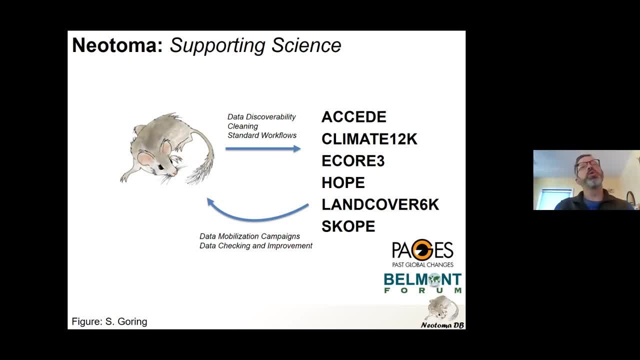 return value back by doing things like training data stewards and getting new records added to the Atoma that we didn't have yet, by helping with data checking and improvement, age model updates and all the rest. so we see this sort of two way synergy between the Atoma, providing these foundational services and data, and these other projects doing these kind of global 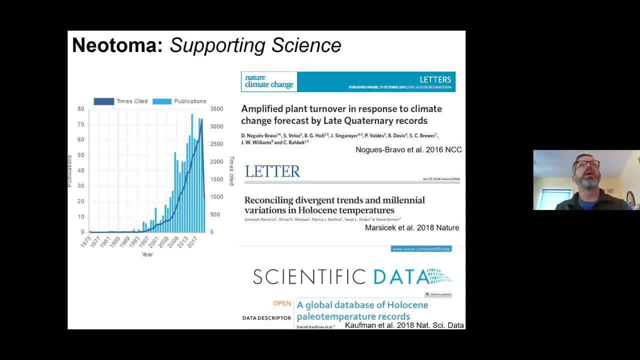 value added, science oriented projects. You know I think we've been successful there, so we see this sort of rate of tracking, a publication rate of papers using the Atoma data left there A few highlights of some different papers that have used the Atoma data, some you know: the nature and nature climate. 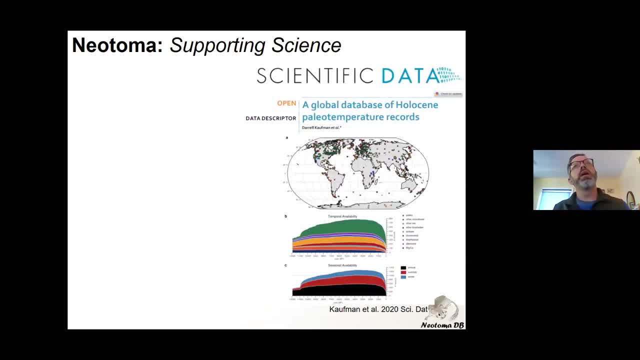 change papers. that right there. And then just kind of one example, this is, you know, Daryl's moderating this appointed one of his, his papers, where you know he's of course been really leading this effort. This is a very, very, very commendable effort towards building global paleo climate data products and inferences that are fully open and transparent, where you can look at a map like this and trace it all the way back to the individual records. 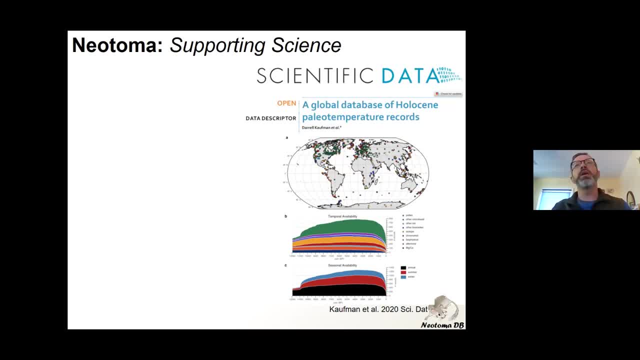 that powered this. so really making sure that we are doing transparent, open science, that we go to a congressional hearing and say we know the world is warming, that we could in principle, documents and provenance all the way back to the first point of origin for these data points. 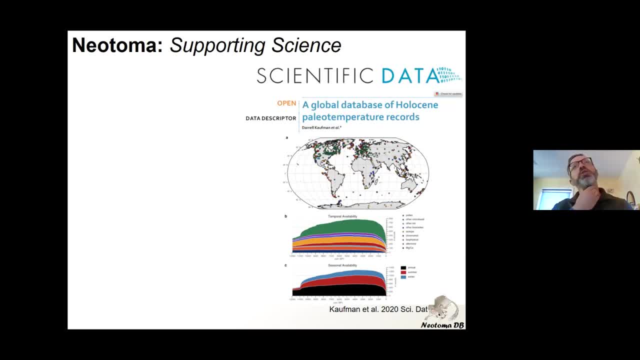 So. So this is a data paper that presenting this new database of policy paleo temperature records. the green dots are pollen. probably most or all of those green dots are the Atoma records and, you know, pulling in other sources as well, so this isn't all the Atoma. 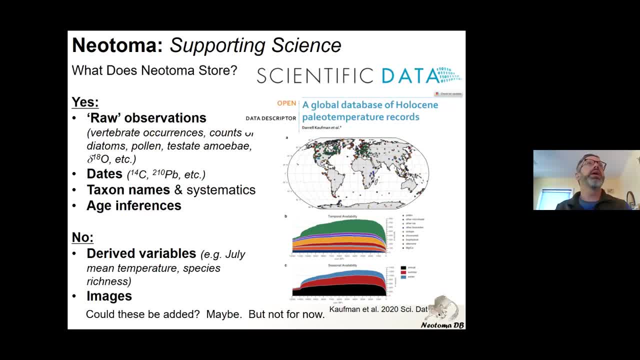 data, something that is definitely the Atoma data contributing to this, And, as I put this together, I thought it was important to make an important point about what the Atoma does and doesn't store, because I think this is a good example of thinking about that. 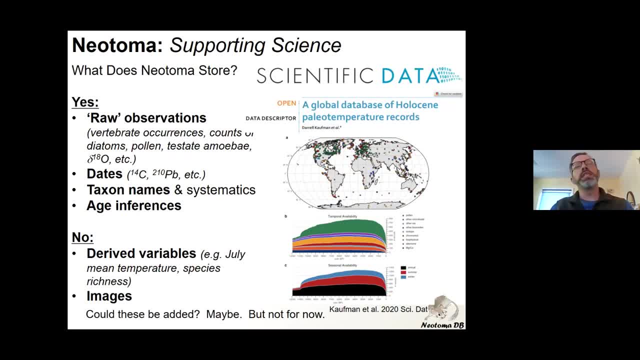 And this is as much as possible. the raw data, the occurrences of bones at different site, localities, that counts, or abundances of diatoms or pollen, or ostracized or what have you. You know geochemical measurements such as stable isotopes, the radio carbon dates, the tax on name, the inferred ages, Those are things that the Atoma does store. 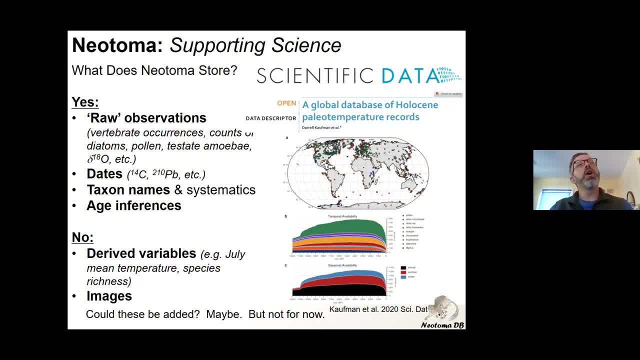 What we typically have avoided storing so far are the derived variables- July mean, temperature, biodiversity indices like species richness or turnover. those more derived products We see as outside our mission, And so for us, we see what we do at the Atoma is very complimentary, for example, to what you know- this, this paleo temperature product- because we're kind of more of a foundational data layer that stores the raw information. 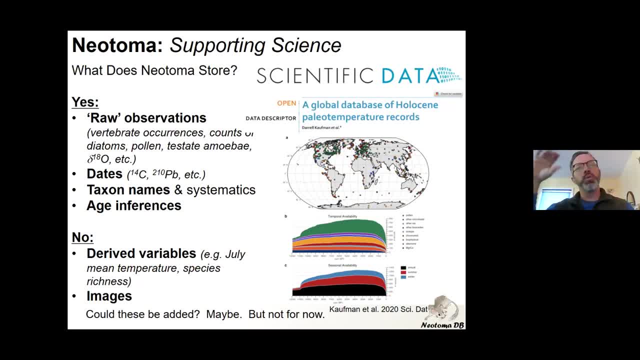 And then this is more of a derived data product. with this very you know how did you get those temperature estimates and you know certainties of them and the methodologies of that. That's all information that's largely stored outside of the Atoma. but 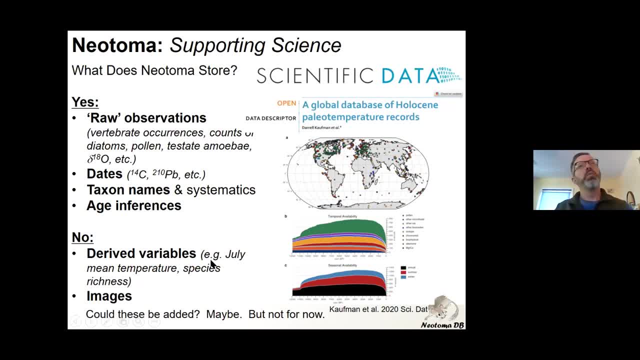 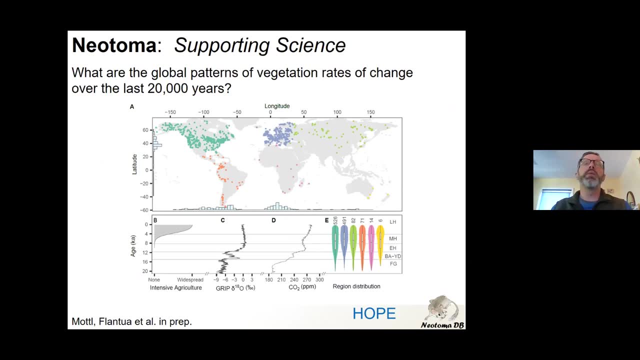 this and founded upon the Atoma. We don't store images. just another example: There's no hard rule that we couldn't do these things, but we're not. they're not part of our core mission right now. Another project that I've been involved in recently, and this has been with the HOPE team led by John Burts and others in Bergen, Norway, with Andre Andre Model and Suzette Flantua- some of the key leaders in terms of doing as postdocs, doing the active work. 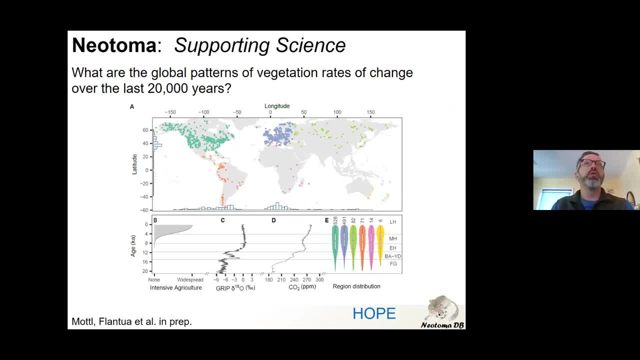 This is a project we're working on. This is taking some of the currently available pollen data in the Atoma. This is roughly a April to May snapshot here- And then basically asking what are the global patterns and rates of vegetation change over the last 20,000 years? So that's our site map. up top the lower right plot shows our time distribution of these different continents, data distribution and then some of the 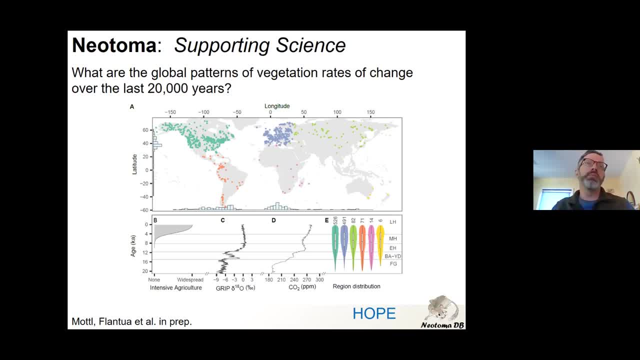 standard things that might be causing vegetation change in plots BCD: Growth of human agricultural and land use. climate represented by grip and climate. Growth of human agricultural and land use. climate represented by grip and land use by grip and co2 rises. so it's a representative important time series and last slide or two um. 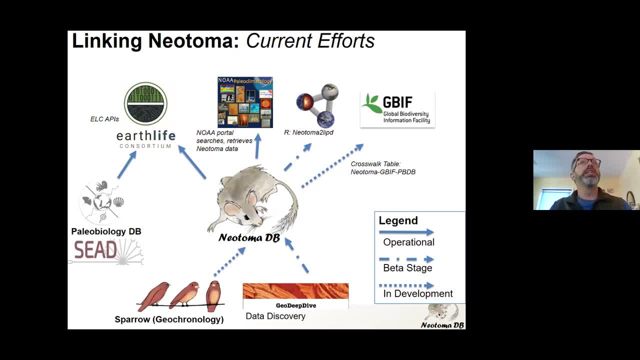 i just want to mention this, and there's a lot here, so i won't go in this detail, but let's know that we can come back. we're going to talk more about it. you know, neotome is part of a larger ecosystem. there's some kinds of data that we curate and there's other kinds of data that other people 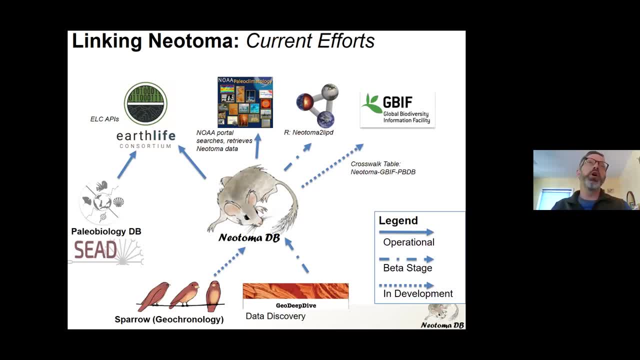 curate, and so big goals. in addition to kind of building our own internal data resources and bringing data in and building new tools to support the kinds of things that we want to do, another very important mission is to better link out to other resources, and so this is just kind. 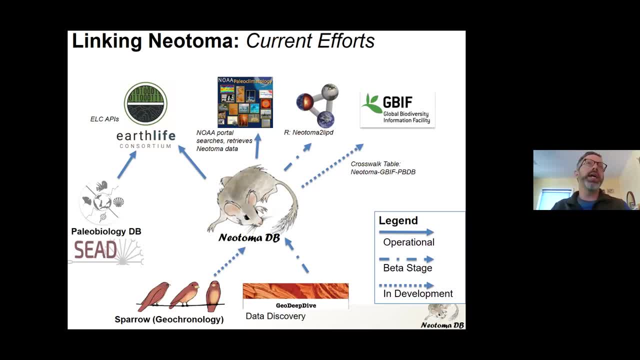 of a quick summary of some of the active, like partnering and data integration and linking efforts that are underway and you can see there's the noaa portal that i mentioned before, the earth life consortium linked earth and this lipid neotoma to lipid exporter. so there's more. 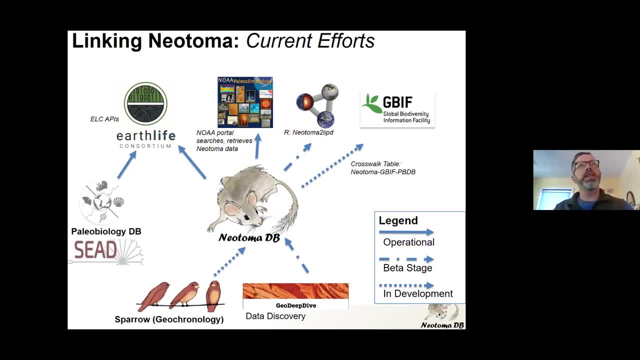 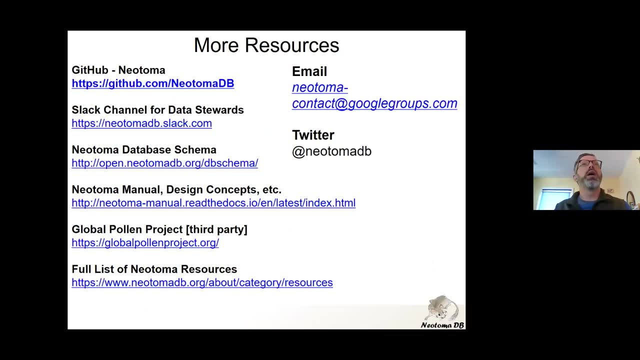 going on there and i'm happy to go circle back to any of this, but just to kind of say that you know we see ourselves as part of a broader ecosystem and that we are one node in a larger network. i'll kind of just finish here by just kind of leaving up some, some summary resources, i know. 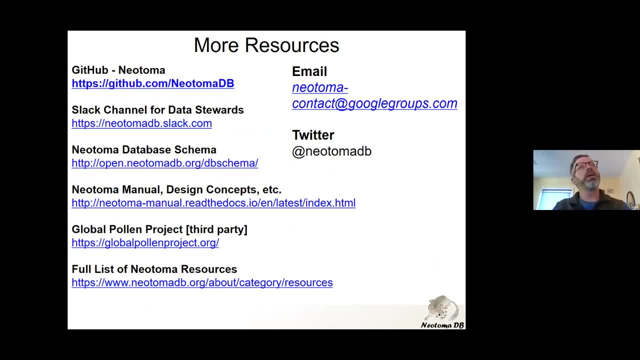 i've covered a lot of ground quickly, and so here are some of the links of different kinds of things that might be useful if you want to learn more and, as always, you want to drop an email saying, hey, i'd like to become a data steward, or i'd like to contribute data or like to learn more. 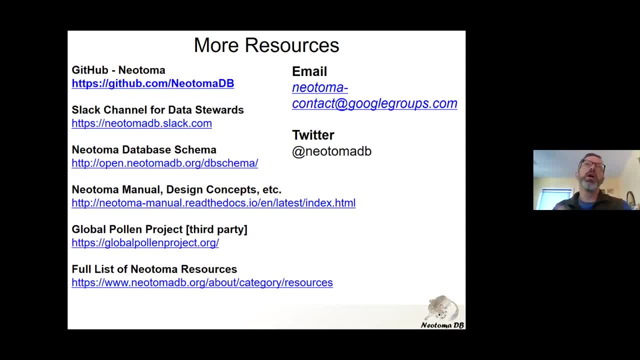 how about use the r package? just reach out to us by email, by twitter. you can email my personal email address, happy to talk more, and i'll just finish by again thanking everybody who's contributed to this, and i'll open up for questions at this point. so thank you. thank you for your time here. 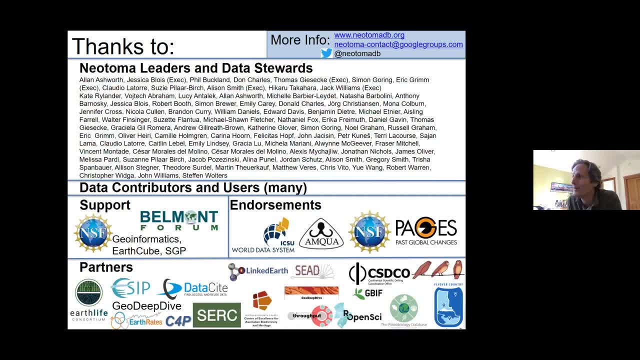 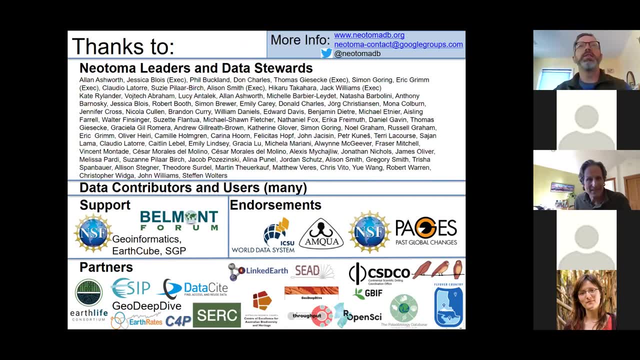 thank you, jack, for that very informative review of neotoma and its many functions. so let's see, i'd like to open it up for questions. feel free to uh join in on the the chat and i'd be happy to moderate that. um or um, you may open your. 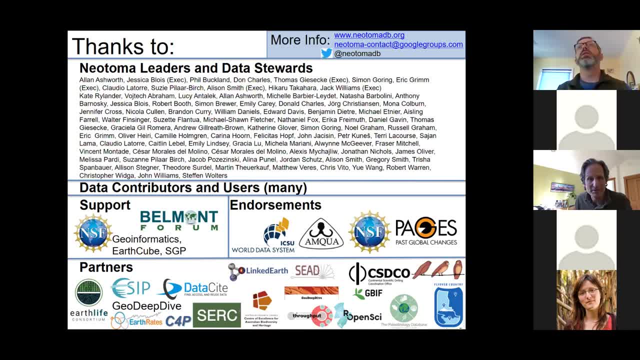 mics. i believe sarah participants have that ability. um so let's see. uh, our friend mike evans has been busy on the chat. mike, do you want to open your mic and choose among the the topics that you've already brought up in the chat, or can you do that? uh, yeah, sure, hi. 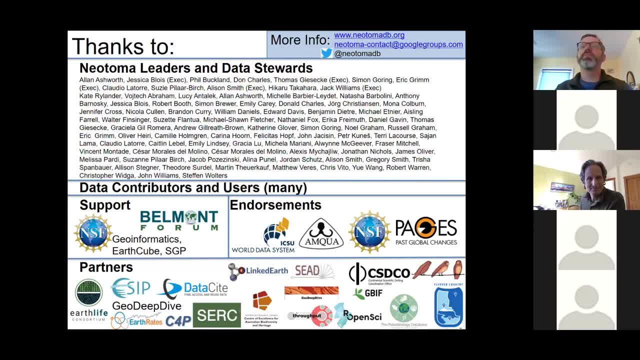 can you hear me? okay? yeah, hi, um, this was fabulous and really fun and a great introduction for me. let me ask just two the questions. well, one question in the chat and then one a science question. the question in the chat is i? i saw that bruce bauer was also here, um, and i was wondering. 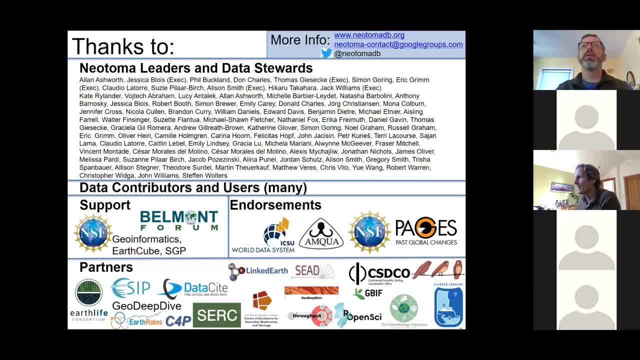 if, between the two of you, you could compare and contrast um, like the, the wdca, paleo with neotoma, um. the second question was more science related. i was wondering to what extent you have explored, um, uh, the, the spatial and and temporal biases and the sort of of syntheses you you were showing in the. 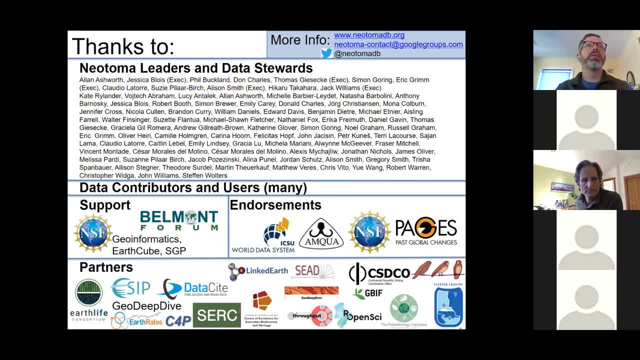 um in those last few figures, the, the rates of change in um in uh in ecosystems over over time. thanks, great questions. both. let's do the first. let's go in kind of first and second. um, bruce, do you want? i just kind of gave my neotoma spiel. do you want to talk maybe for a moment or two about wca and 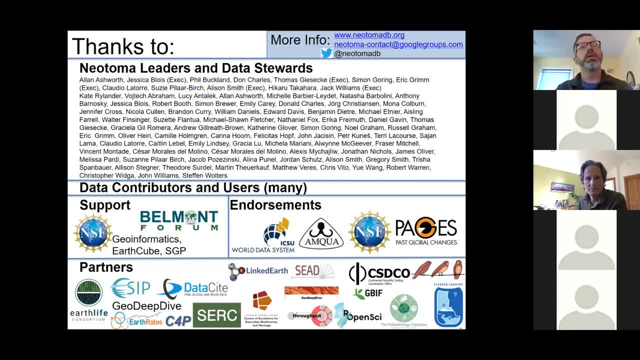 similarities or differences and you're um not not hearing you maybe your mic off, i will, i'll start and then and then chime in. um, yeah, i, i, i think obviously some very similar missions right of you know, make you know. archiving and making available data, um, obviously is a different sort of a. 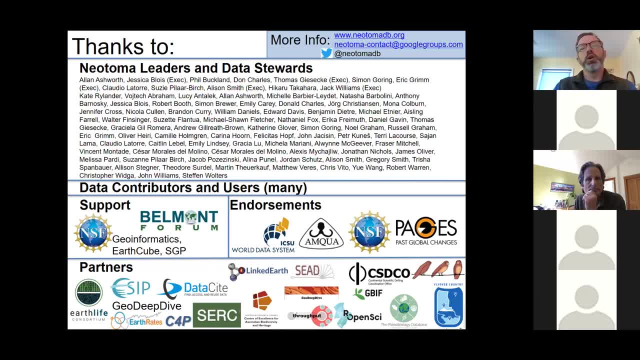 different scope in that you know, you know, noah, you know, is seriously focused on on climatic data. and you know, no, no, noah started earlier, when the mission was really focused on paleo climate and understanding the past climate system, and that proxies were gathered in service of that mission. 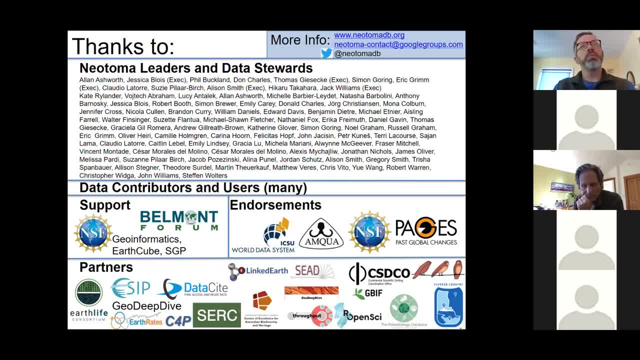 um neotoma, is really focused on understanding ecological and biosphere dynamics and sometimes overlap because, say, pollen is a well-established paleo climate proxy and it is also used to study, say, vegetation dynamics. but then there's other things, like vertebrates um, which aren't as widely 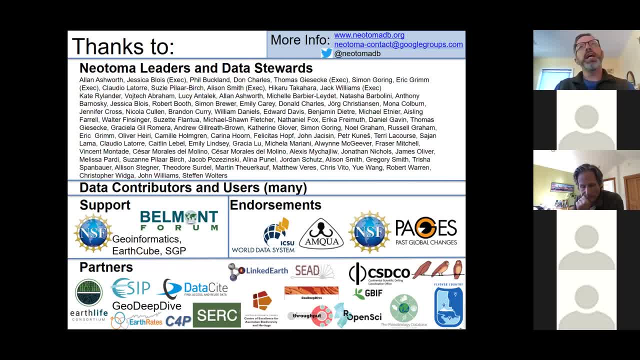 used as paleochromatic proxies but are really important too. so it's a classic venn diagram. we can look at our data sets that we store and the data sets that wdca stores. you'd find some that would could be plausibly stored in either one, and then some that are very clearly one or very. 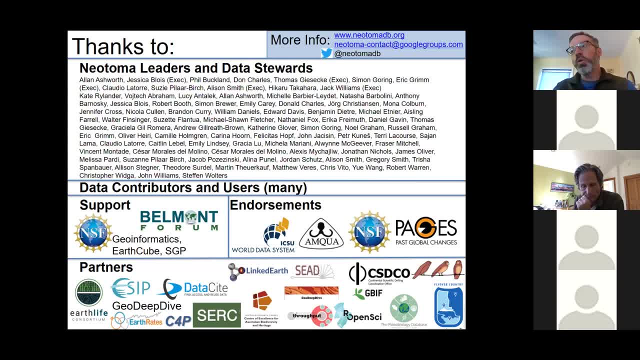 clearly the other, um, you know, that's one sort of thematic difference. and then, if you kind of get into the underlying data structure, you know neotoma, as i sort of said, is this: you know, you know postgres model, with these defined relationships and hierarchy and so forth. you know all these. 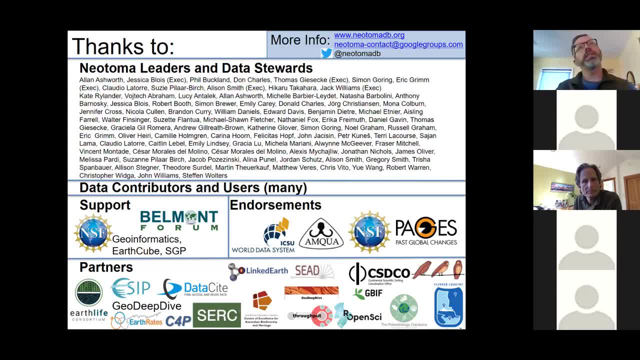 different data resources all have some underlying data model that you know at the at the surface level seems: oh, they're all the same. they're storing paleo climate data or they're storing pollen data. but those structural differences in data models end up being really important because 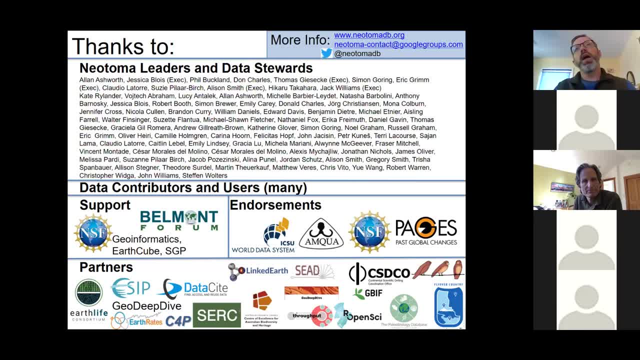 we know that they can provide data that they need, and it's really important that it has a lot of analytic leftover data and it's always gonna be a very distributed data. so i think you, you said, you said, you said it's. it's one of those things where you 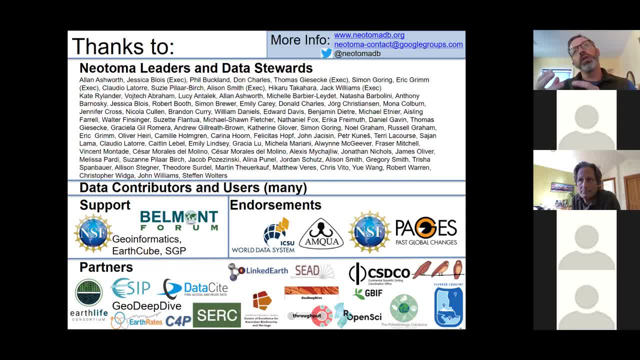 could. you could do a very long distribution of data and it would kind of do it at the same time. you know how. you know a lot of data is a great source of functions and data is limited in terms of steps. we defined internally, the way that we sort of organize data hierarchically and so forth. So 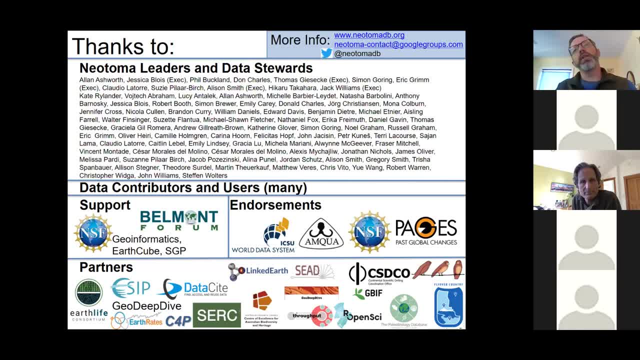 this updating of age models, which we can do programmatically pretty readily, may be harder, for example with the WCA. But, Bruce, are you there, Or Wendy, I'm here. This is Carrie Morrill. Oh hi, Carrie Morrill, You can answer this question too. Yeah, and Jack also, kind of 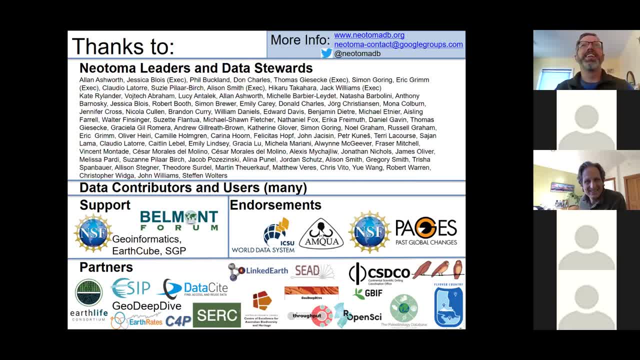 touched off. he answered a couple of my other questions already in his answer. Great, Yeah, I think Jack's explanation was great. I don't have a whole lot to add. I think that the data that we curate are complementary, And Jack talked a lot about taxonomy and systematics being 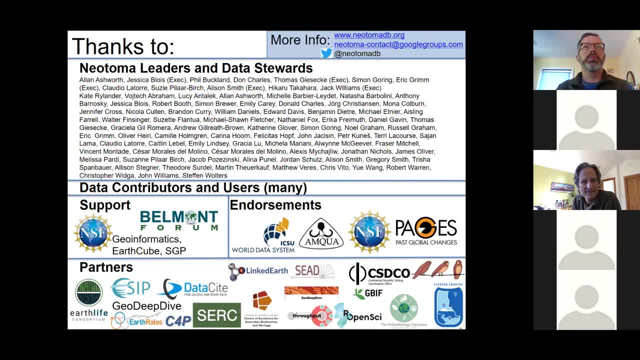 an important component of what we're doing, And I think that's a great point. I think that's a key part of what Io teme curates, And we don't do that so much at the WDS, paleo. But on the other, 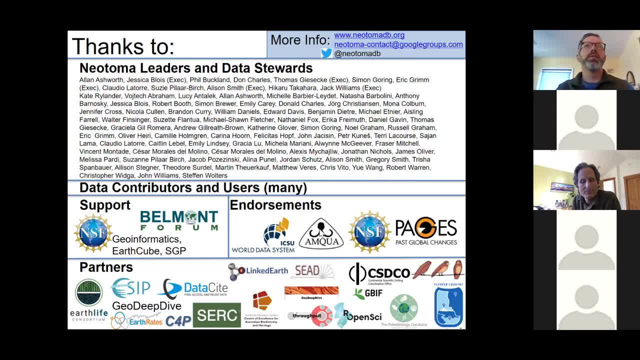 hand, we do devote a lot of resources towards curating the derived variables. So I think that's one example of kind of on the Venn diagram where we don't overlap so much. But I also really like Jack's description of the symbiosis between the data contributors and the data center. 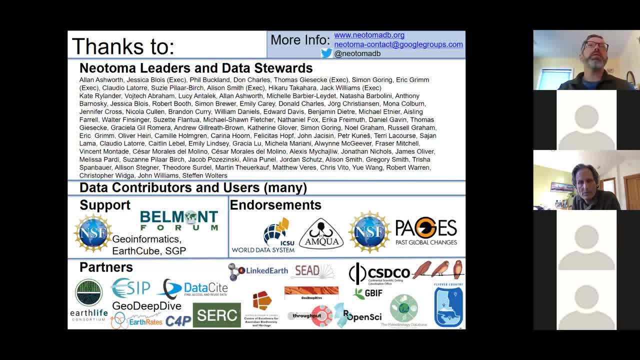 and the data synthesizers in the data center, And I think a lot of that goes on in the data center And I think a lot of that goes on in the data center at the wds paleo as well. thanks, carrie, and the tag off of that, for example. i do think that that. 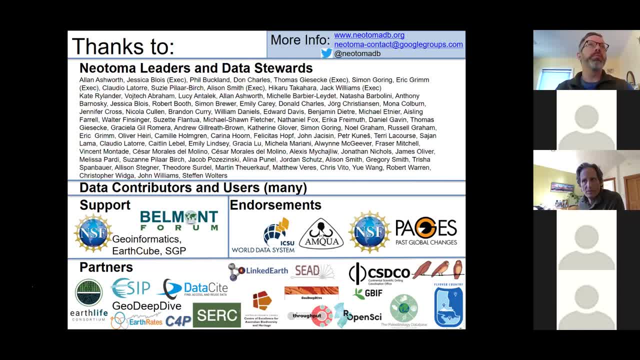 idea of these community curated data resources is really important, important as a general concept, because i do see that as something that has kind of emerged and evolved in lots of places. like you know what? noah does the same thing: people contribute their data to it. there's some 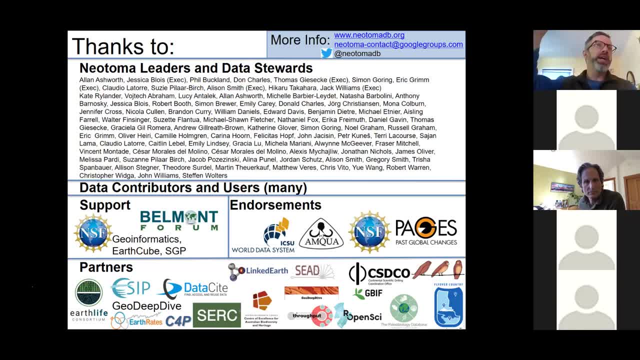 standardization, harmonization. that happens there, and then data is provided out to the data synthesizers, and so that same model that i described could also apply to noah. but you know who does the work and how it's done, and the exact model for that can vary from from resource to. 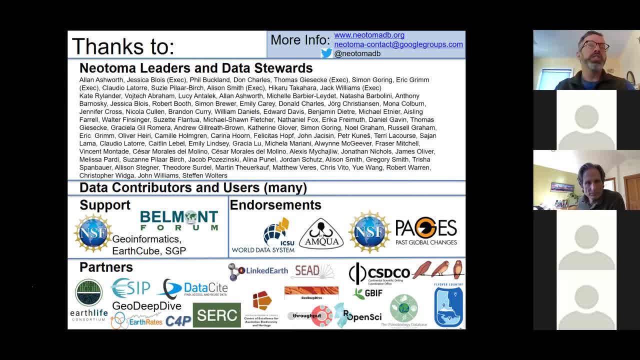 resource. i've also mentioned the paleobiology database, which is a deep time resource that is very similar. you know they have. you know people work with mollusks or deep sea ocean cores or other things, and they are also getting experts together bringing data in into the pbdb and then 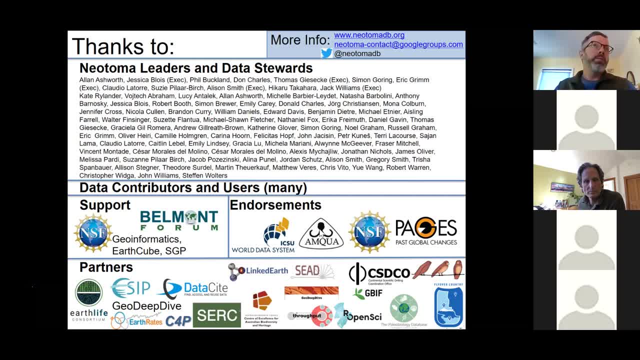 making that as a common data portal for their kind of data, but because the communities are different and they're they're storing and focusing on different things. so, carrie, you gave the example of you know we manage taxa names and you don't. that's an important difference and in in the deep time, they really they are also focusing. 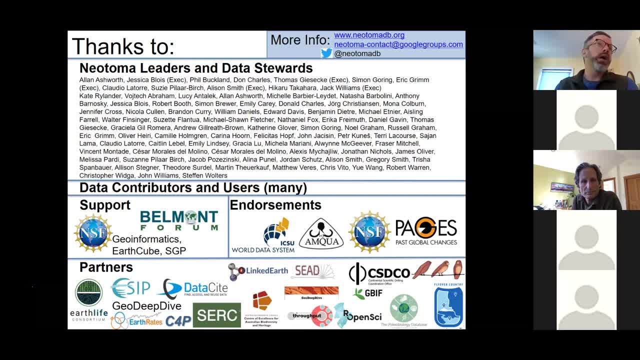 on taxa names a lot, but they don't care. they are less focused on, say, radiocarbon dates and getting radiocarbon dates are than we are. so the time scale leads to some different design decisions that we have focused on that they have not focused on, and vice versa. 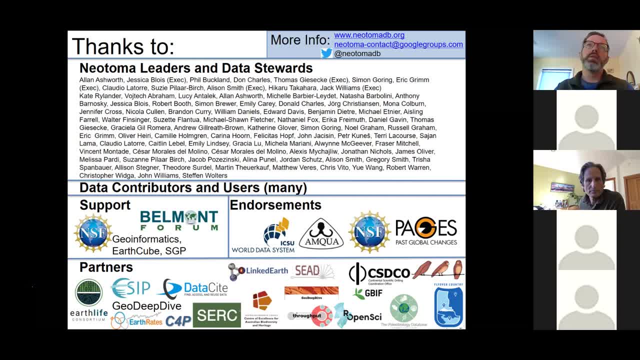 could you talk about a risk of going on? um, could you talk about, uh, the differences in the data models? like it sounds like the vtca has, maybe like pangea and its own database, but neotoma has is fundamentally comprised. it's like a database of databases. 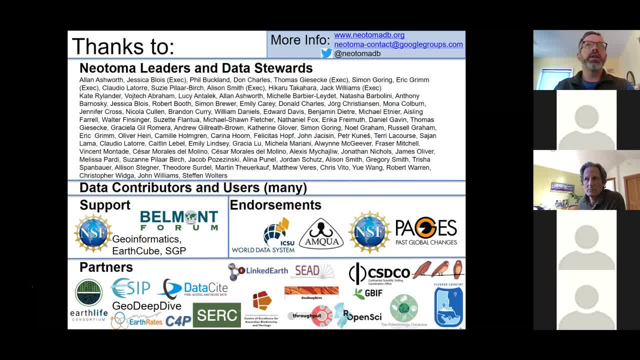 um, i'll talk about the neotoma side first and then carry maybe compare and contrast. um, the neotoma database is one relational database. it is one set of tables sitting on a server that has one set of relationships. so there's a sites table and a cheer chronology table and, uh, you know, a, a pi's name table. so we have a, we have a defined set. 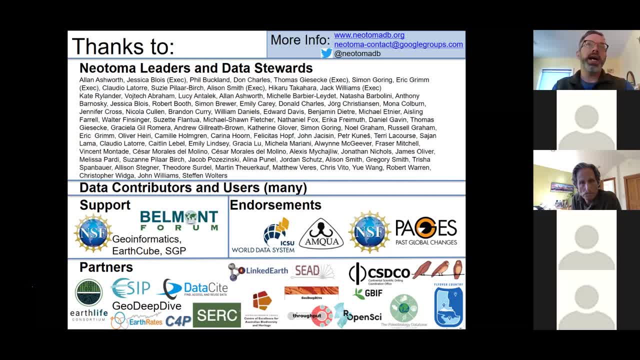 of tables and relationships among those tables. so if anybody uses work with access or, you know, sql server or postgres, these kind of relational database structures, we have one database that holds all this information. so that's the centralized side and that's one of the values that neotoma provides is providing one. 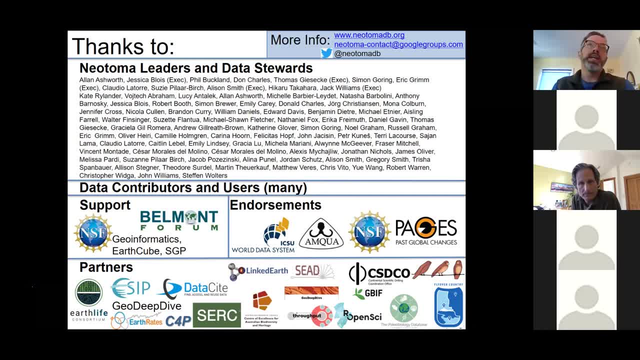 centralized database with one set of software based on that database that lots of communities can use potentially. but then we set up access rules that different data sets stored inside of neotoma are tagged to be owned by different constituent databases. so there are data sitting inside of neotoma. 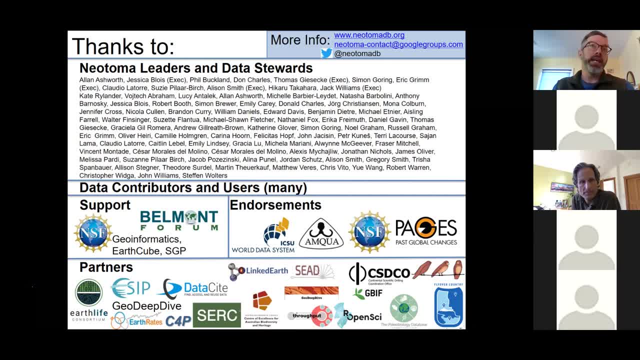 that are tagged as napd- north american pollen database data that i have access privileges to and can edit. there are other data sitting inside of neotoma that are tagged as epd- data that i do not have access privileges, so we have this sort of access control that allows. 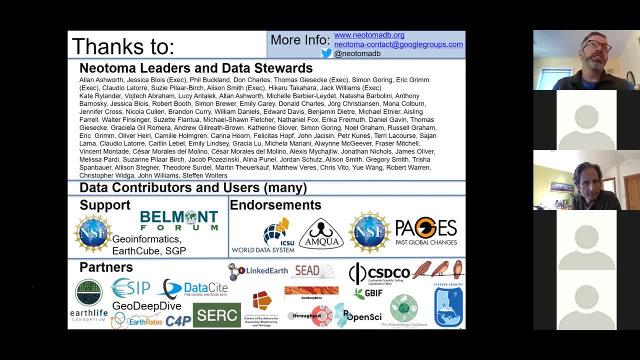 data stewards to to edit and manage subsets of the data inside of neotoma. and can i maybe just one more fallen add to that? i mean, i think that's an important difference between maybe just think about the evolution. so noaa and wdc formed in the 1990s, when the model 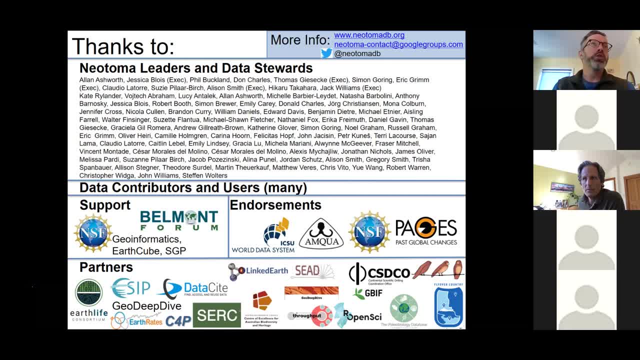 was kind of these centralized databases right, that all data goes into um one place and the people there manage that, and so i think i'll just i think a. a challenge then is how, how do you do that curation and stewardship, and who does the work? 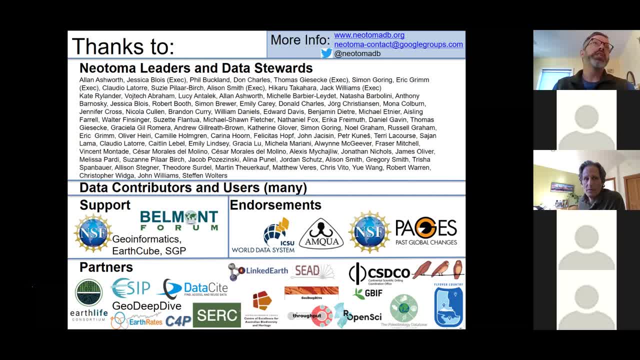 carrie, you might want to talk a little bit about who does the work when people contribute data to you. who cleans it? who makes sure it's kind of, you know, standardized and ready for general use. in our model it's kind of this distributed model of different data stewards among different 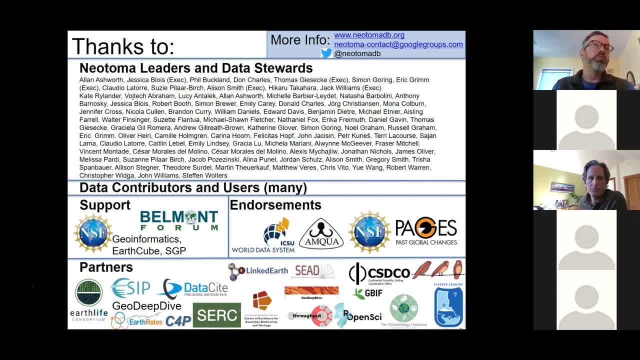 constituent databases that can be in a sort of franchise model. you could have more people doing that effort for different systems. so that's one of the things that we're trying to do with neotoma, um. so i think it's important to make sure that we're not just on the fringe of the data. 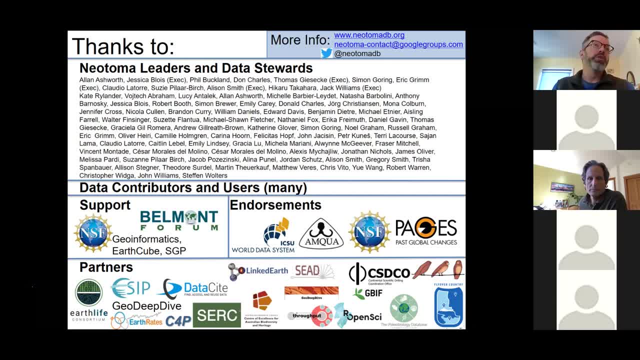 got to be a little more of a centralized model in terms of the data that we're collecting, that we're not just sort of working on a particular subset of the data. but my sense is that noaa has a little bit more of a centralized model in terms of a staff at 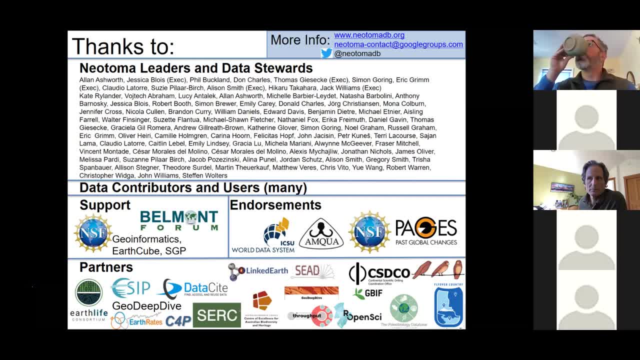 your at your institute that does most that work or works with individual scientists to get things ready? yeah, that's correct. i think that's a good um description of a very centralized model. i see that bruce is unmuted. is bruce there? bruce would have more insights on this than i do. 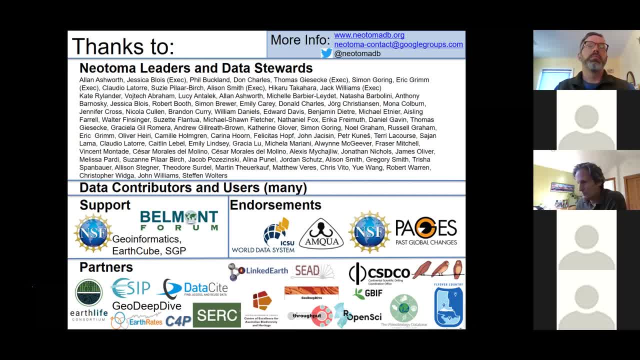 Right. We have data contributors who send us data and there's some back and forth between our data managers and the contributors to try to get it right, get the metadata correct, do a little bit of quality assurance, especially for tree ring contributions. There's a big workflow there in terms of doing some quality assurance And then the metadata goes into our database. The data does not. So that kind of goes back to what Jack was talking about with the flat files of accessing the data. 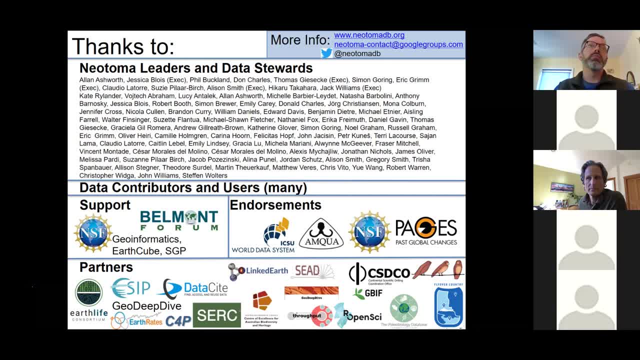 It's in flat files And we also have interaction with data synthesizers, So we provide data out to people and then we get data back As people synthesize it into larger compilations, like, for example, the temperature 12K project, And so that's another method by which there is some quality assurance, that happens and additional information is added through time in that way. 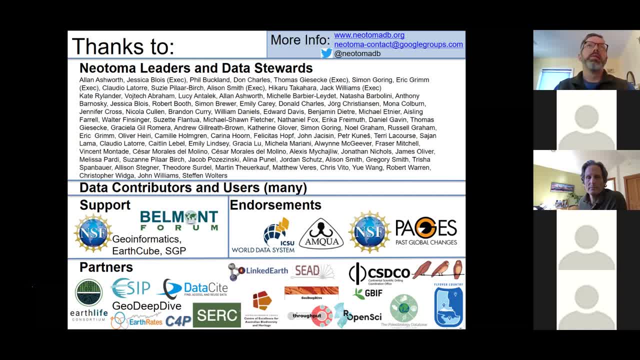 But yes, it's a much more centralized model. There's not a lot of data stewards who have access to our underlying database. Another point I'll add too. I think there's an underlying question of should there be one database or many databases, right? 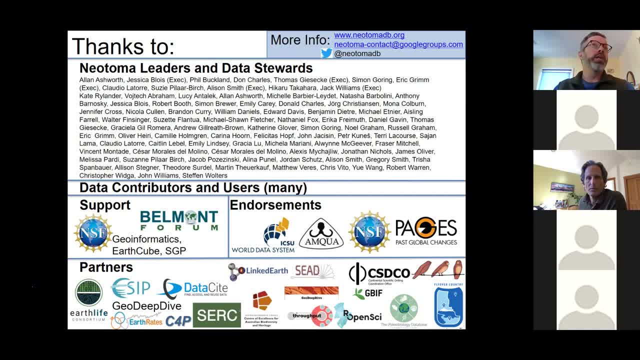 You know, are NOAA, WDC and NIATOMA redundant with each other? Or, if they're not redundant, what are the advantages and distinctions between them? And I really see that what we are. I see there's some process of consolidation in which, you know, FONMAP does not need to be a standalone database anymore. It's part of NIATOMA as a constituent database. So we have one model of aggregation in which data comes into NIATOMA, gets added to it as part of the database and then it gets added to the database as part of the database. 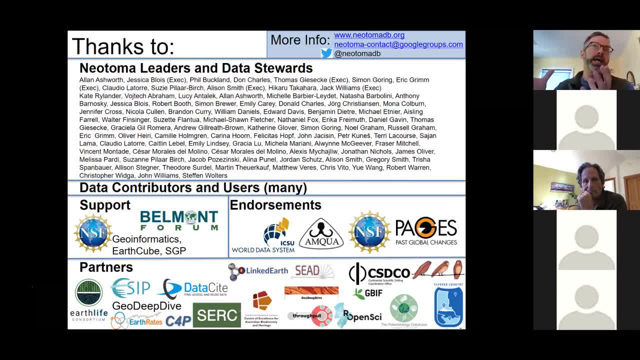 So we have one model of aggregation in which data comes into NIATOMA, gets added to it as part of the database and then it gets added to it as part of the database. So we have one model of aggregation in which data comes into NIATOMA, gets added to it as part of the database and then it gets added to it as part of the database. 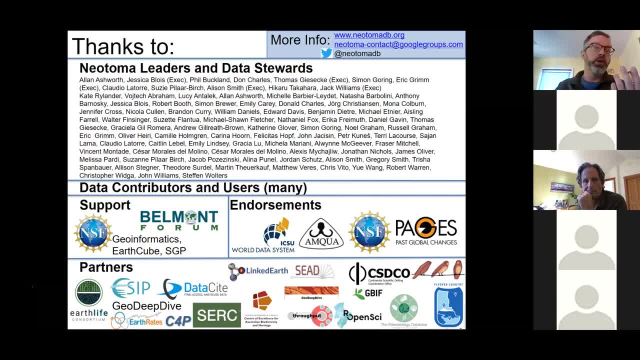 And there are things we'll never try to curate and you know, and we'll always have these sort of finite subdomains of what's out there. So I do see this emerging ecosystem of different data resources, curating different kinds of domain and knowledge. 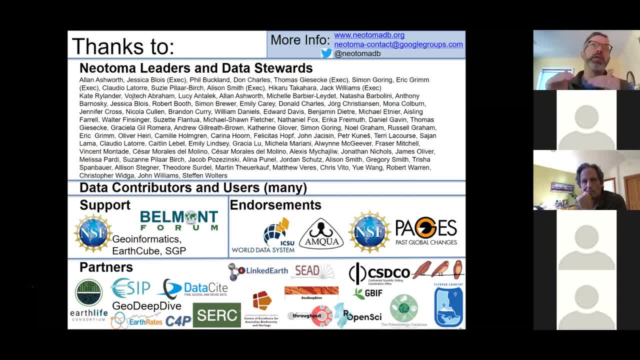 And there's always going to be some gray areas of potential overlap between different data resources and what they do. So I think it's helpful to start to understand that they all have slightly different models of how they do this. they all have slightly different models of what they're storing, but they're not 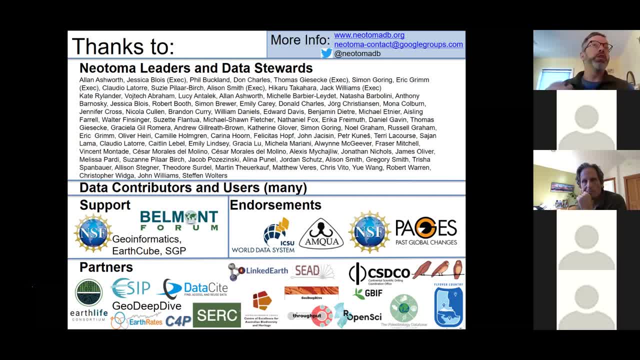 I am looking at it. you know you can do a pangea. you know pangea tries to be sort of a database of everything, and that's great. pangea is good for that. but what it means the trade-off then is that you have less. 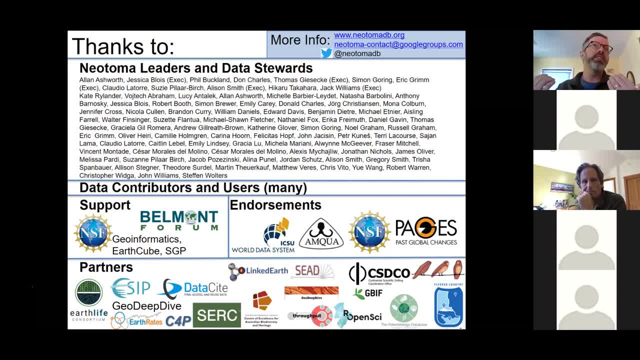 customization. so they have some general service they provide for all kinds of data. the less customized services for, say, tax on name management, which is something that's really important for us, so you know there can be different spectrums for more general purpose, generic databases with sort. 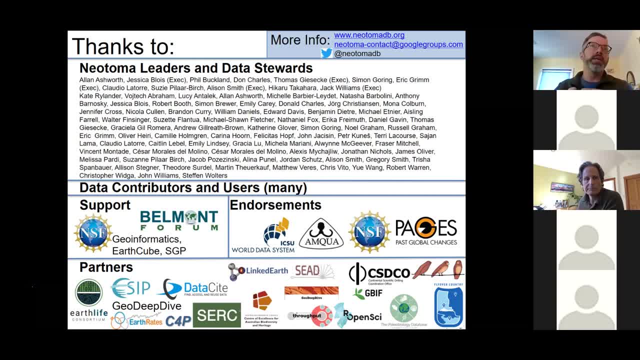 of generic services versus more customized community specific databases that meet community specific needs. great, we um sort of along this line. there there's a question from pierre francis who's asking about whether there's an option to have uh sort of the neotoma data container. 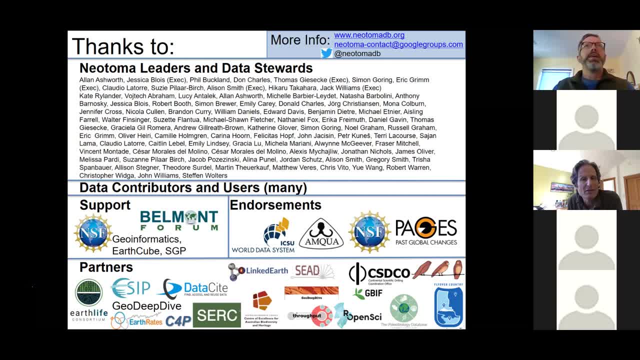 available sort of on a lab level, um sort of along those lines. i mean, is there a way that we can um sort of facilitate the um, the the transfer of data from individual labs to the data container? um, so that we can sort of facilitate the um the the transfer of data from individual labs? 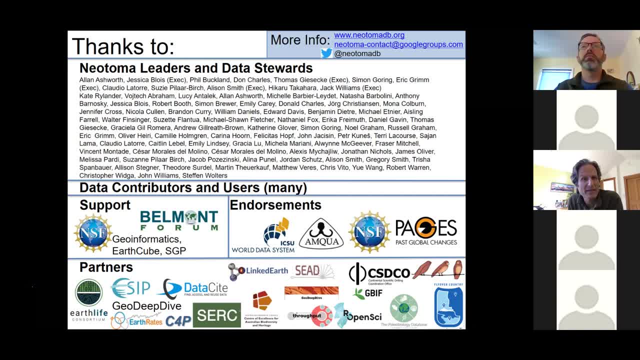 to sort of um foresee what the structure and the metadata that are needed in order to enter data into neotoma? yeah, yeah, great question. um, yeah, so, um, a couple different things there. um just to, uh, you know, deal with kind of data versioning and just make sure we have kind of one. 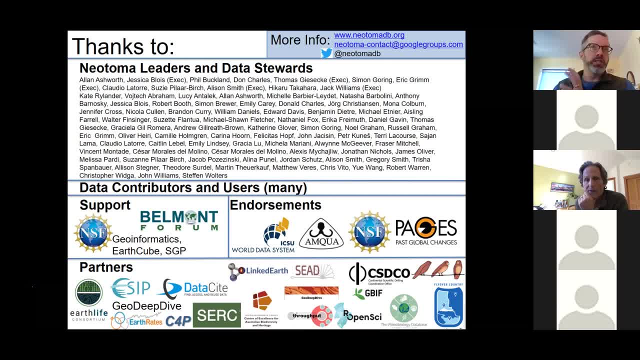 master version that neotoma database is on a central is centralized on a single, on a server with, you know, backups and and you know backup redundancy and stuff. but we just we don't yet have a um well, so a couple things. um, uh, we do support database snapshots, like every. 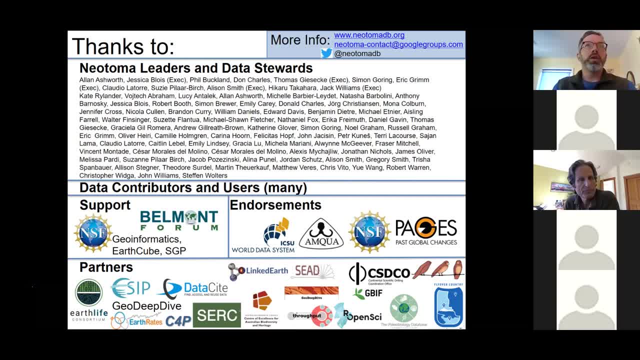 now and then we'll just do a database dump. so if you just wanted to get the full contents of the database and and have it locally, you could. you could get that, and we periodically post snapshots um up to be available, um, so it's not quite an automatic do it every three months, kind of thing. 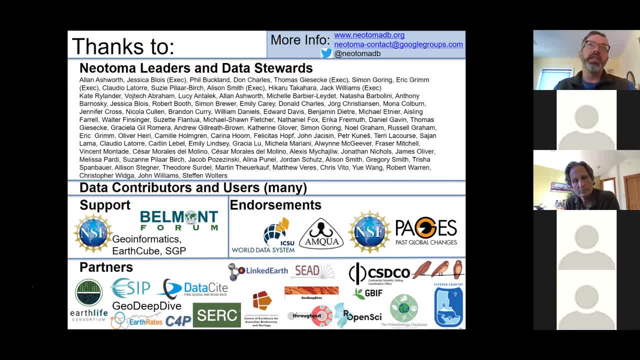 but it's on a on-demand basis. so if you wanted a full copy of the neotoma database to look at and look at its data structures, we could make that available to you. um, we you know, working you know. again, it's kind of like figuring out what people's needs are. um, when we worked with alpadaba, for example, this alpine- 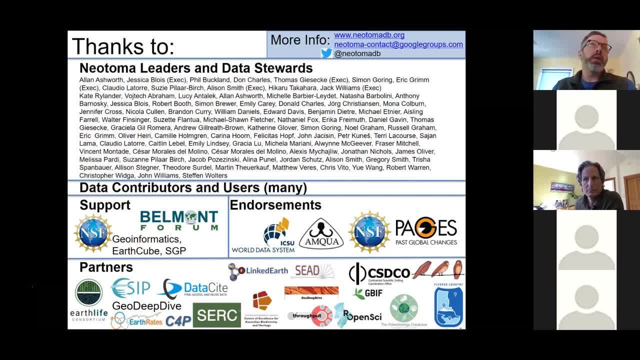 pollen database. it turned out that they really did want to have their own copy of their data, you know they. so they basically put into neotoma, but they want us to kind of then dump back out a postgres copy for them of their data. um, because they needed to be able to show their, you know the. 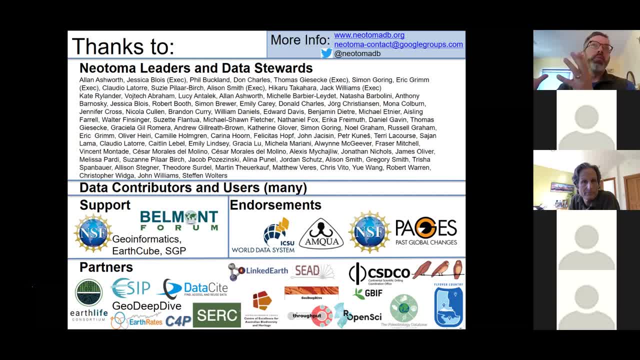 swiss national science foundation that they had a data product that they could point to, and so we can then do that. so if you're a constituent database and you want to have your own copy of the data, we can kind of do that service on kind of an on-demand basis, um, and then you know learning. 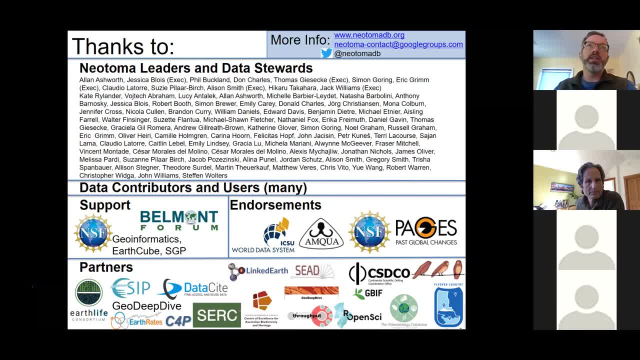 more about how to do this. you know tilia, for example, that that tilia point of interface of uploading data to neotoma. you can have your own copy of tilia, you can have some example data files. so if you want to kind of get involved in that process of, you know, getting data ready for upload, 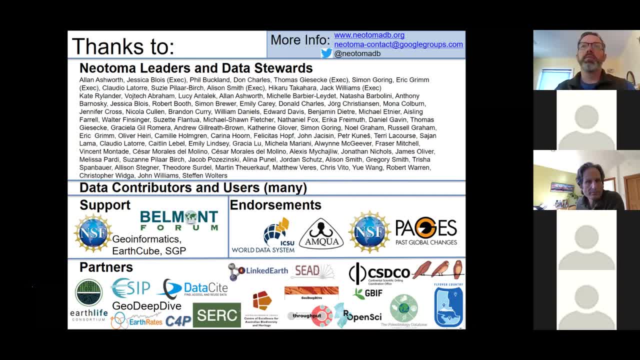 we can certainly give you model data and software to work with that and feel free to follow up on that question up here if you want to more specifics on that point. um, do you hear me? yes, uh, yes, well, actually i don't, i don't need to have the whole data set. 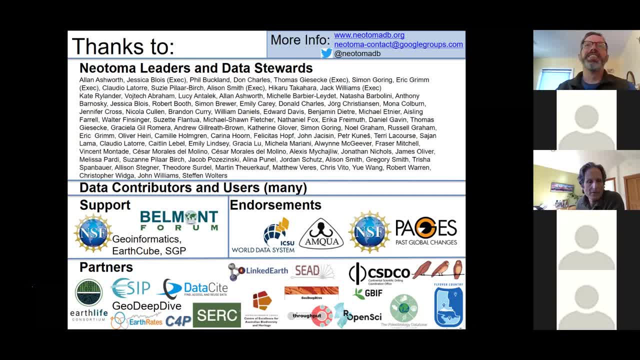 i guess i can access that on the website. uh, it was just more the the structure of the database. so i'm thinking of the students. when they arrive in a lab they don't know what to do with a sediment core, what do, what information they have to to record, and so on and so on. so having a database to 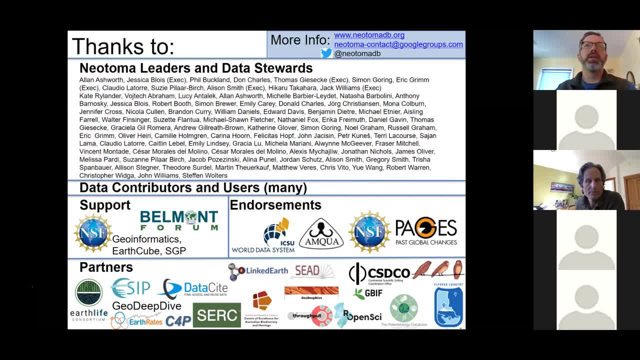 actually to collect the data every day, um, but sometimes to provide information in auting the lab? um, what can we do with that data? um, but sometimes it's so it's like nobody knows. uh, sometimes it's the people who aren't learning, so sometimes they don't know what to do, um. 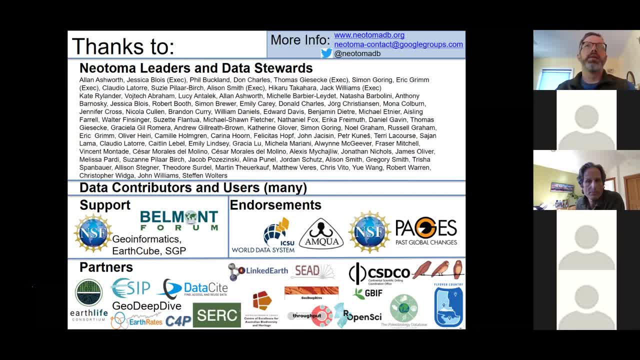 um. so i'm thinking um was, uh, most of the things that we do all the time as Teachers, how they take their time to understand, how to integrate Japan and filtered elements different in order to better share them with the community. It's a great question. 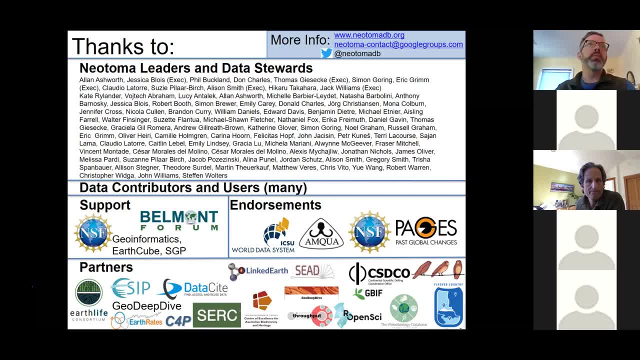 We don't really have a lab information management system. that would be a nice thing to have. It's still a bit of people doing it on our own. In my lab we would still count and have data in Excel files and we would copy over import to Tilia. 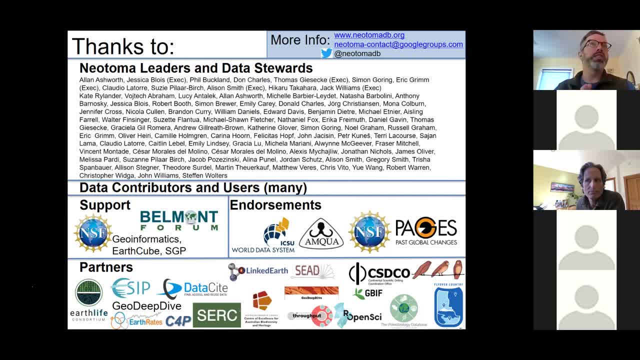 Tilia's kind of made upload interface and then we'd bring it to the Atoma. So it's cumbersome and it's not the best system. We have some colleagues in Australia who have developed a tablet-based pollen counter, And so I think one of the really exciting ideas. 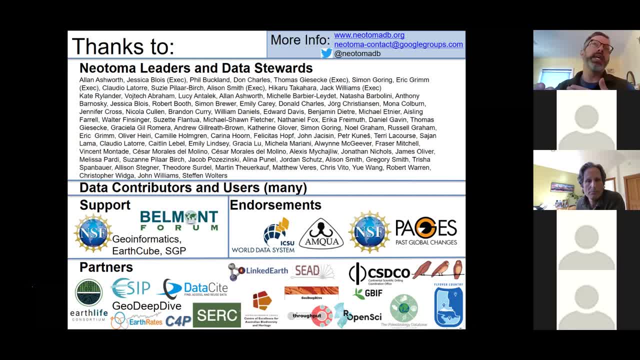 is to have like a tablet-based pollen counter that then generates the data in a ready to import data format. We haven't built that yet, but that is a idea that's just waiting for somebody to do it kind of thing. So that would be a step in the direction. 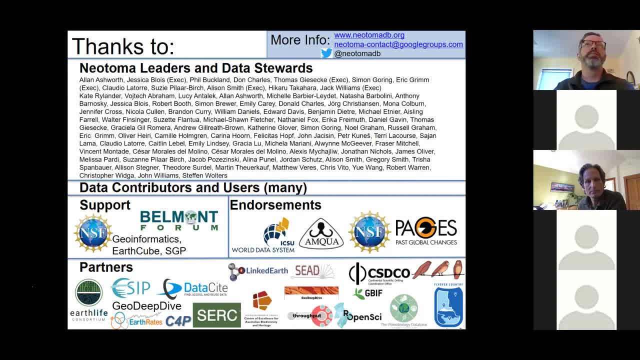 that I think you're asking about Other questions. Well, I'd like to ask one. I understand that the foundation of the Neatoma database are the constituent databases And I'm wondering sort of what constitutes a constituent database. So I can imagine a pages working group, for example. 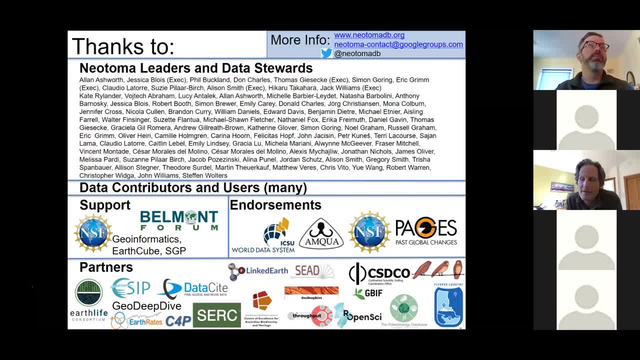 that develops a data synthesis sort of product. Let's say sea ice in Antarctica and we've got a couple dozen cores with various indicators of sea ice extent back in time. Does that constitute a constituent database or does that kind of get parsed into the different proxy types? 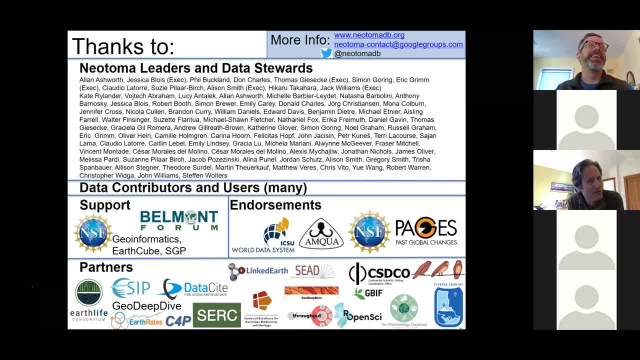 and then we confer with those proxy experts, or how would that work? Yeah, it's a great question, And actually one of things I personally like about the constituent database is that it's a very flexible concept, Because these things can happen in so many different ways. 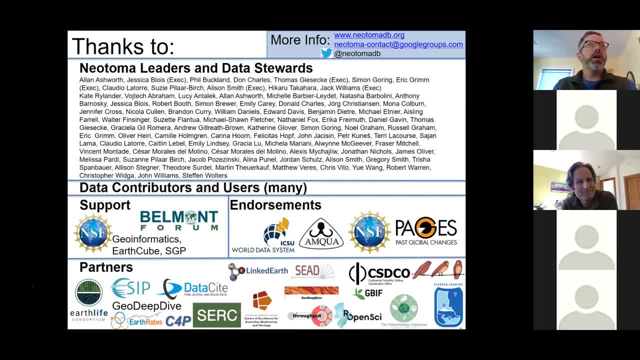 It's hard to be overly prescriptive about it. It's hard to be overly prescriptive about it. I would say the most common way that a concision database is defined is by a proxy type and by a geographic region. So the North American pollen database. 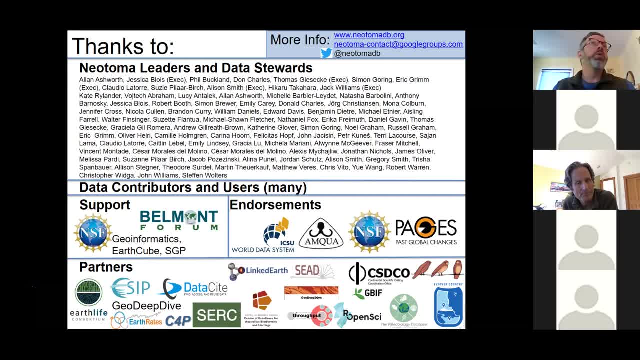 the international Ostracon database. So you know anywhere, but you know it's still kind of that. those are two different examples of different geographic domains, but by one proxy type. There I'm trying to think of I don't have. 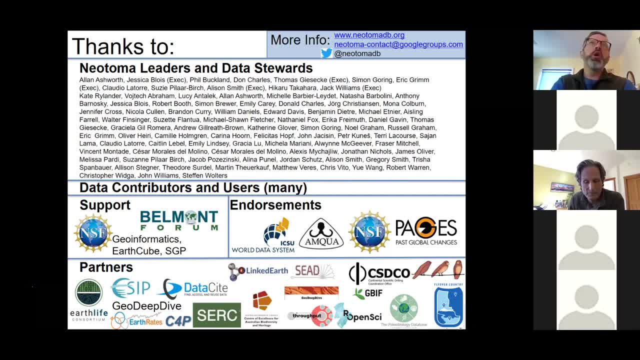 I feel like there was an example of a, and usually we go by proxy type because that's where the expertise is right. People are diatom specialists or pollen specialists, And so you kind of want to map the concision database onto where the expertise is. 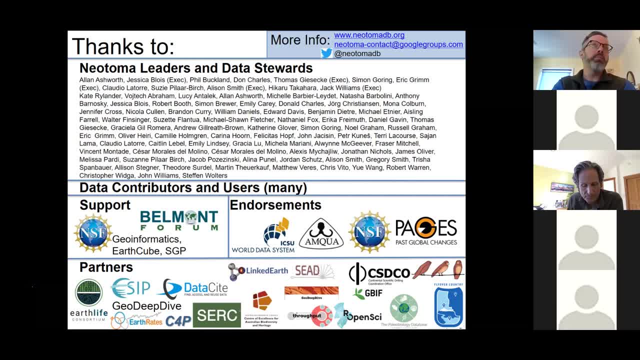 And so a multi-proxy concision database would usually not be a great idea. But sometimes, like you said, you might have someone say: we're going to work up in the Arctic and we're going to get every paleo record we can get from the Arctic and build a database of that. 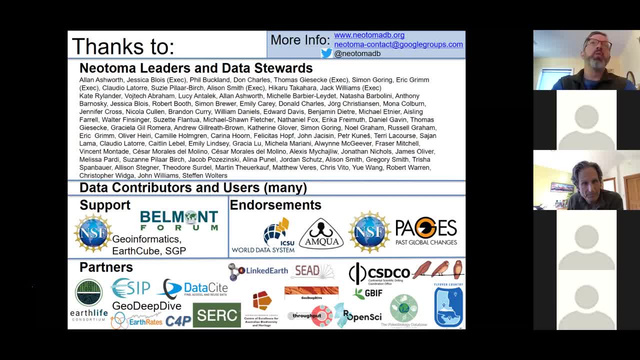 And you do want to enable, then you want to have a postdoc, say, work in the project, be able to upload a bunch of pollen data and charcoal data. Right now we only allow one data set to be owned by one constituent database. 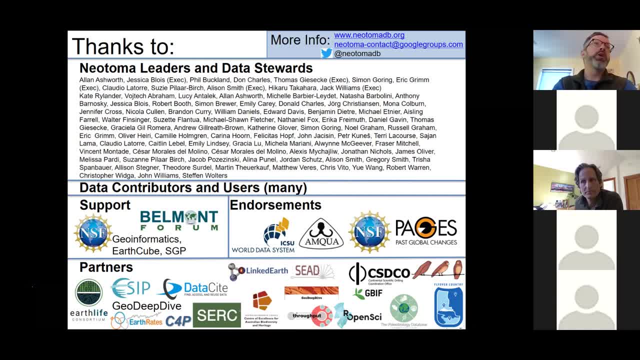 We could relax that rule in the future to say, okay, that record just got added and it's both in the North American pollen database and it's in the high Arctic synthesis database And there's two owners of that. That could be something we could adapt to in the future. 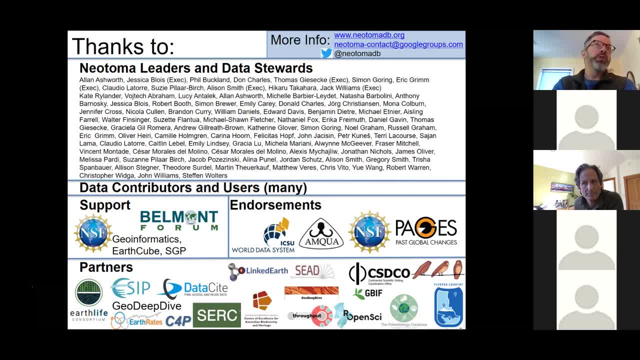 So it's kind of on a case by case basis, And we would typically ask like what's? does somebody already curate this data? If so, can we just add to that existing database? If this is new, where's the gap? 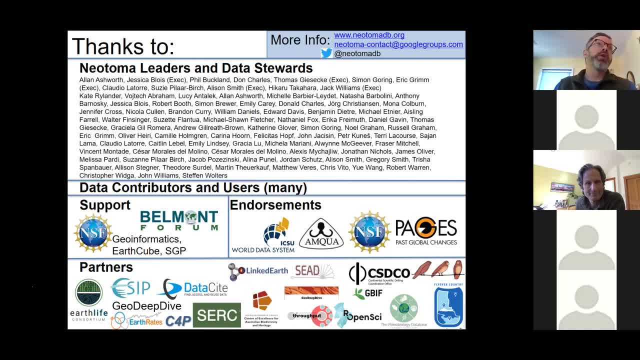 And I would probably also ask: how long will this project last, right? Because if it's kind of a typical research project where it's kind of three and done, then I might say, well, we would like to see some kind of commitment to curating this data. 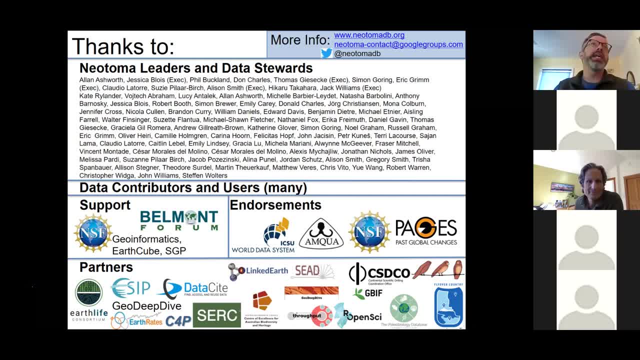 Think about that question beyond that three year time horizon. So there's a little bit of a sustained commitment question. Do you know It could be a lab basis? You know there's some labs that have just generated a ton of data. 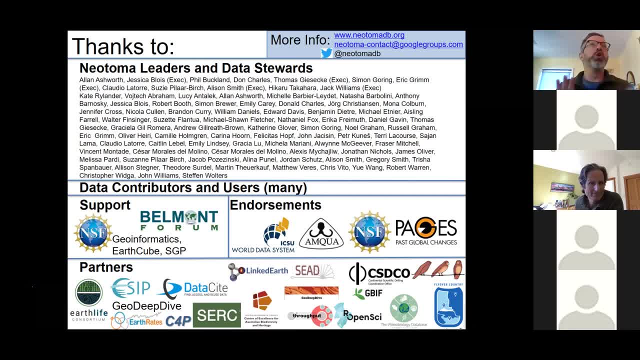 You could argue they should have their own constituent database. So we don't have hard rules, We just have kind of typical examples. That makes good sense. Yeah, yeah, yeah, Hard to one size fits all for sure. Yeah. 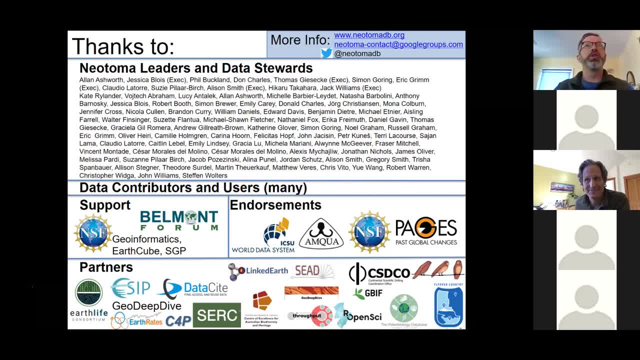 Yeah, Mike, we try to avoid redundant entries, We try to not have that, And so we try to keep an eye on that, And so that could be a risk associated with sort of constituent database proliferation. but we have some tools. 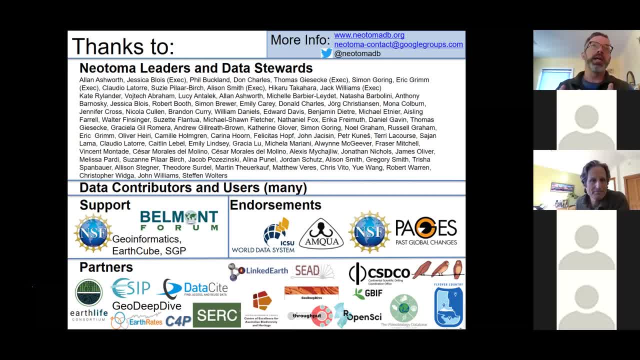 Part of the QAQC during TILIA upload, one of the some nice little tools that Eric has built. So when you're uploading data from TILIA into NIATOMA it'll do some duplicate checks. Is there any other site with a similar name? 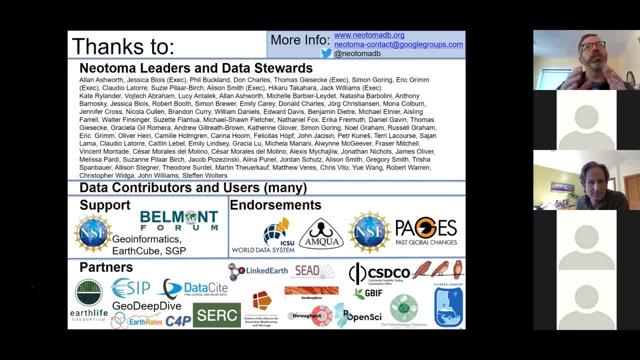 Is there any other site? How many other sites are there within 10 kilometers? So it does some by area, by name checks, And so it starts to say: hey, wait a minute, you just uploaded a dataset from this site. 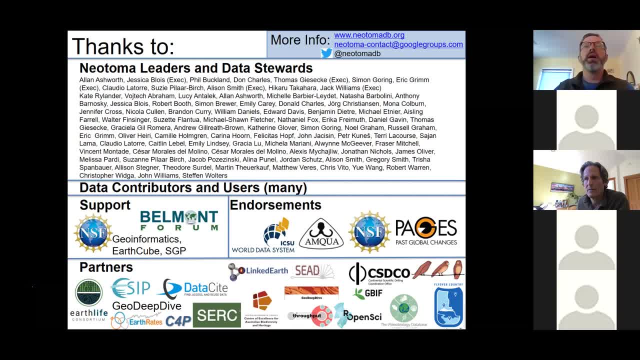 and there's already five datasets from this site, So it'll do some checking there. Mike, you asked another question in the chat window a few minutes ago. That's also important about versioning And we actually an important thing that we traditionally have differed pretty fundamentally. 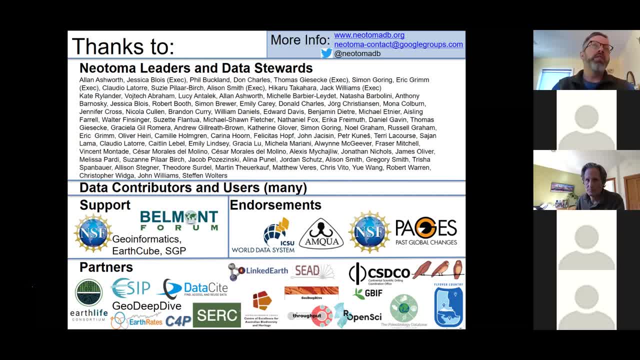 from other archival data resources is that NIATOMA has kind of viewed its primary mission as supporting living data, That our top mission is to provide kind of latest and greatest data that has the updated age models and updated taxonomies and so forth. So that's been our top priority. 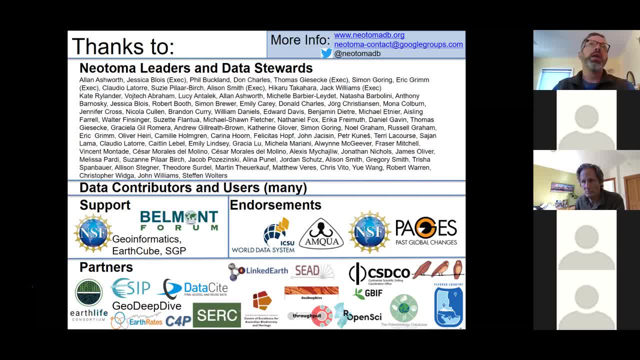 but that creates that issue of versioning and reproducibility and archival And journals. specifically, we really want the data at the time of submission recorded. So now our new system is to basically support two versions of the data: the time of submission version. 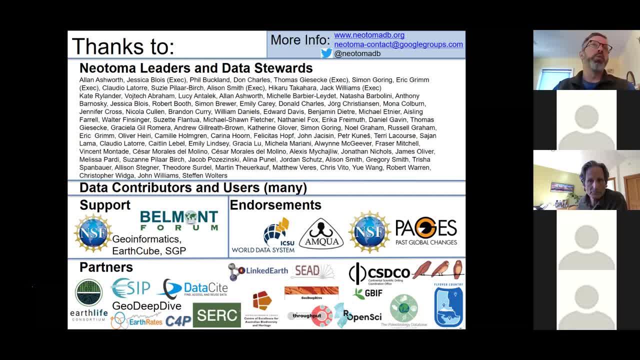 which will support journal needs, and then the living version, which will support most practicing researcher needs. But we don't version at this point in between those two Excellent Other questions. Well, okay then. So we will post this video recording on Paige's YouTube channel, I believe. 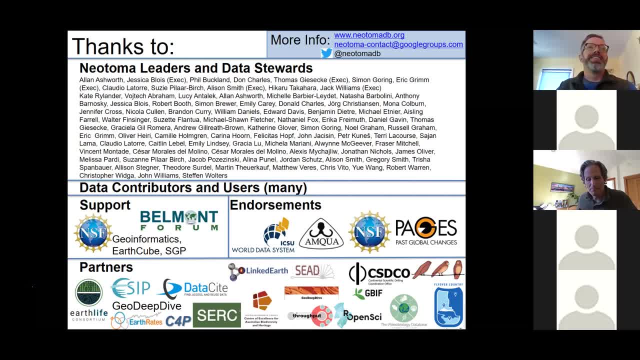 So if you have colleagues or others who would think would benefit from listening in, that will be available next week. So thank you, Jack, very much for the very informative presentation And thank you, Sarah, and thank you to all of our panelists. 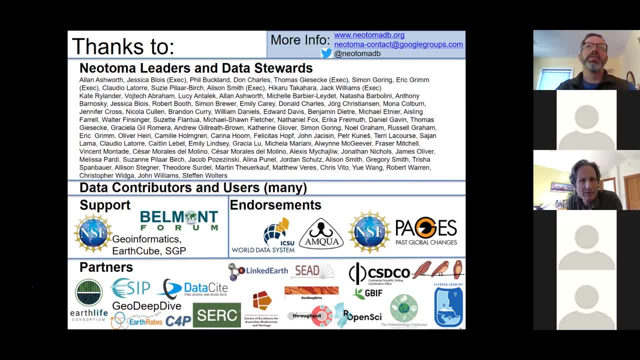